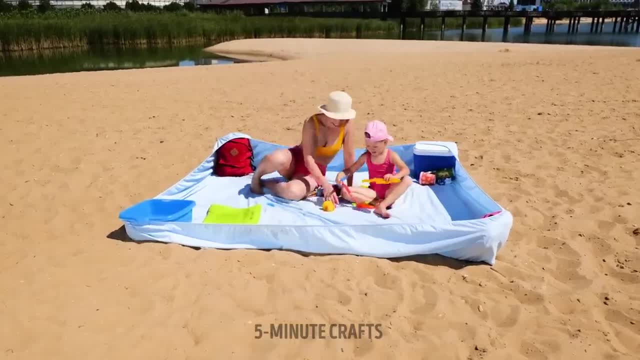 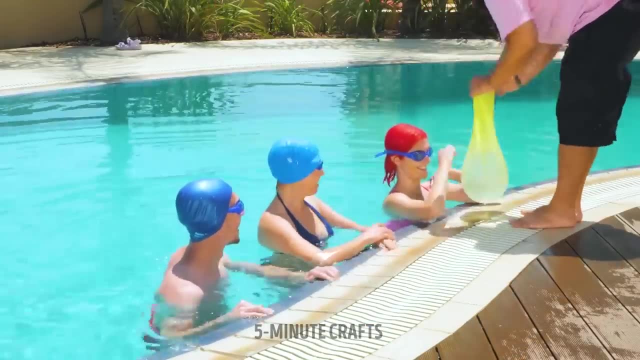 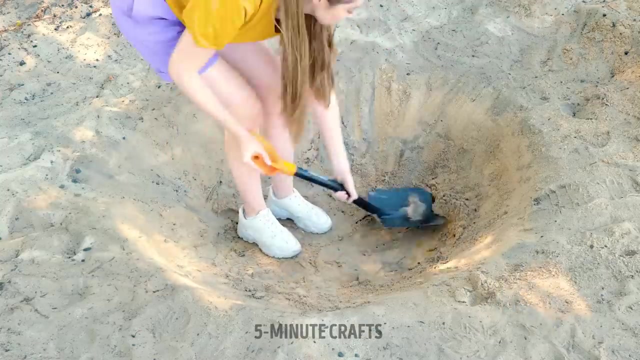 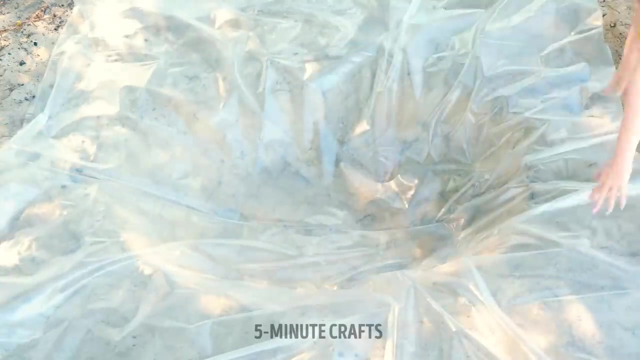 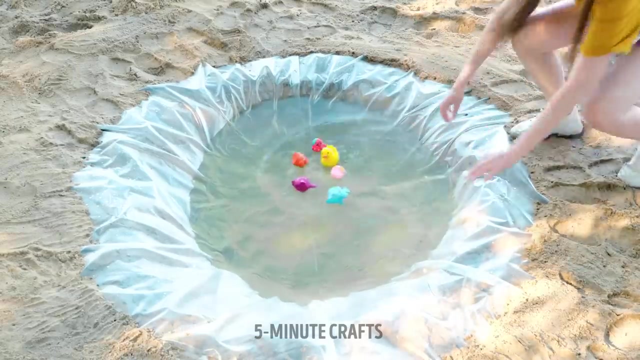 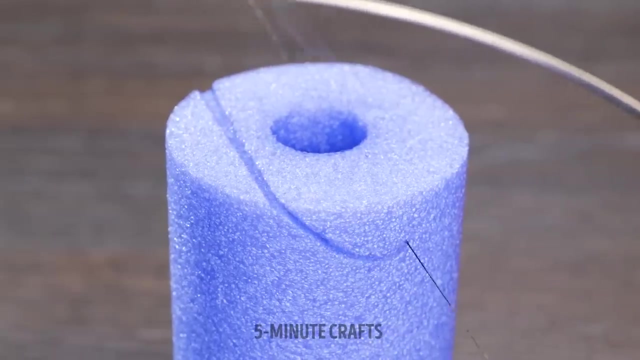 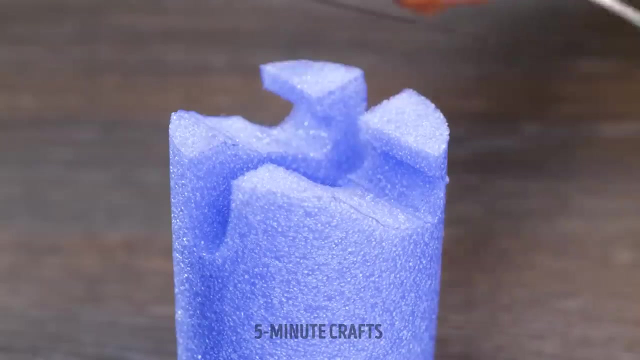 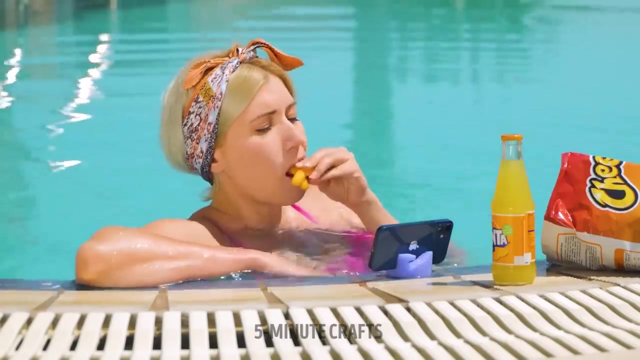 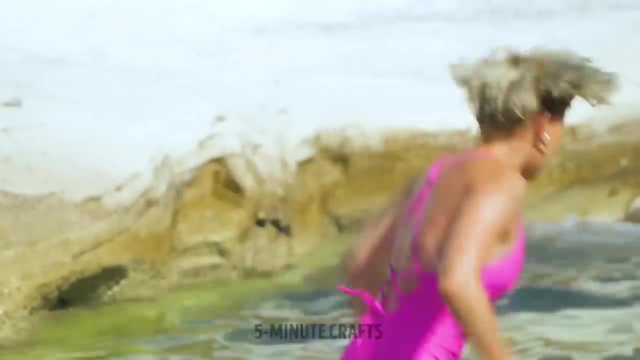 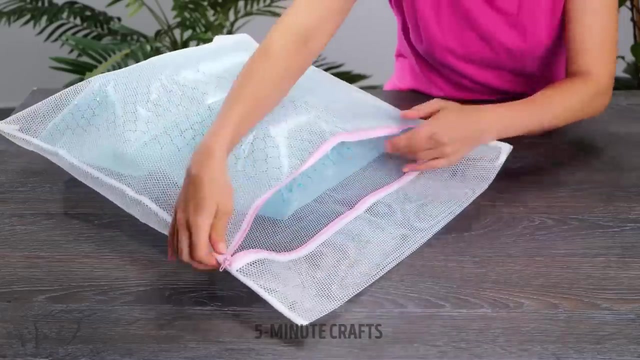 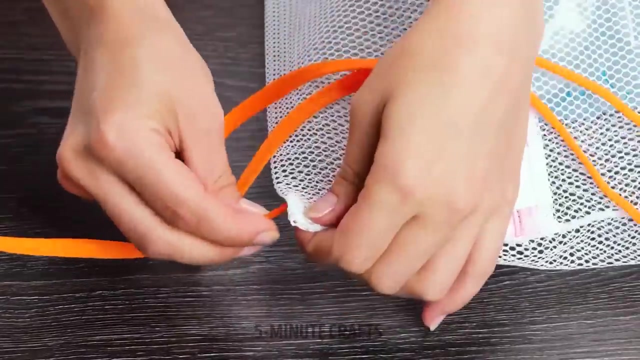 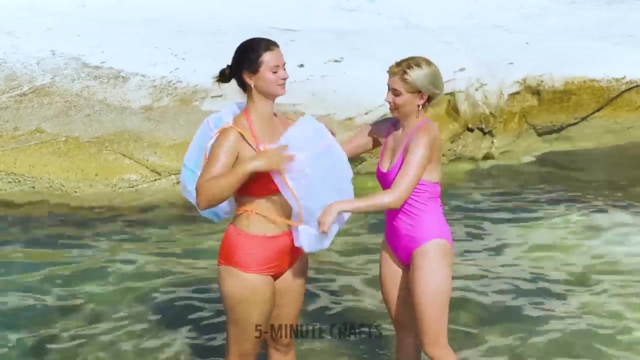 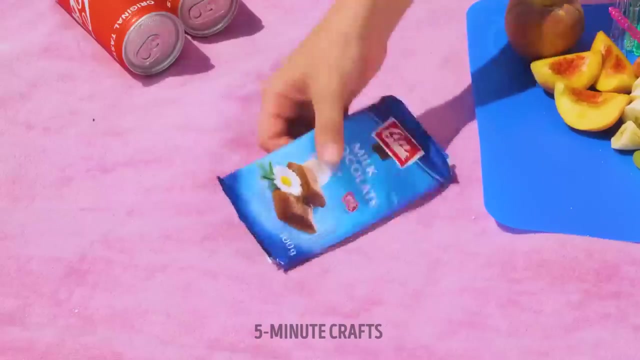 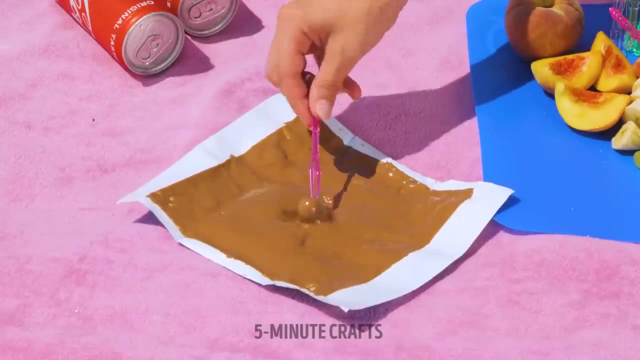 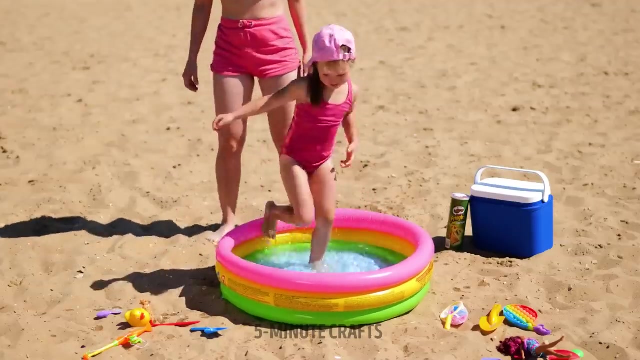 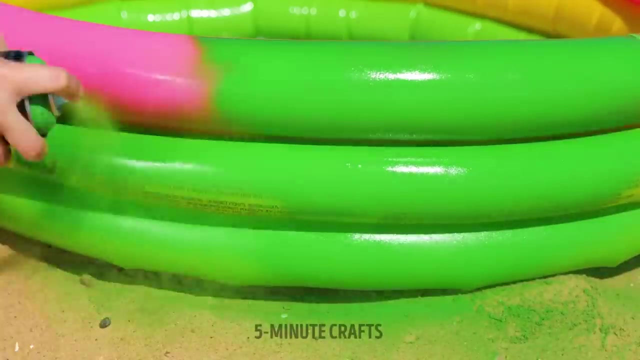 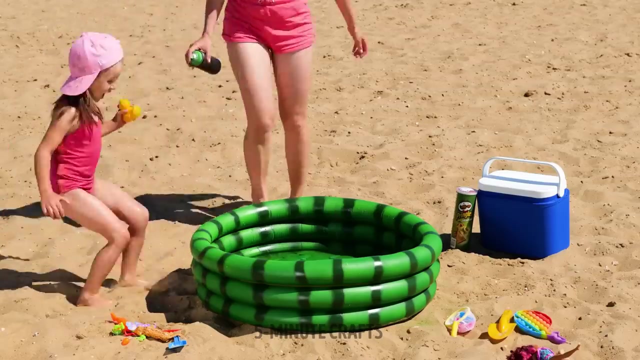 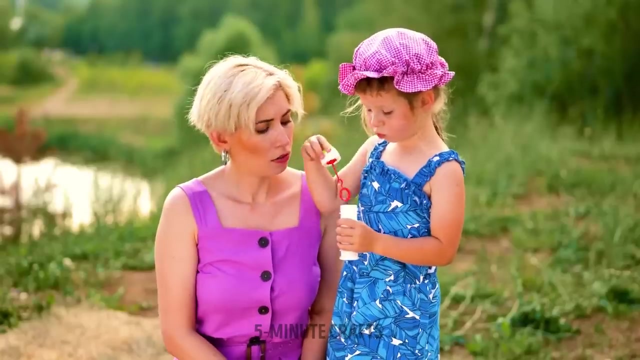 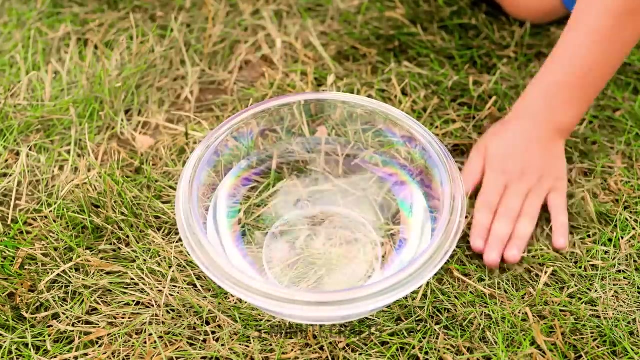 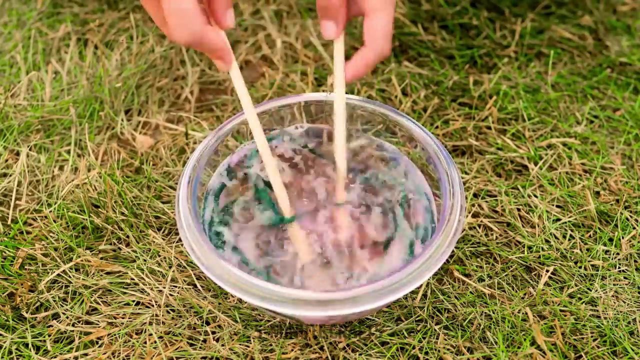 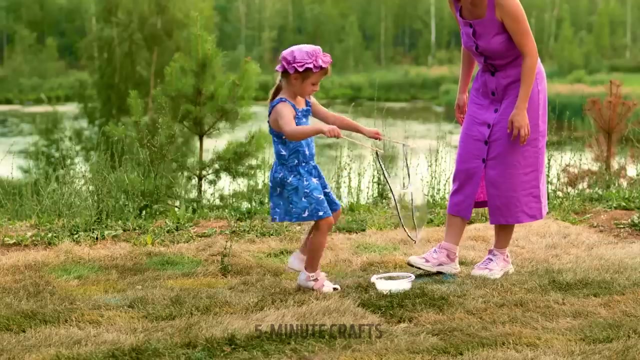 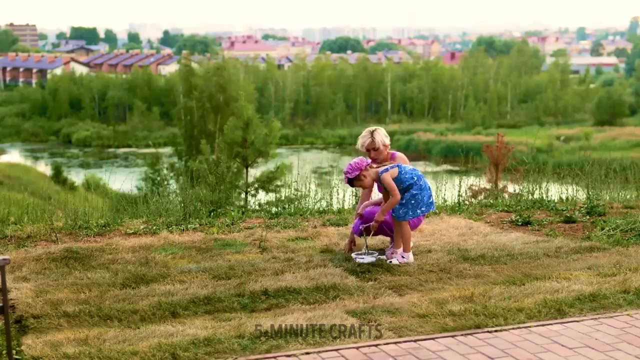 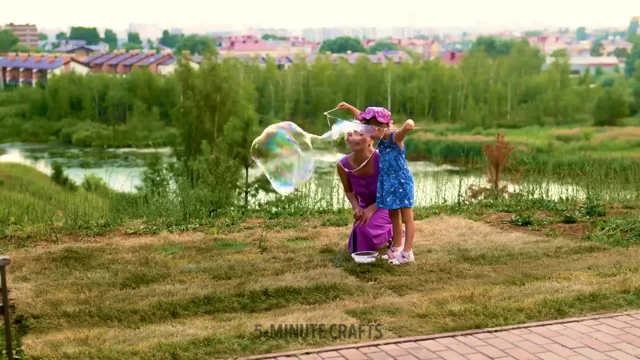 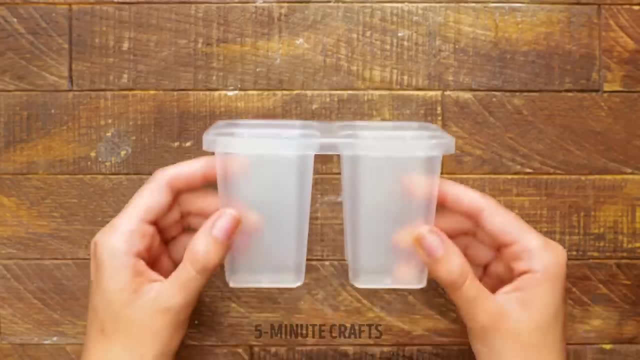 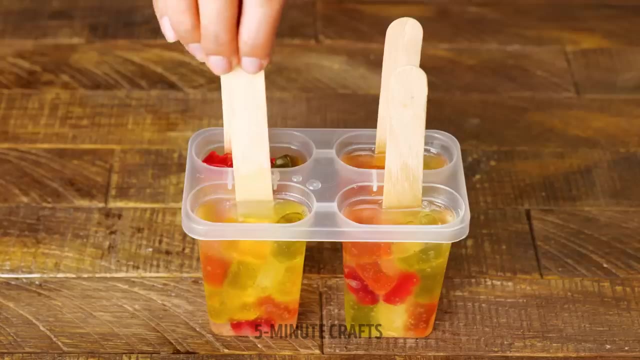 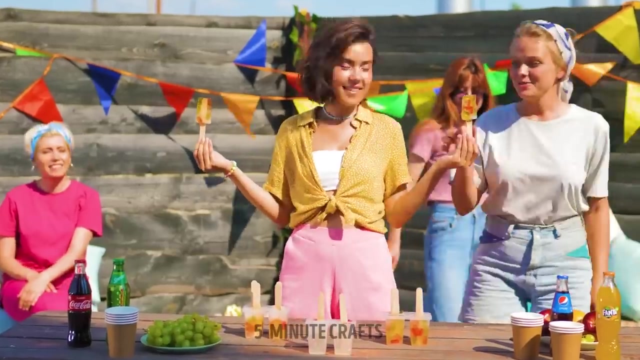 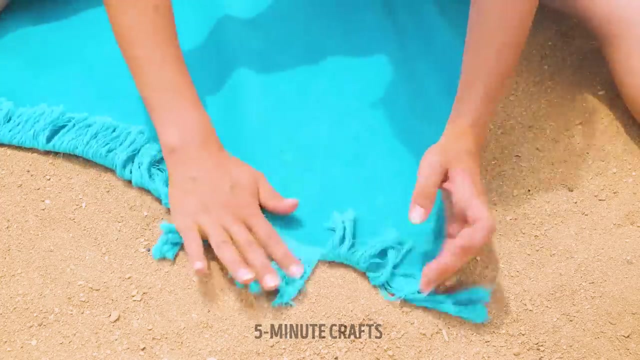 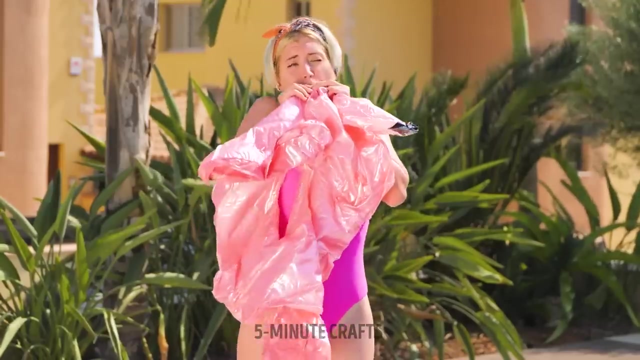 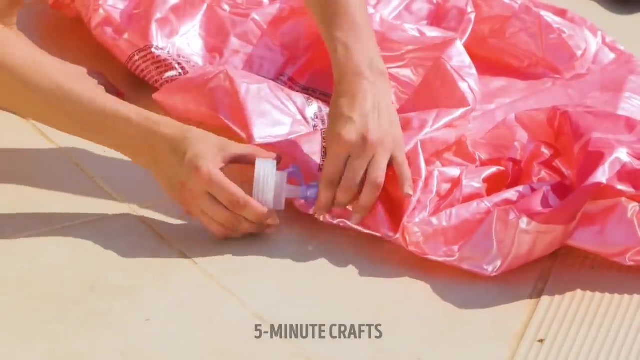 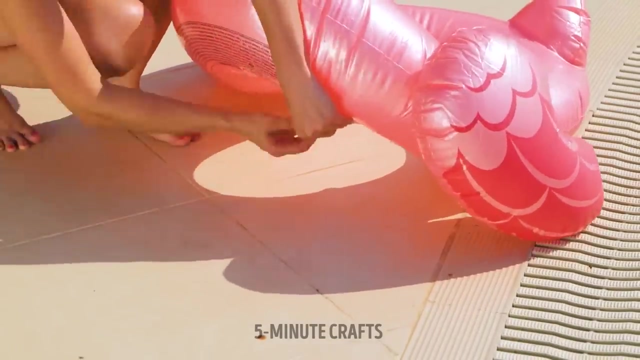 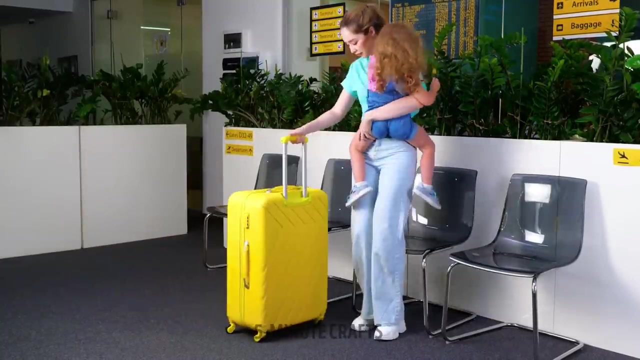 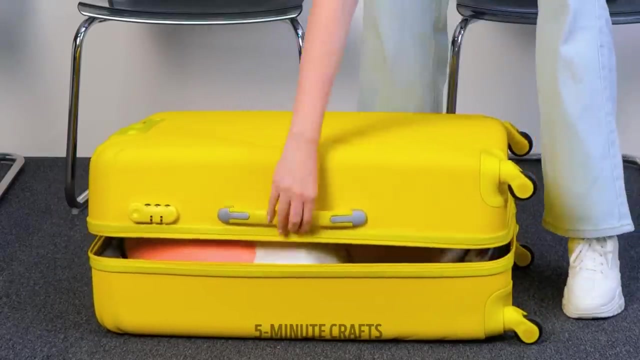 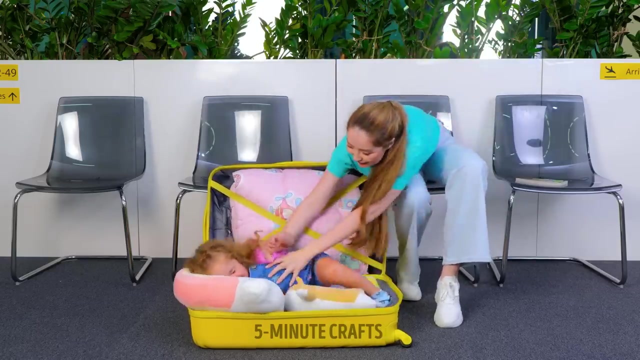 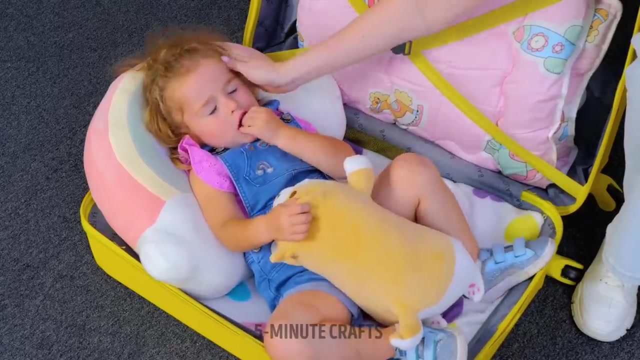 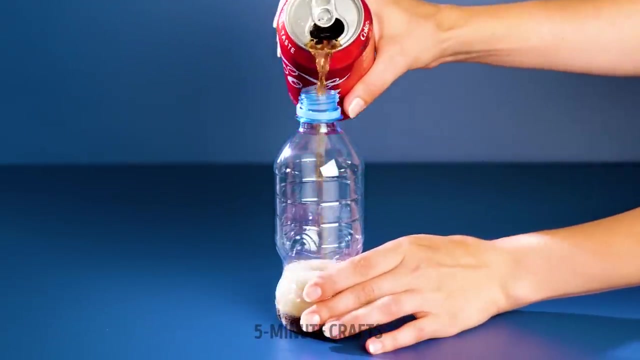 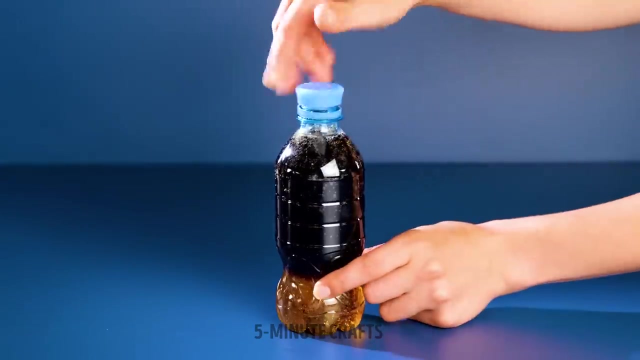 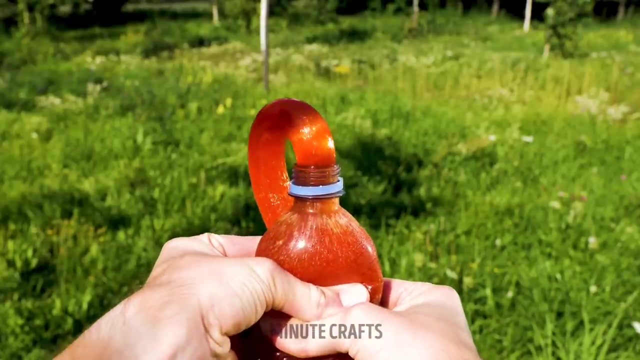 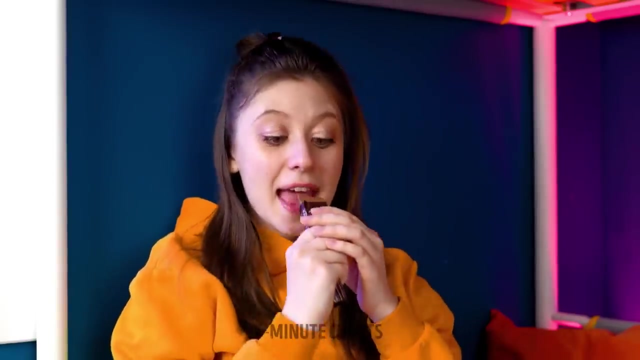 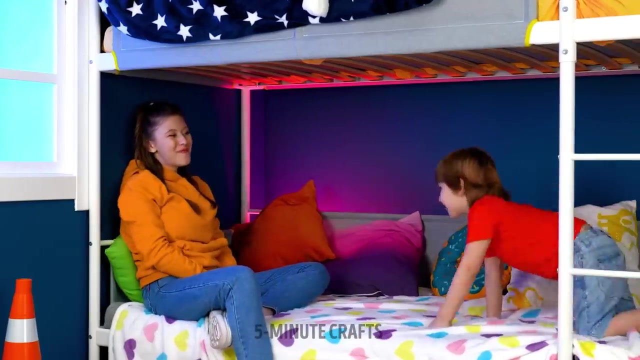 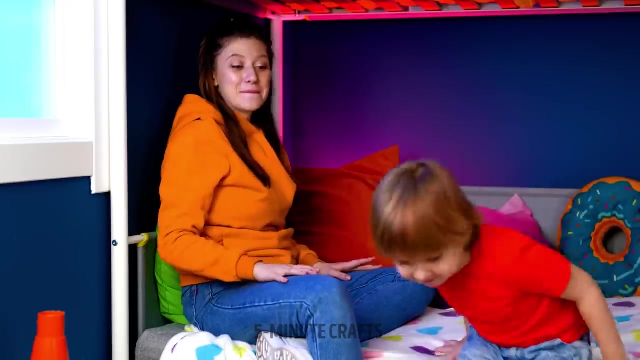 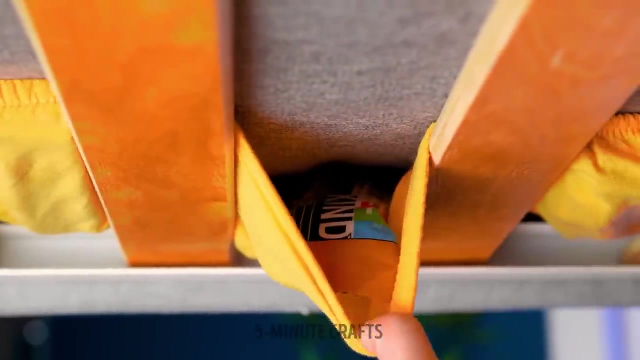 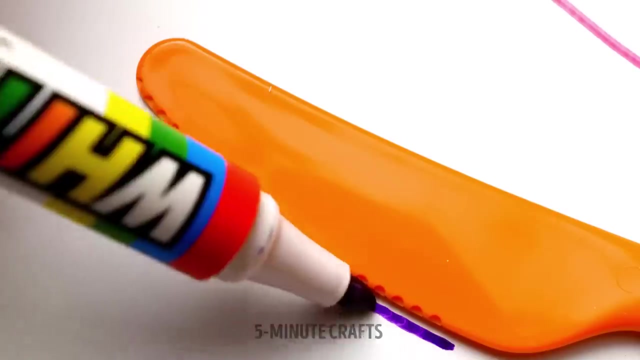 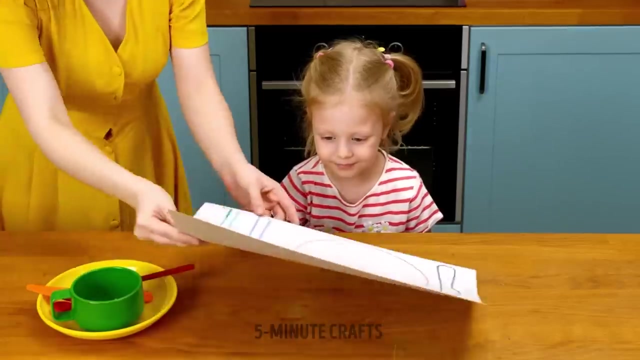 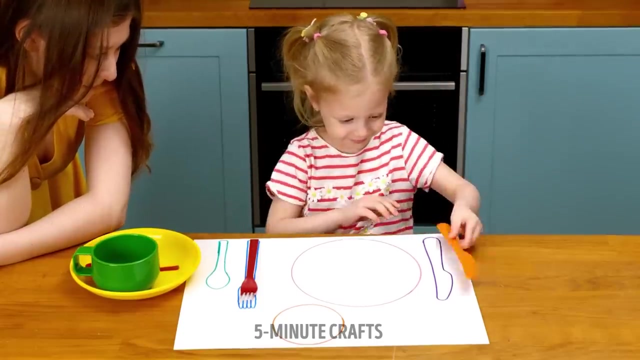 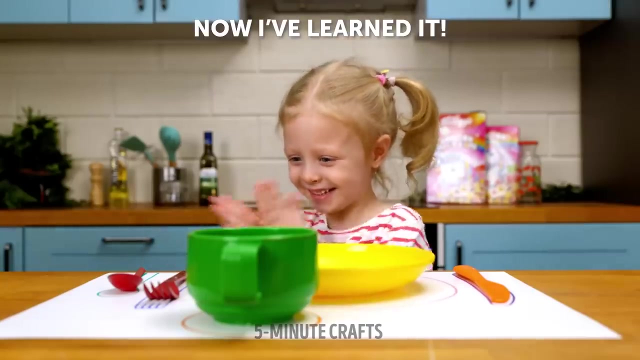 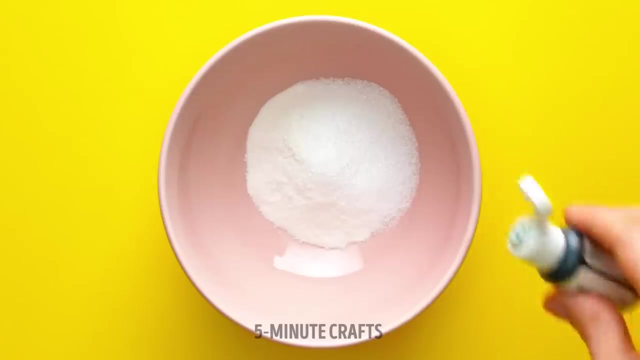 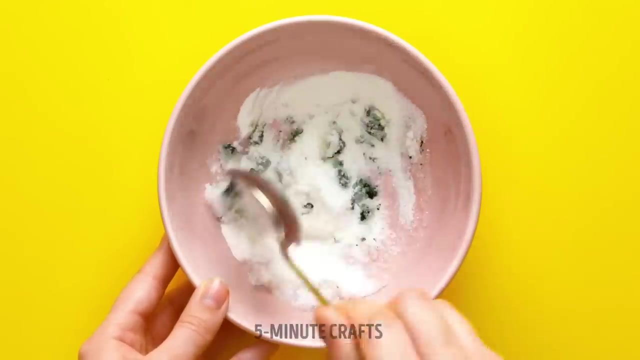 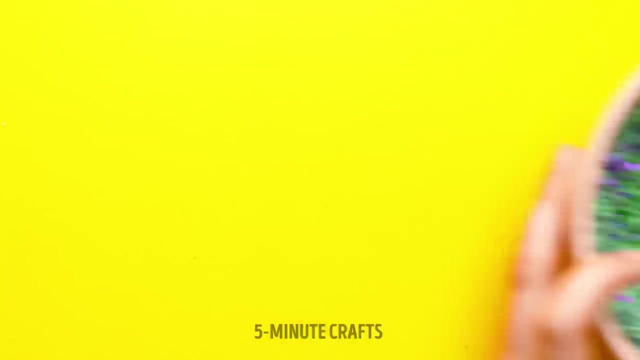 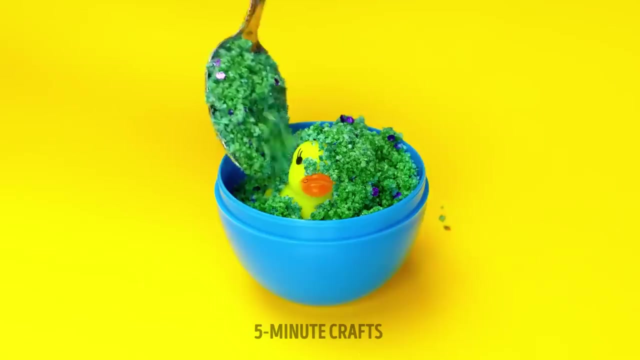 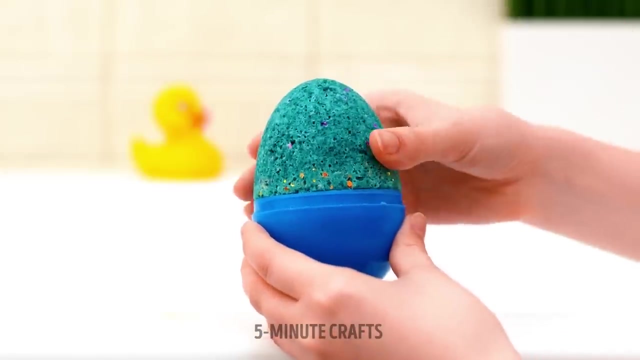 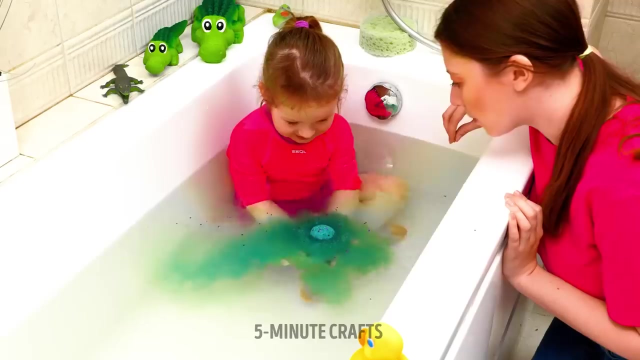 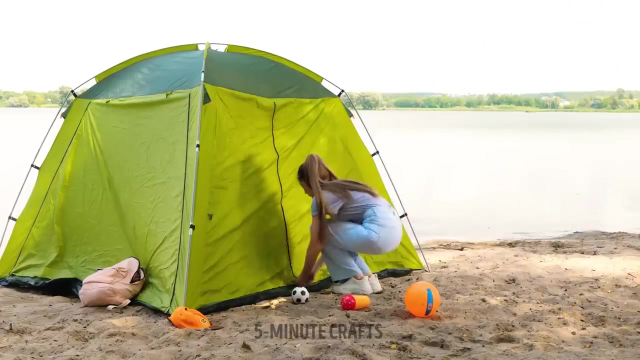 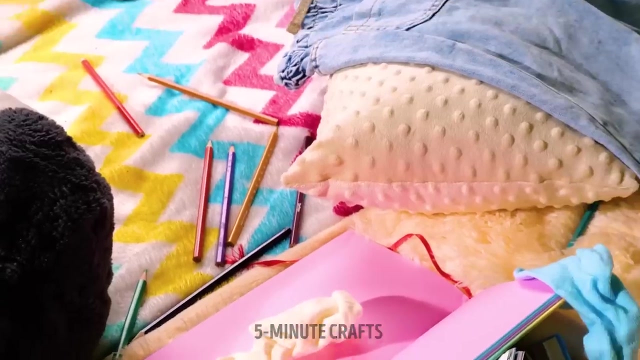 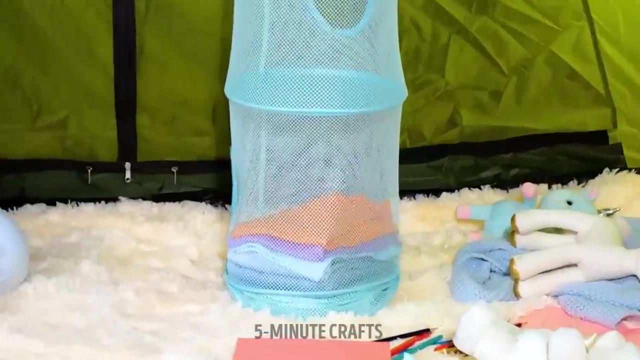 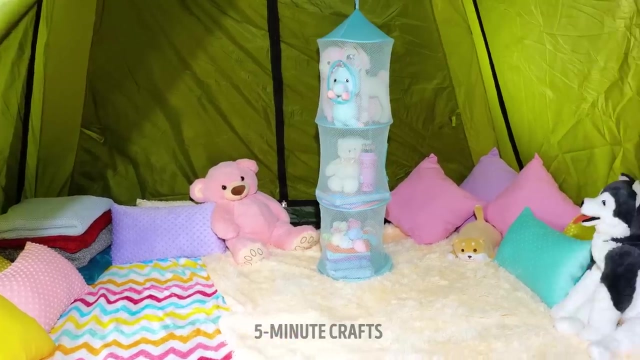 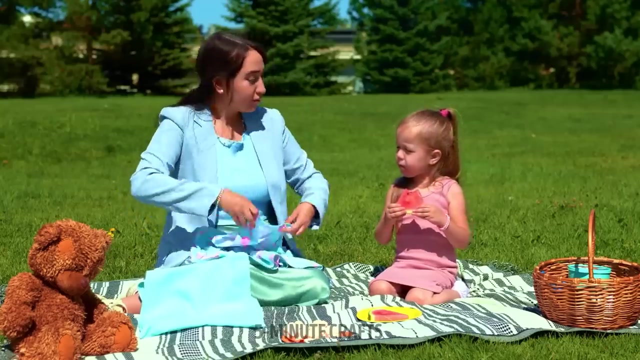 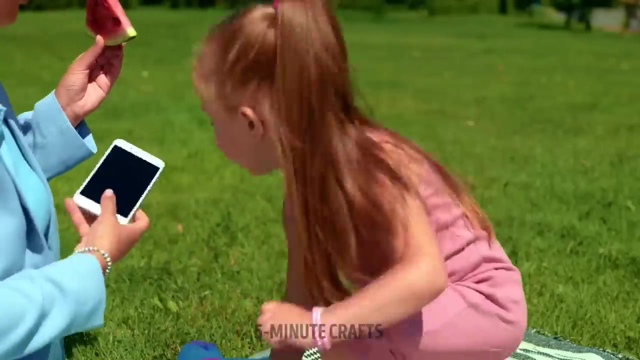 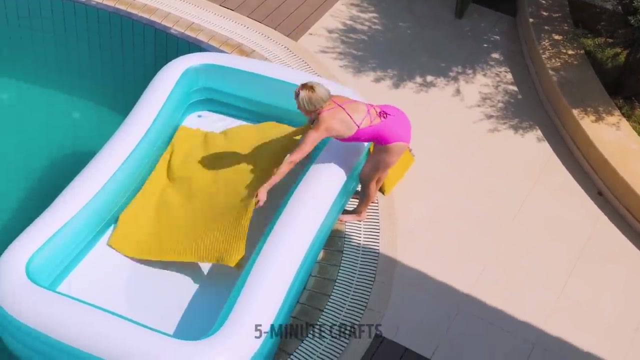 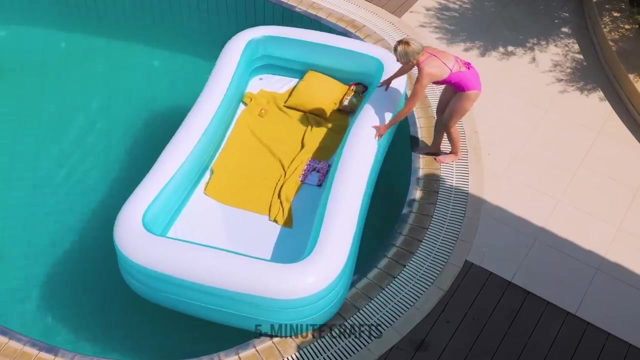 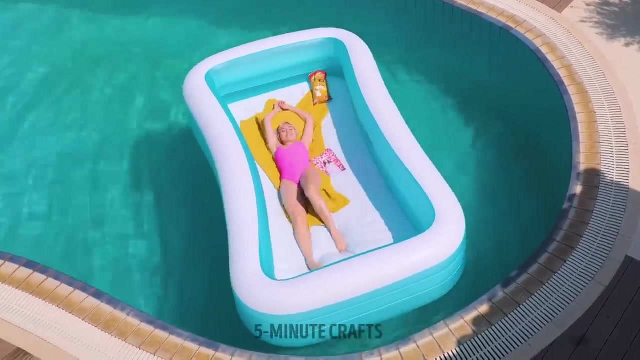 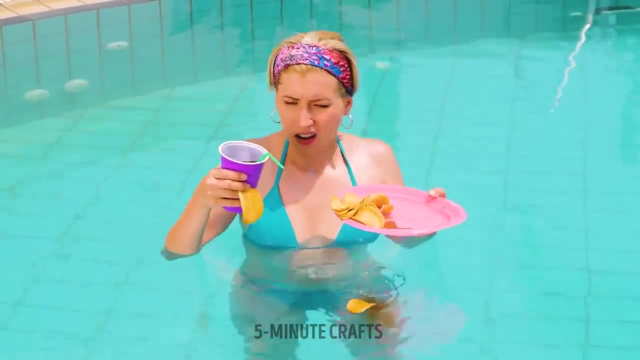 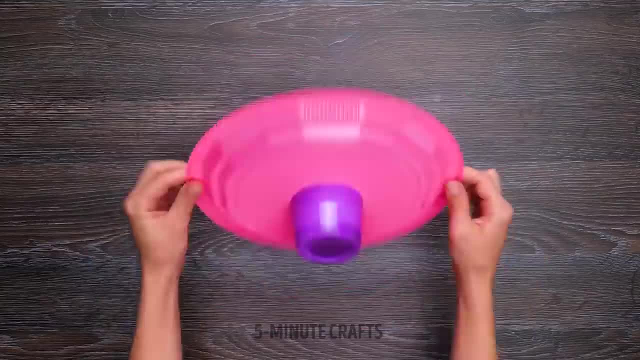 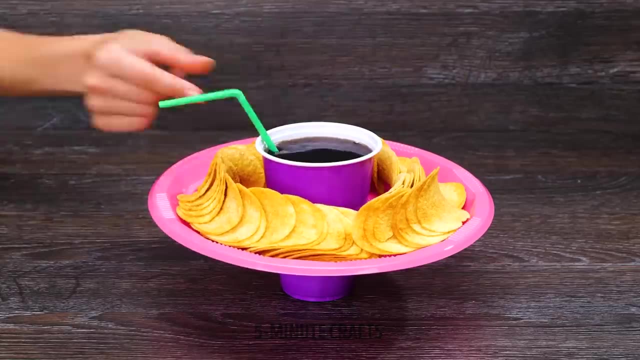 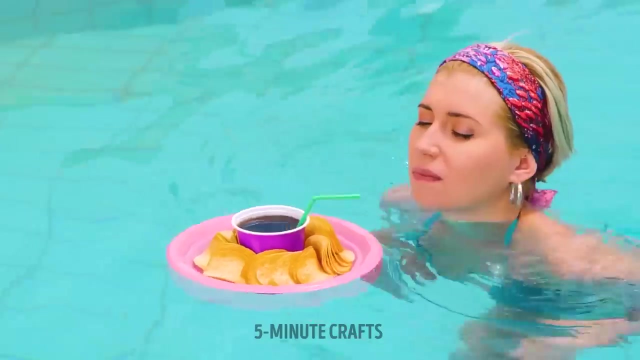 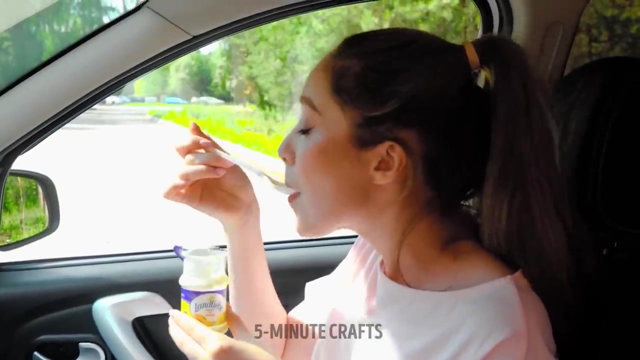 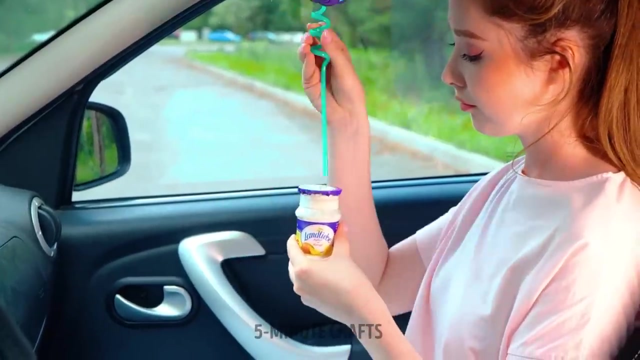 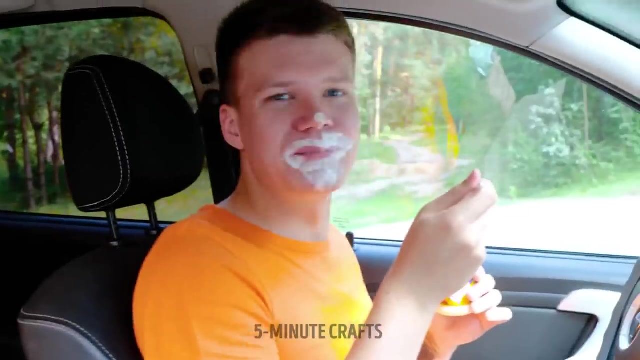 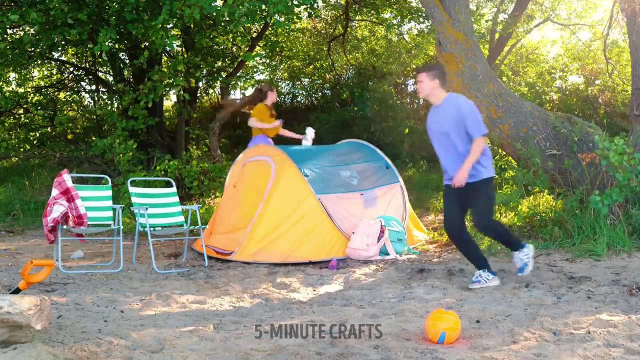 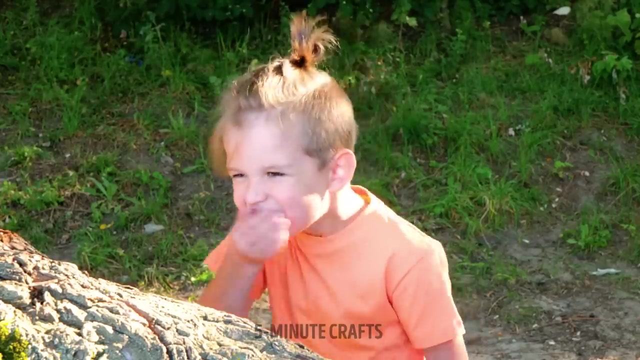 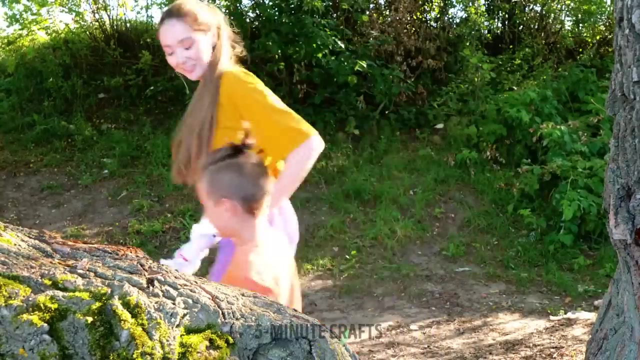 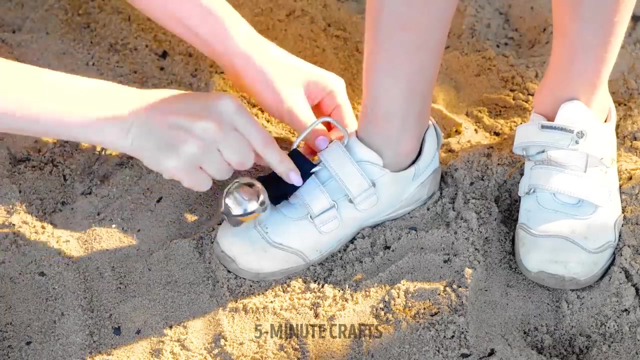 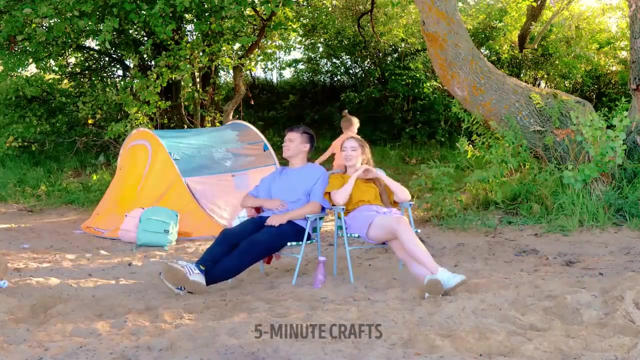 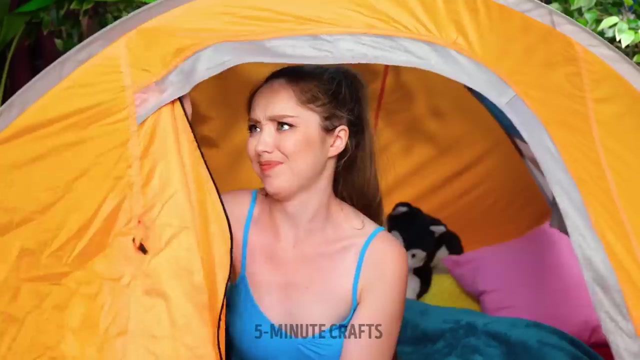 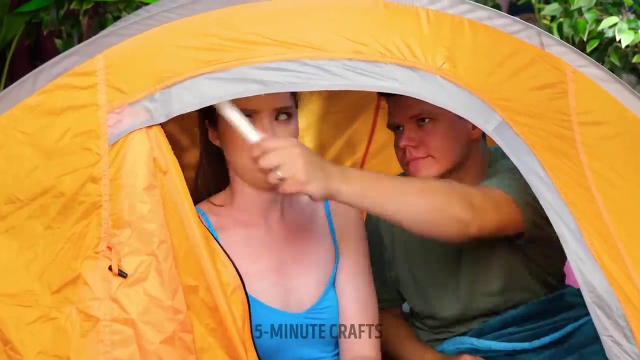 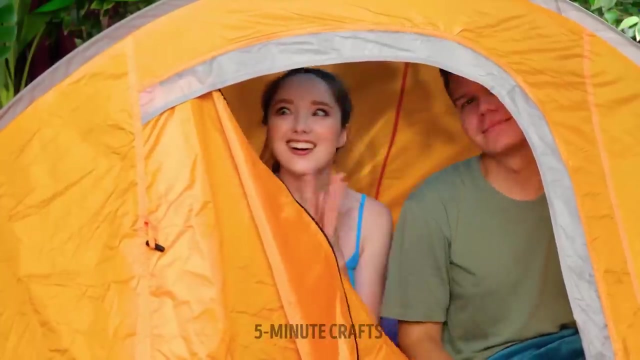 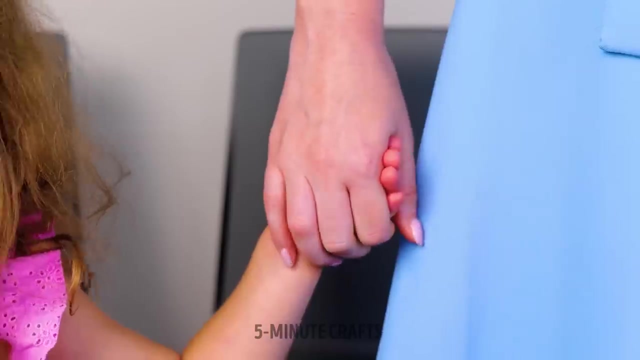 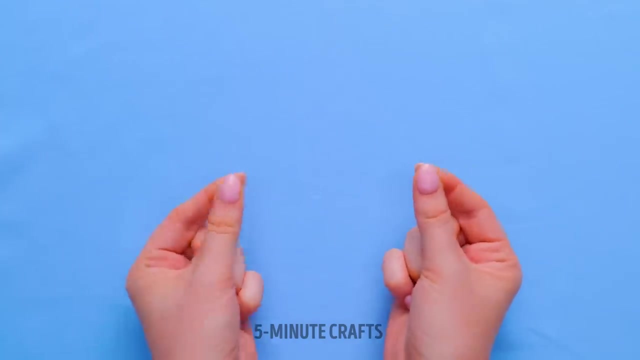 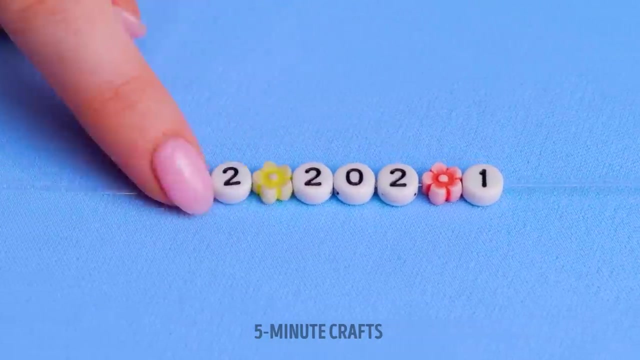 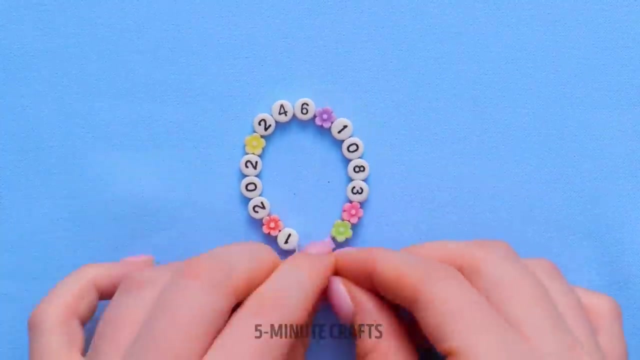 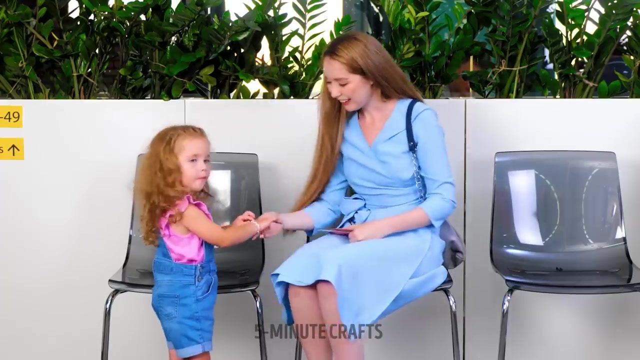 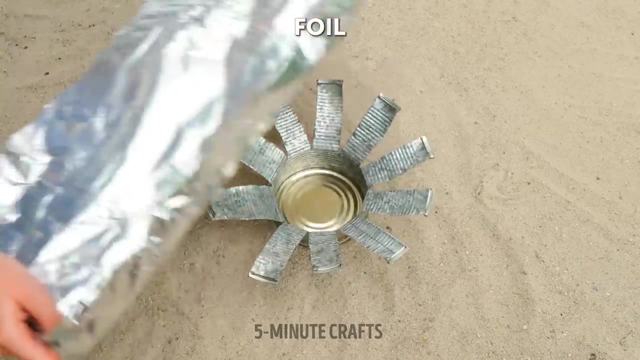 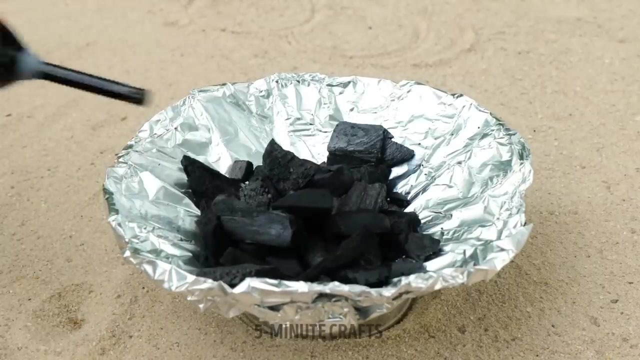 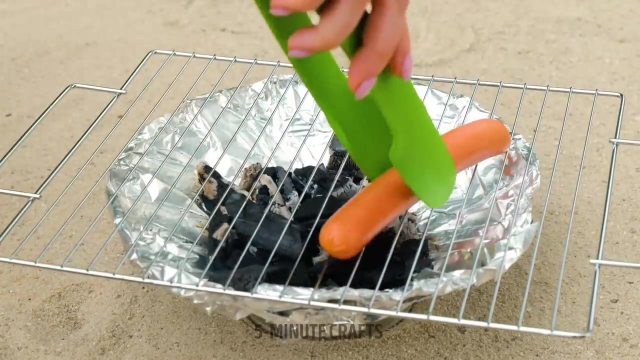 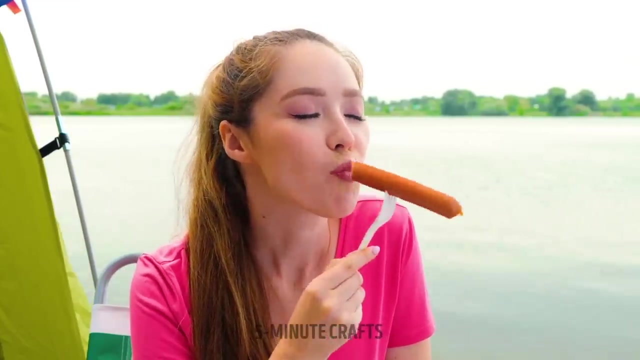 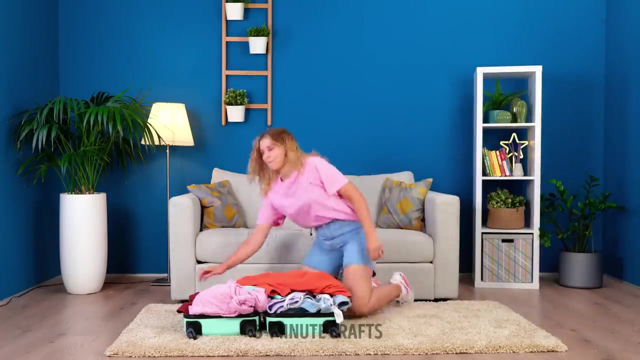 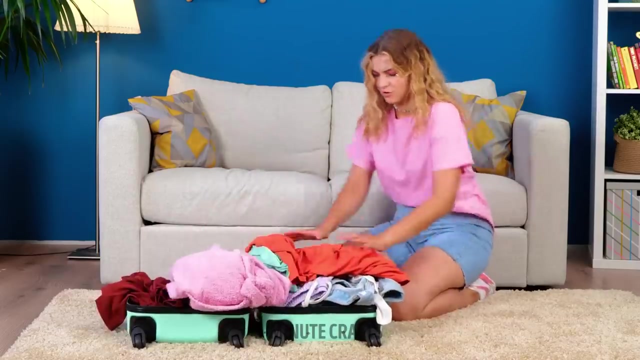 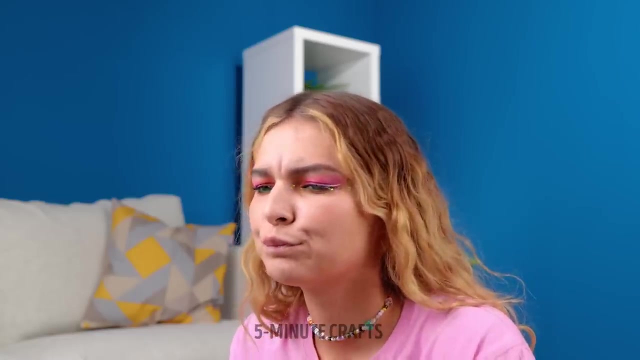 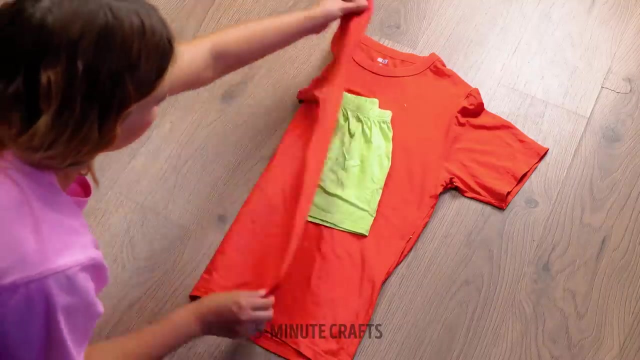 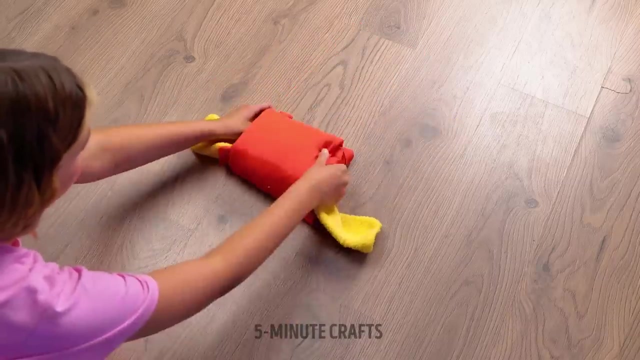 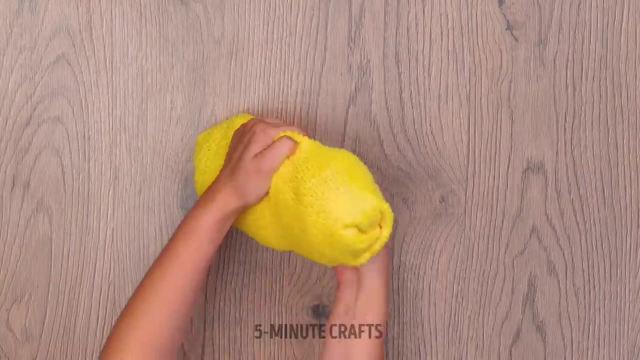 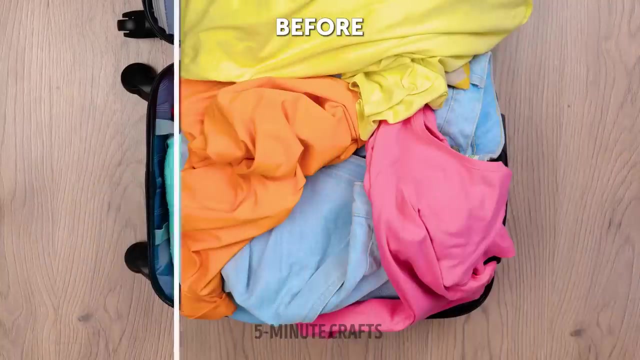 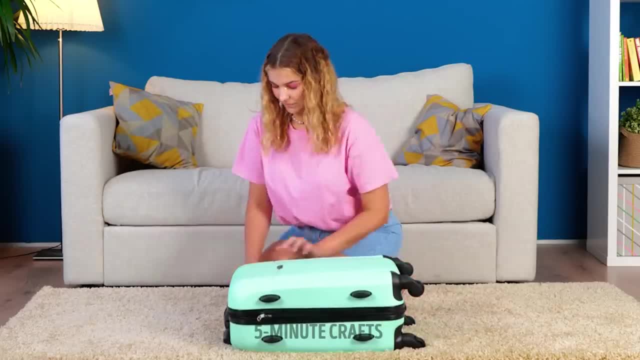 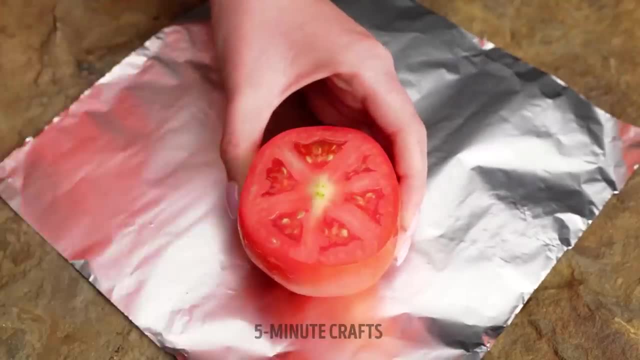 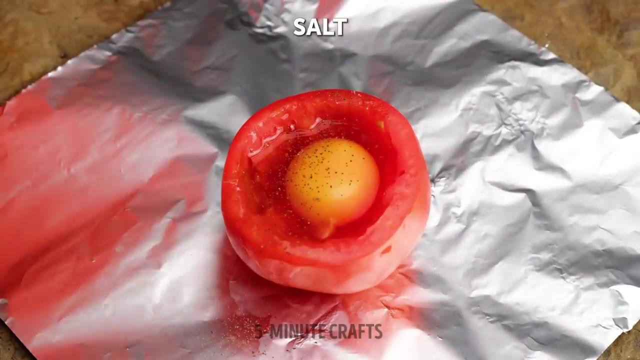 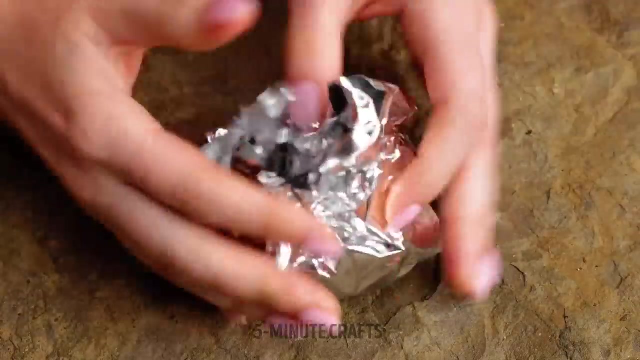 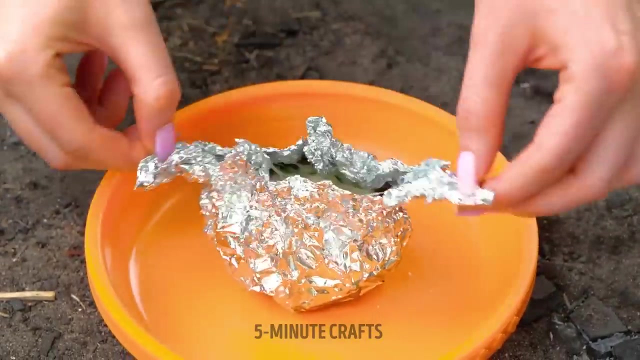 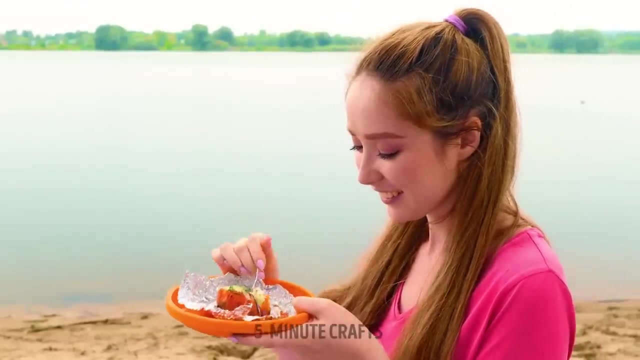 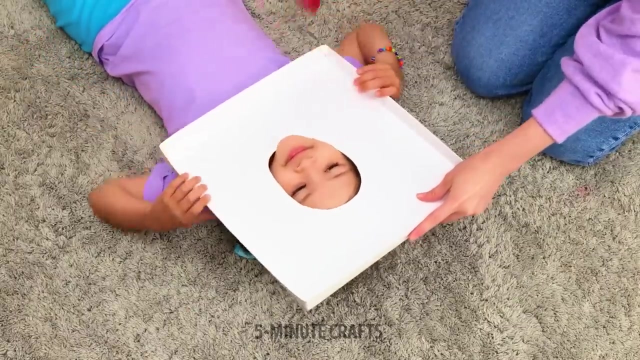 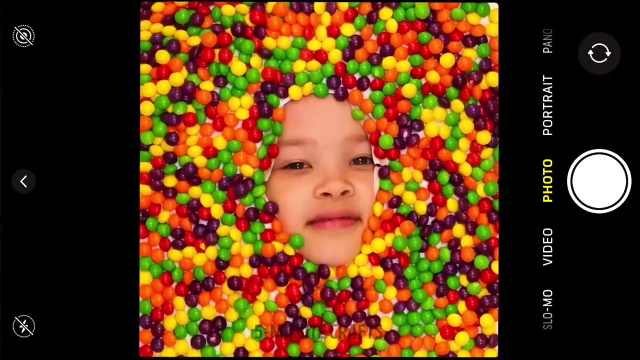 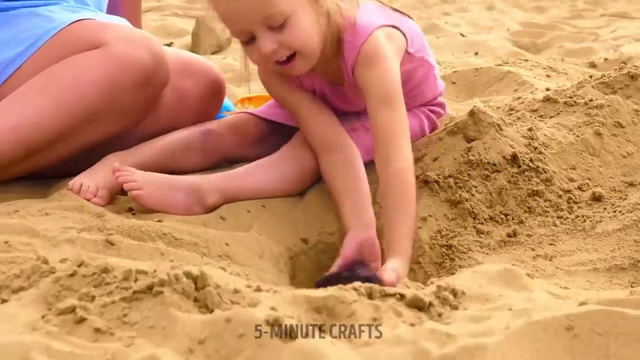 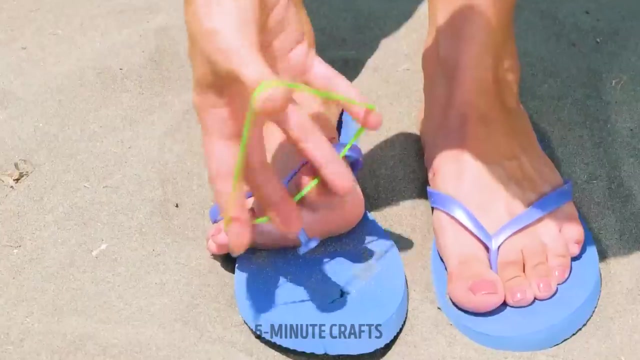 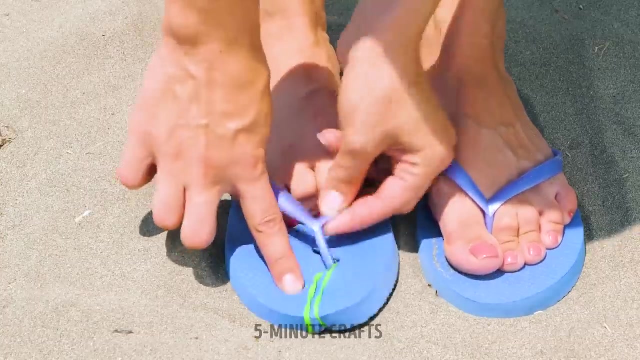 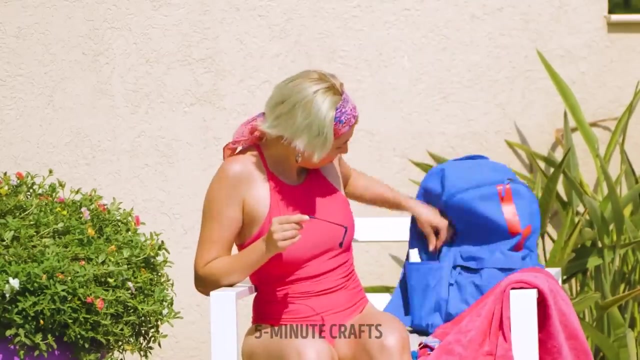 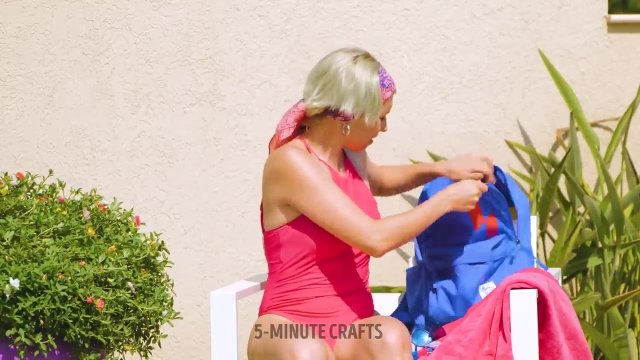 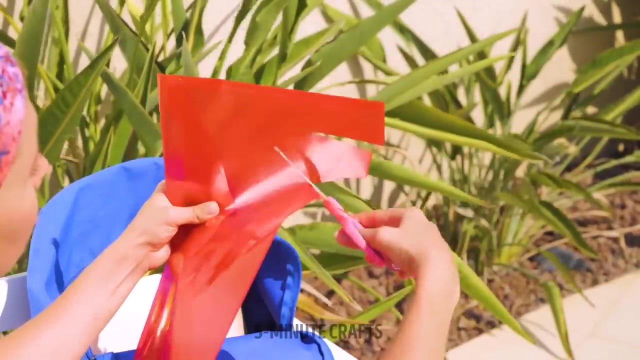 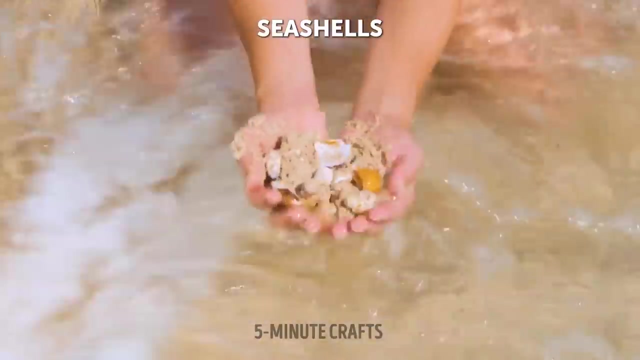 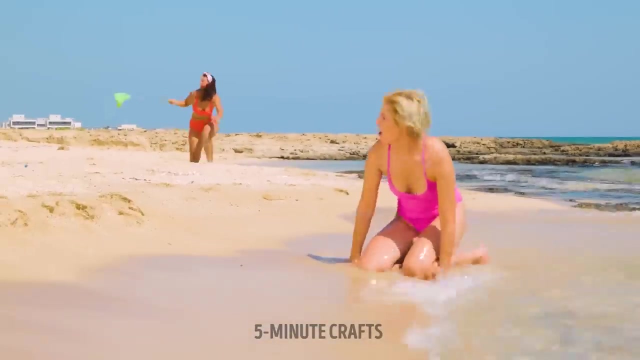 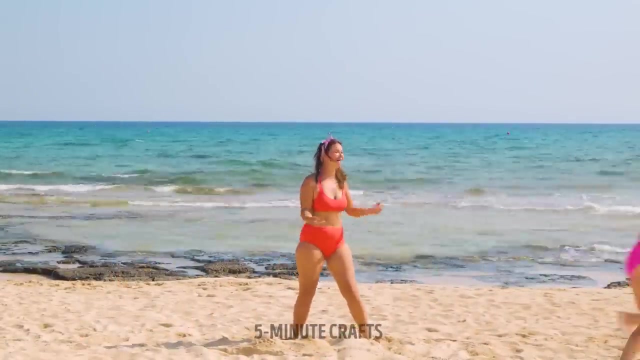 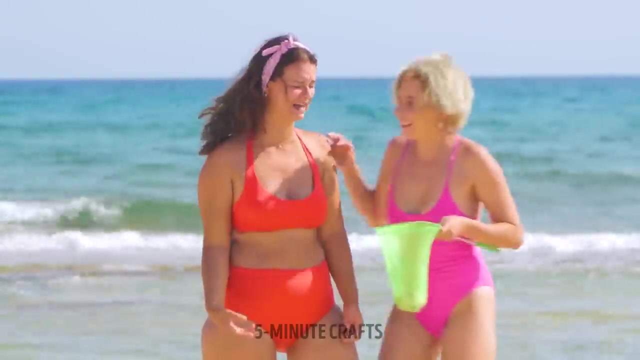 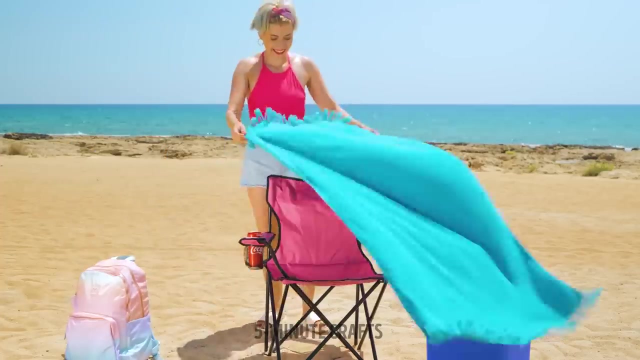 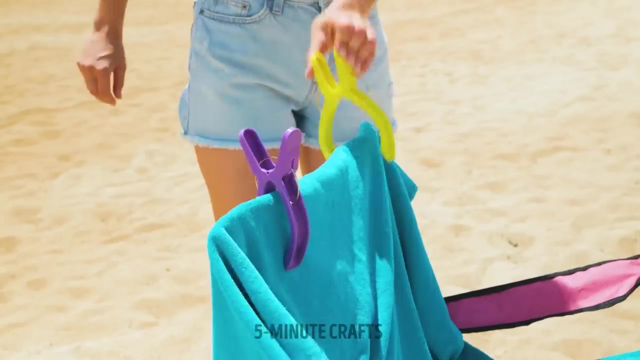 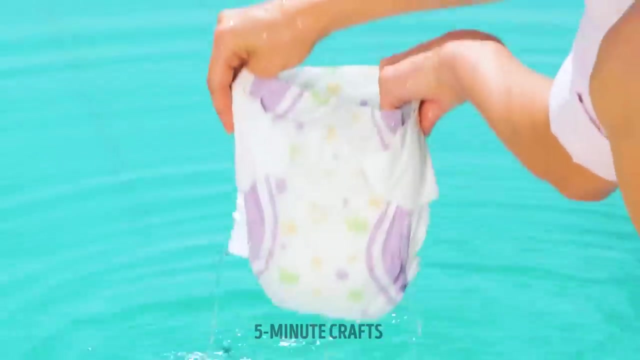 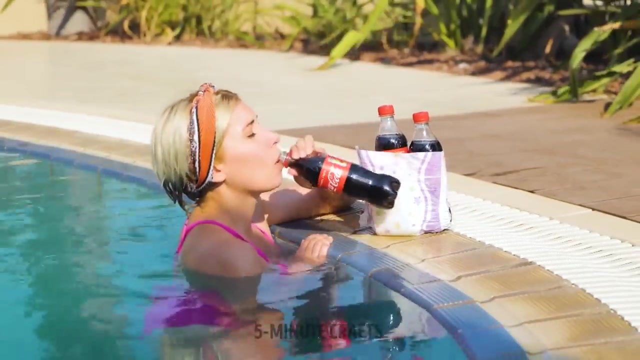 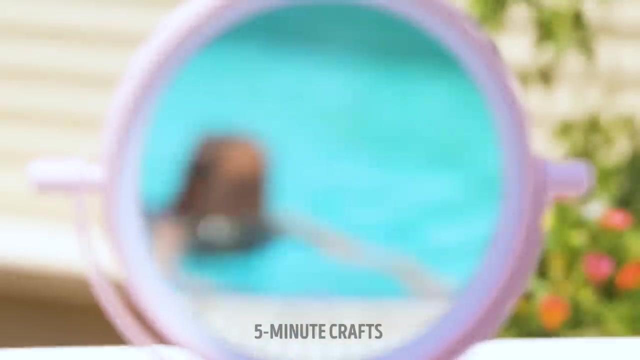 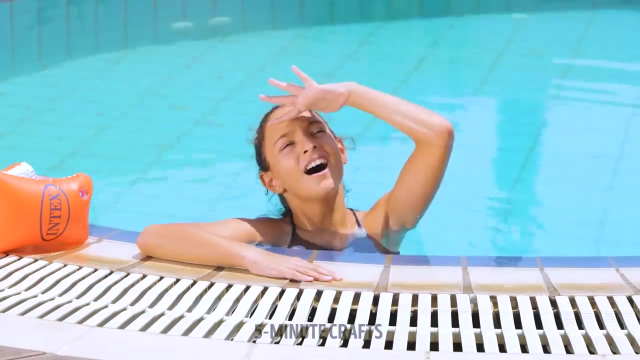 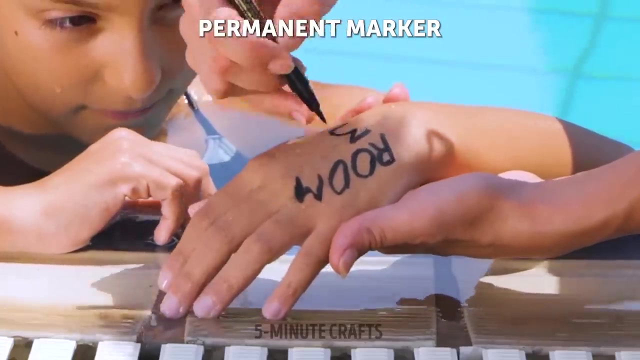 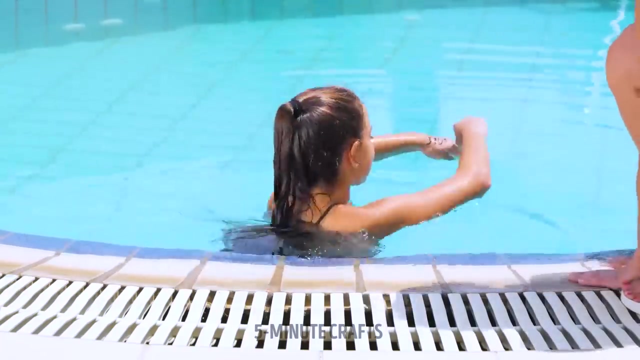 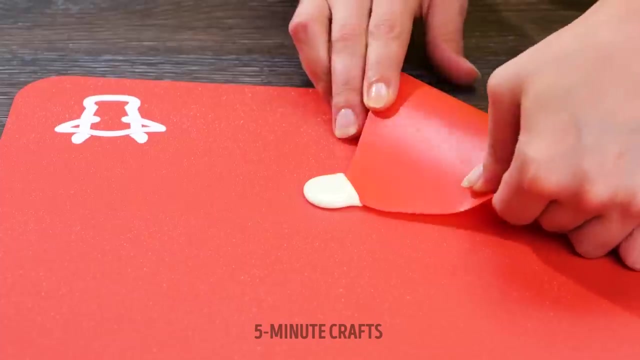 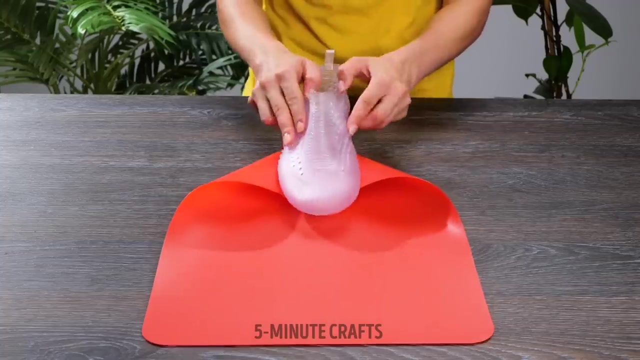 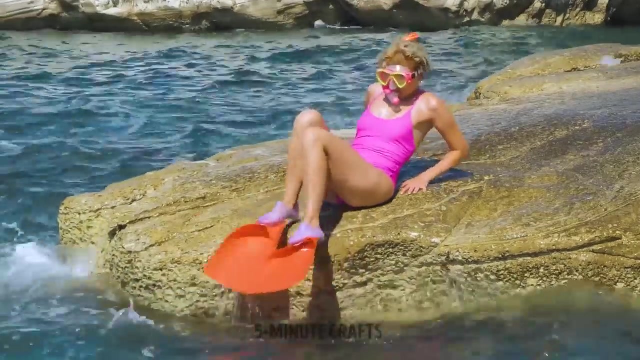 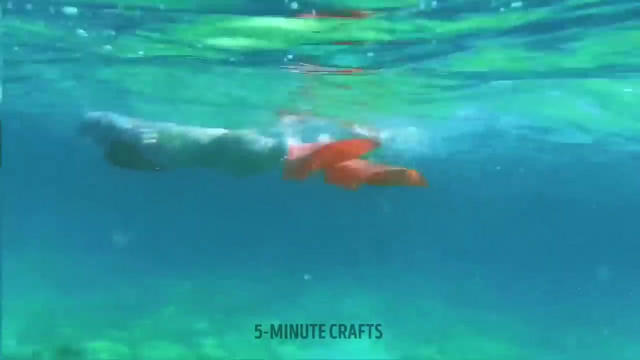 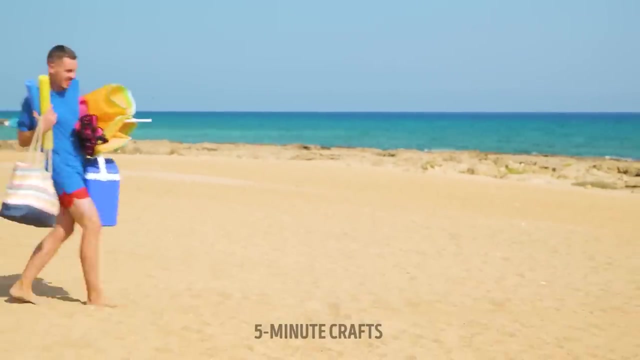 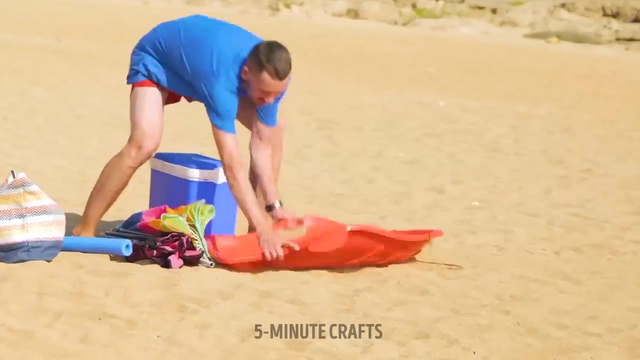 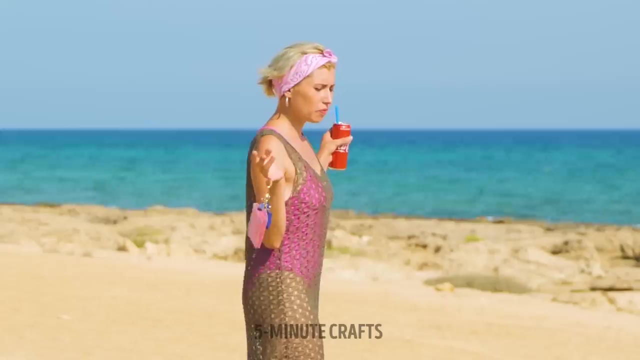 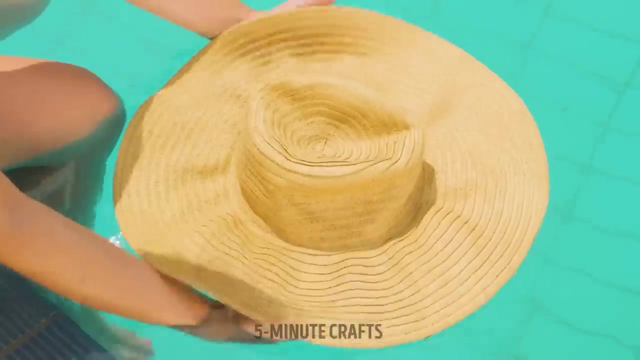 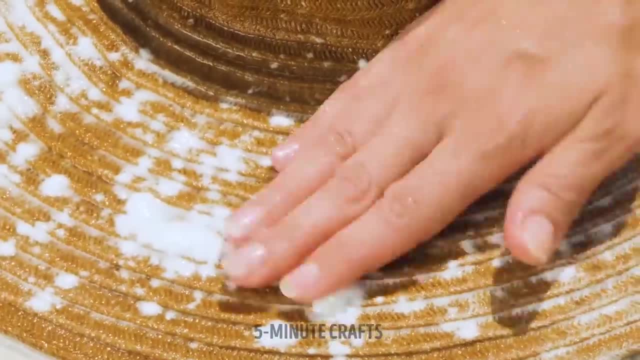 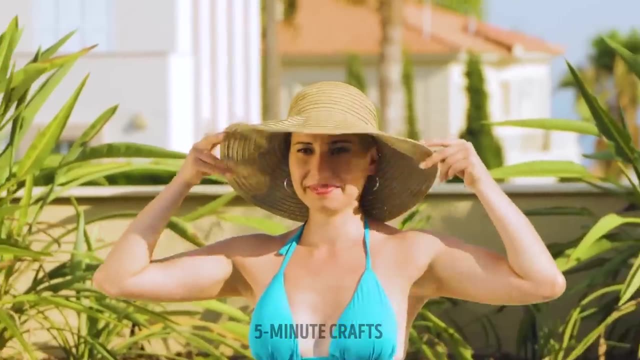 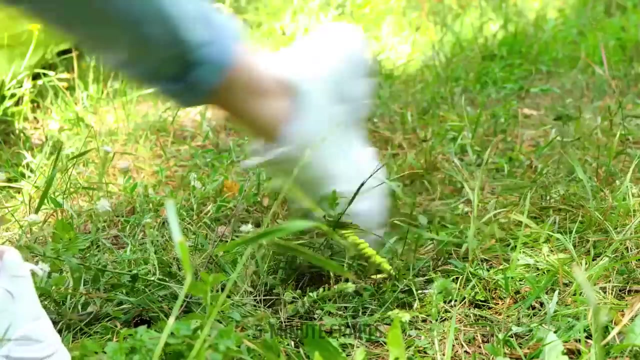 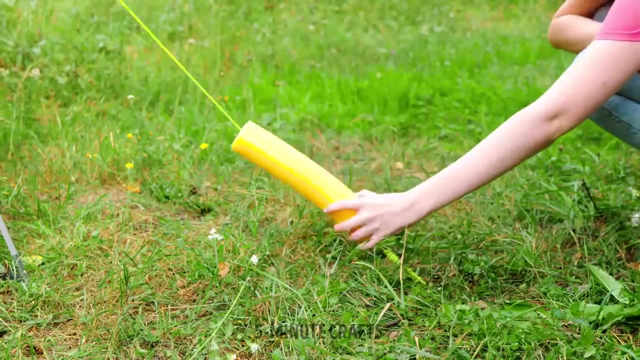 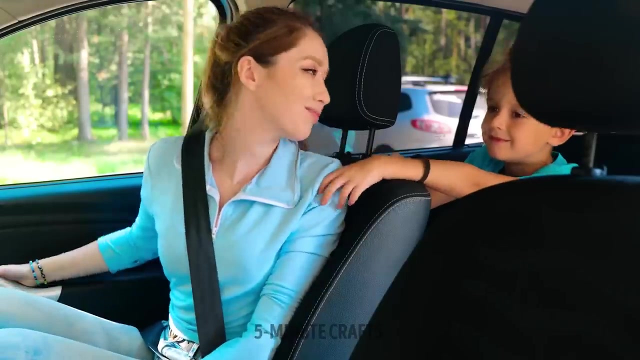 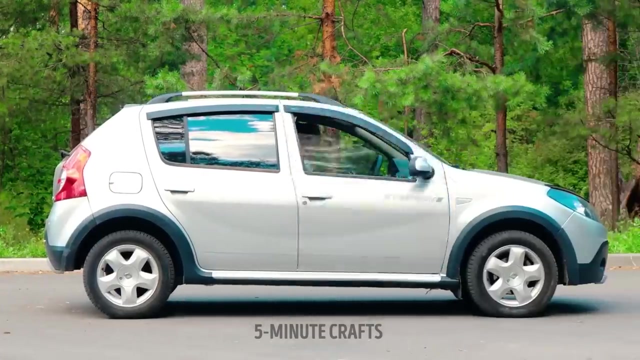 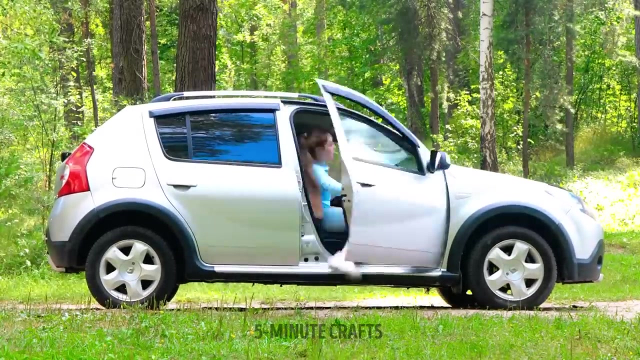 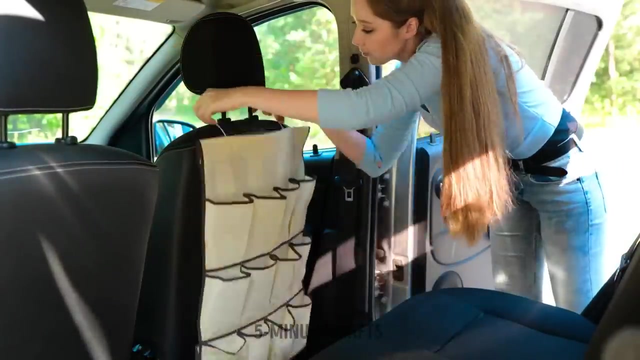 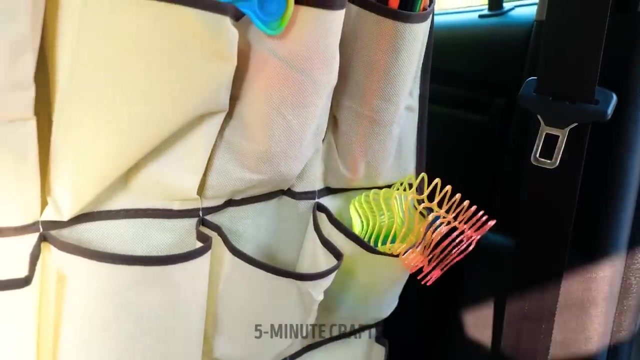 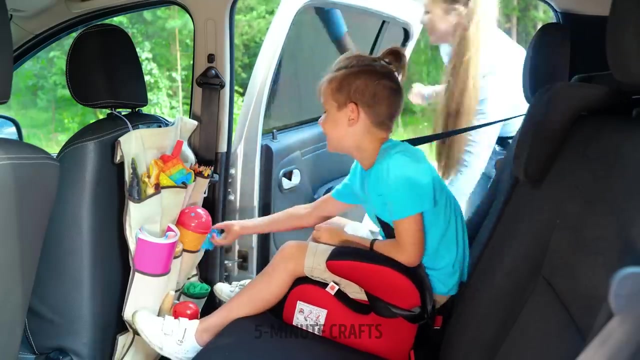 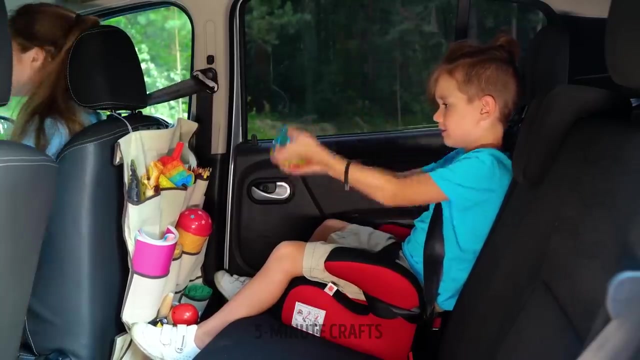 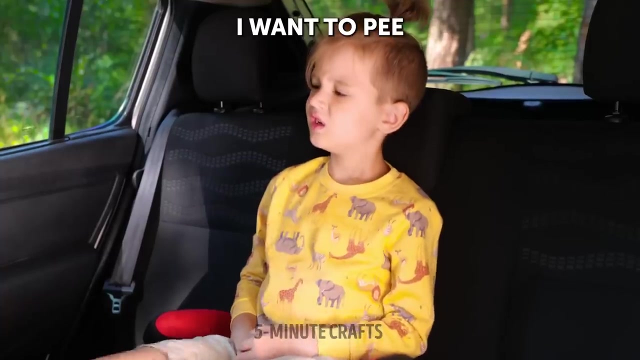 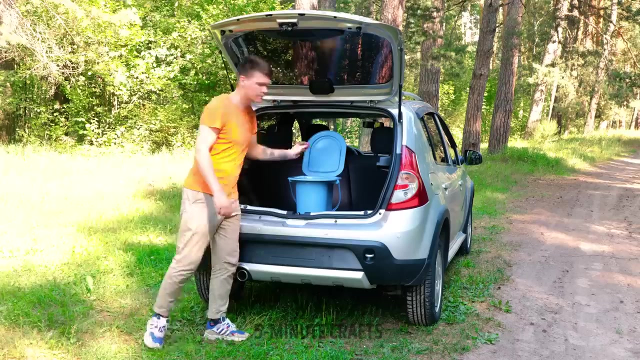 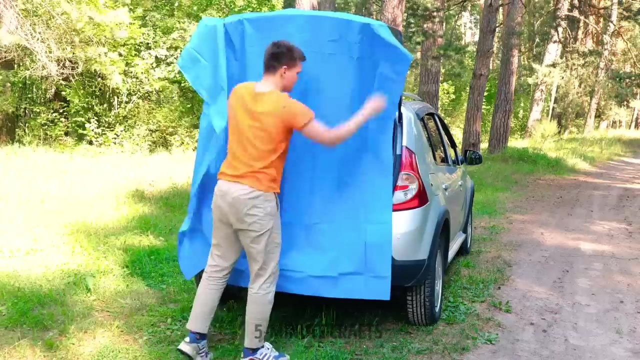 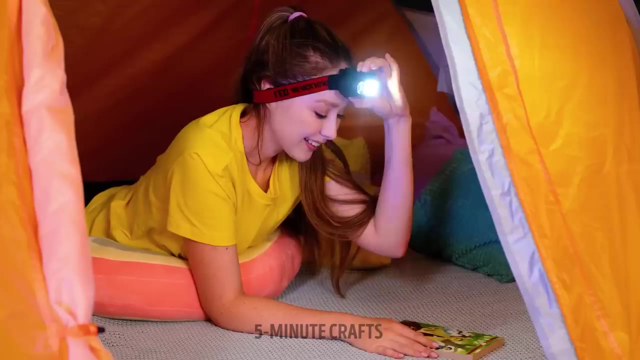 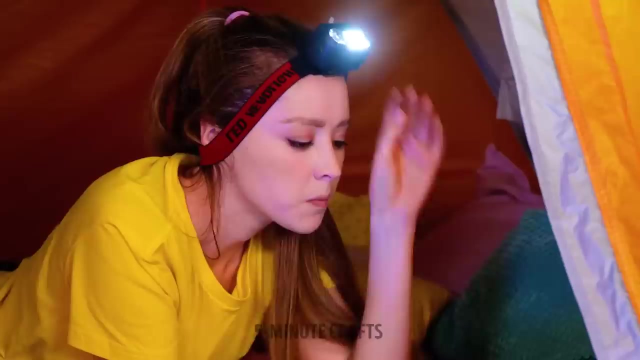 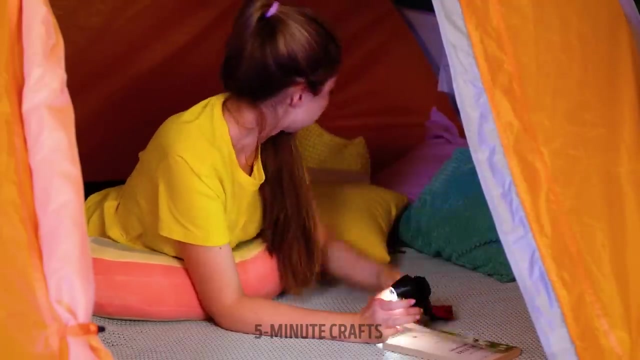 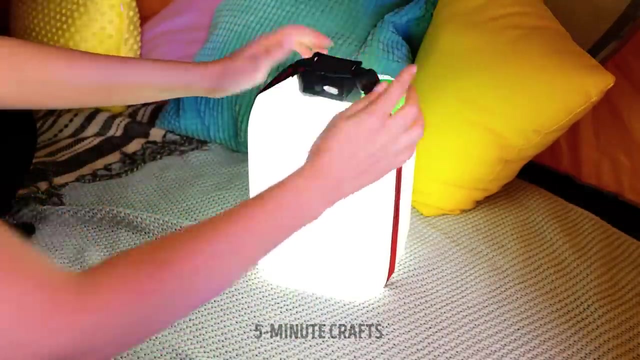 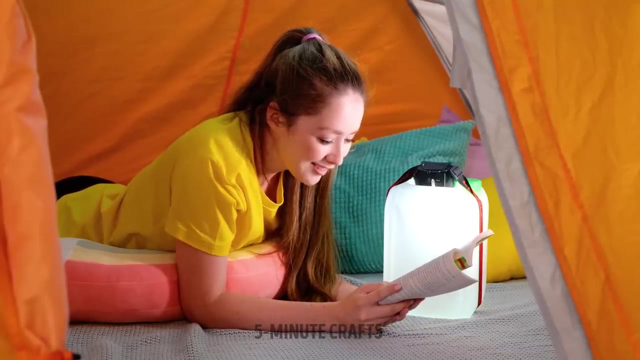 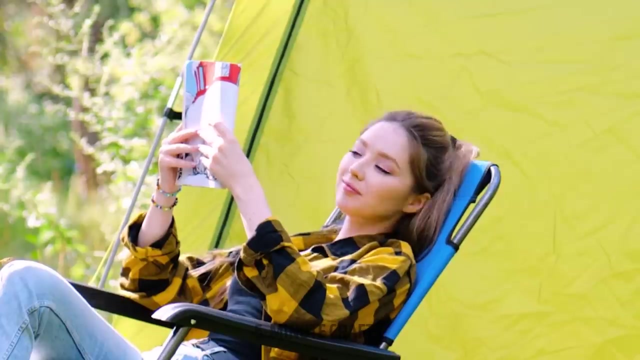 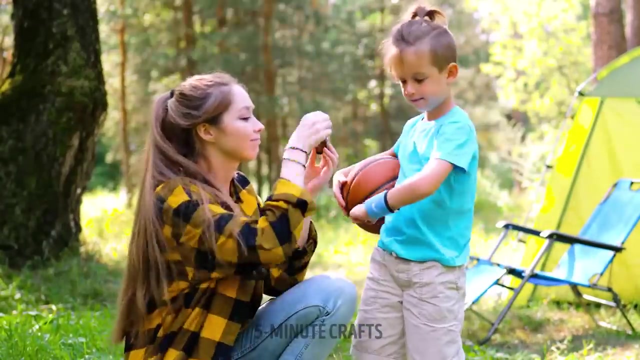 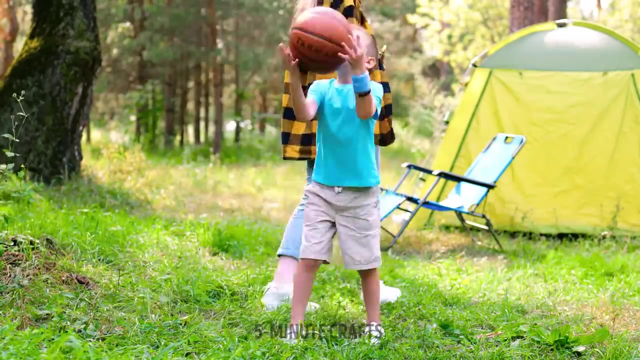 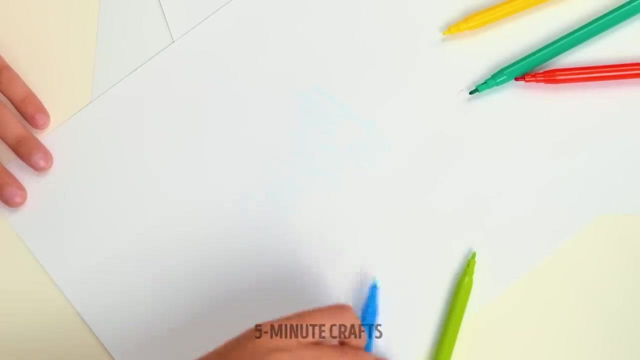 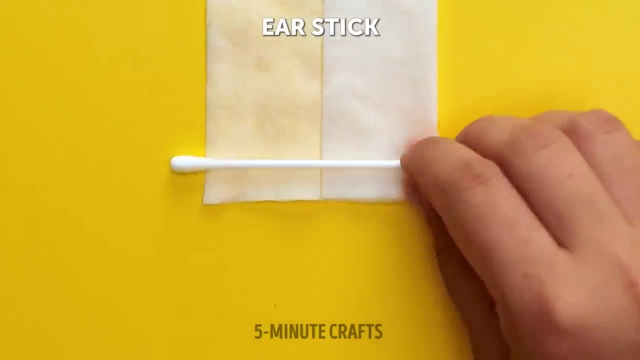 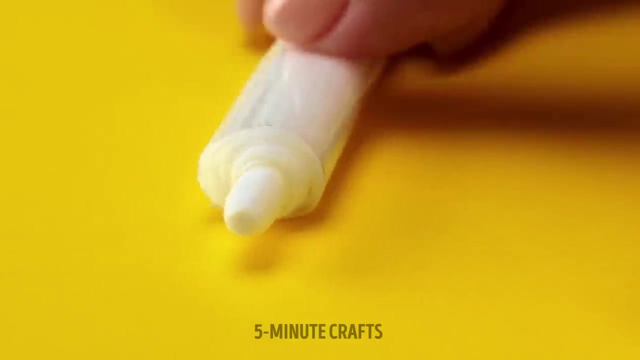 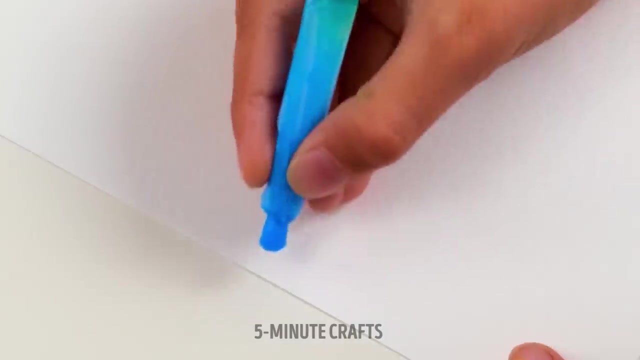 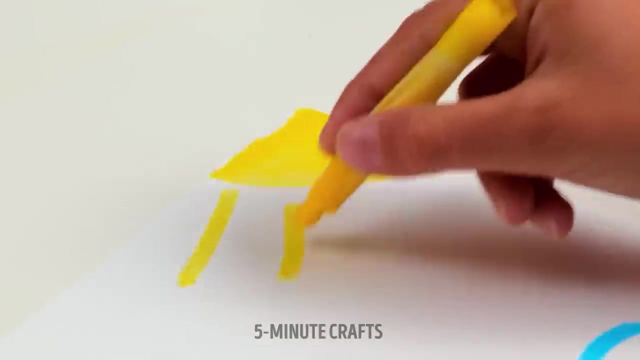 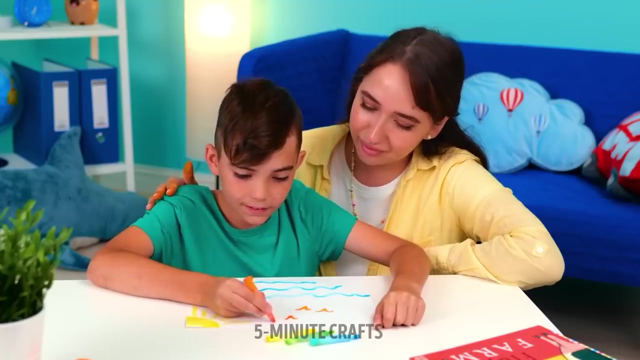 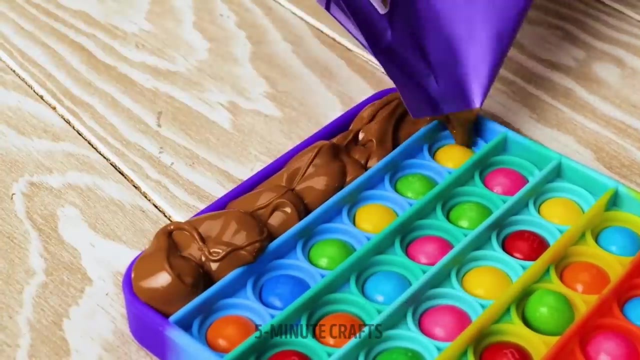 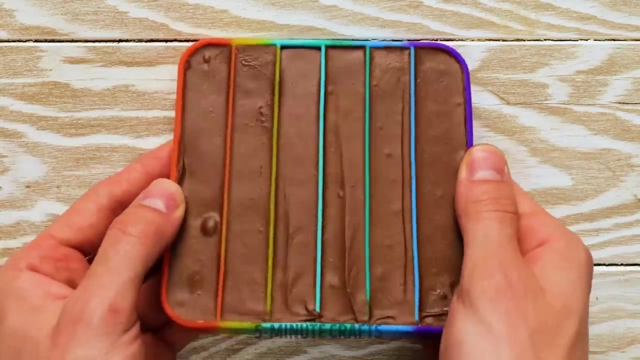 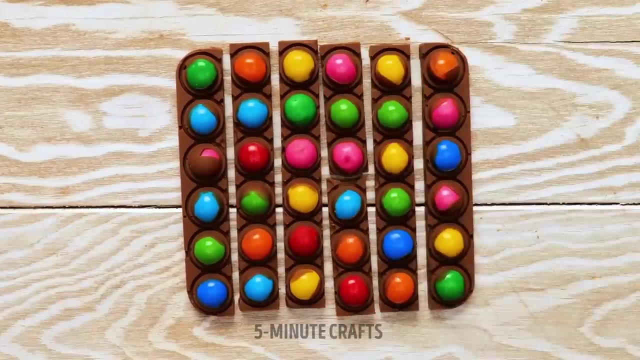 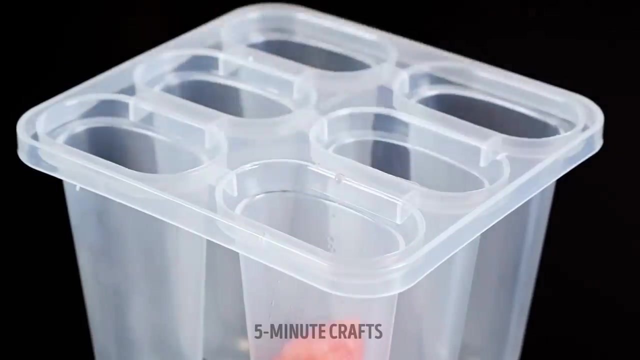 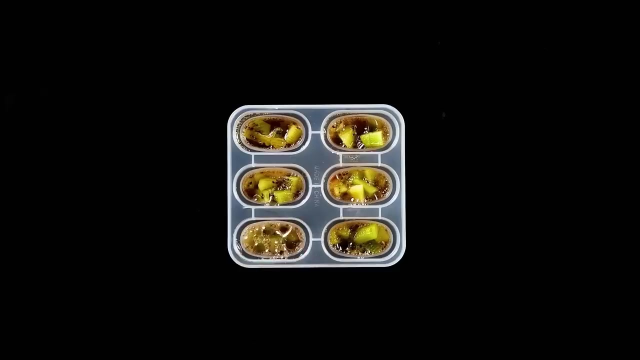 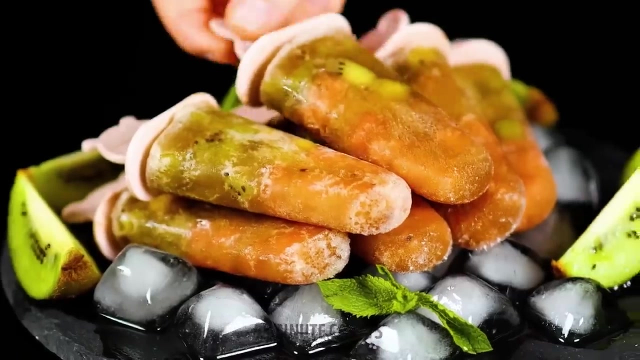 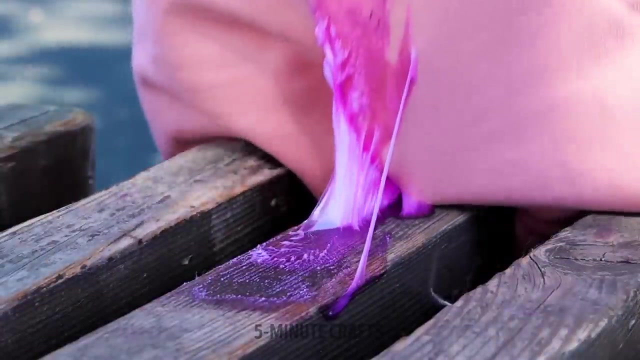 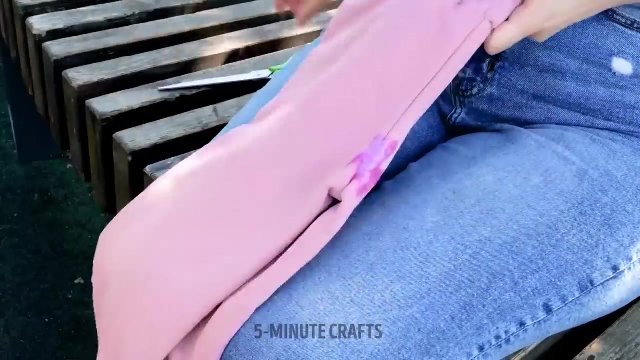 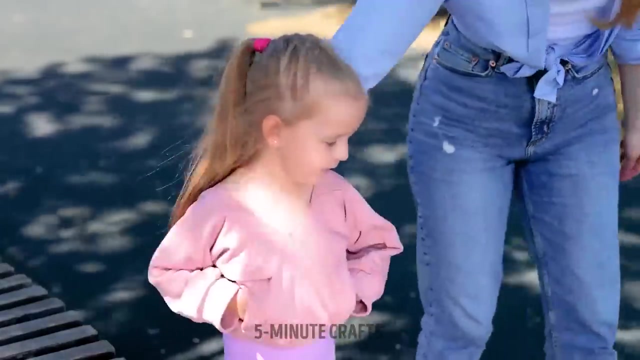 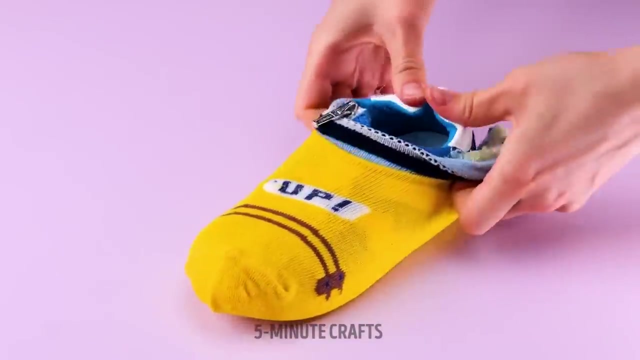 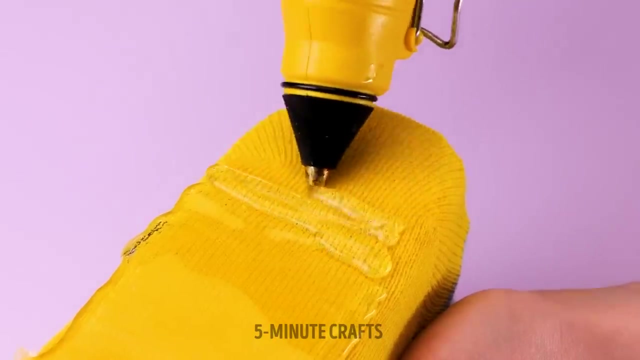 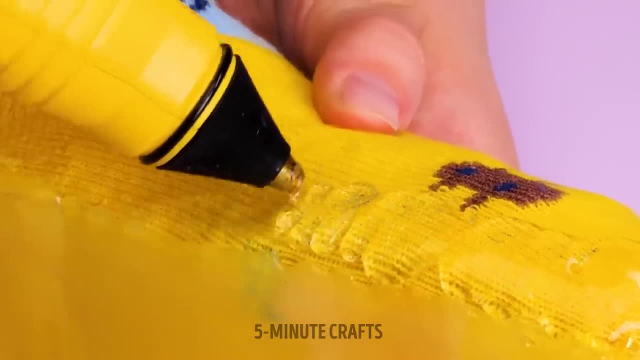 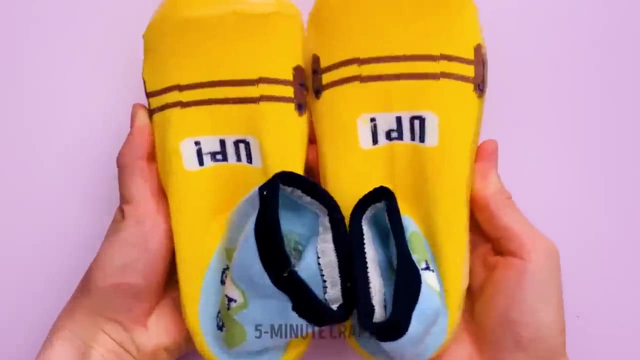 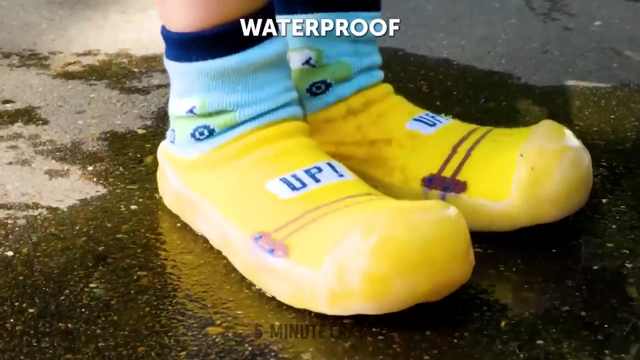 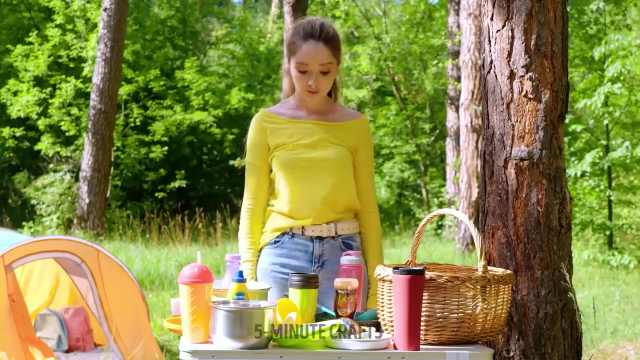 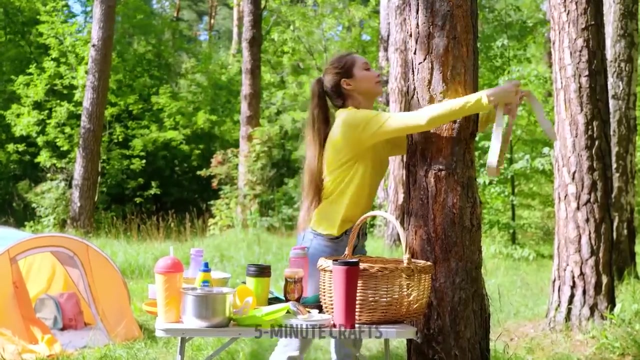 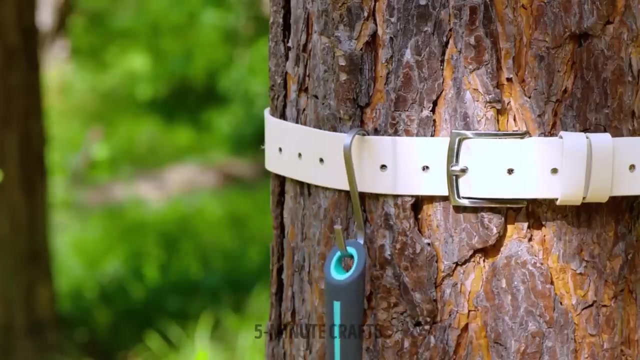 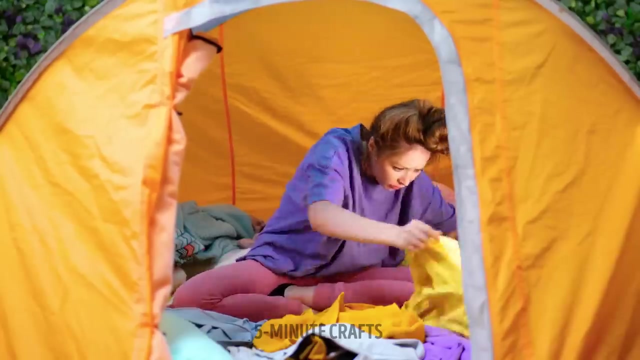 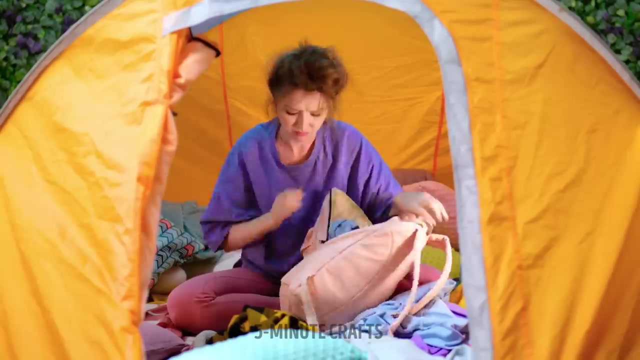 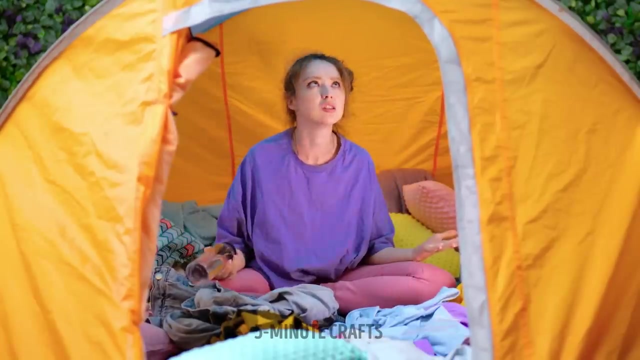 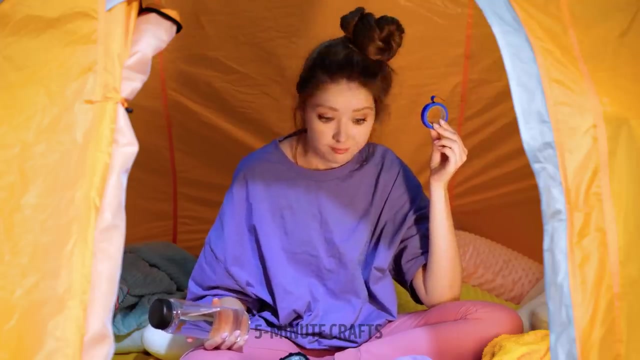 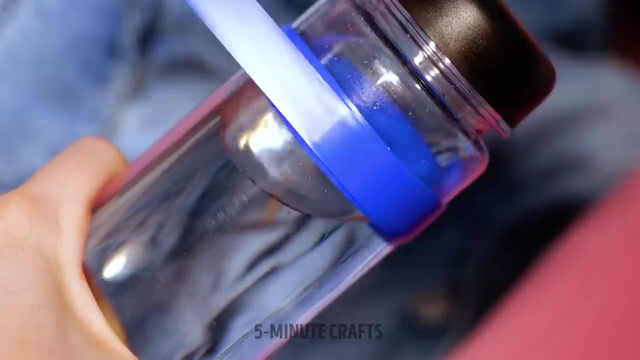 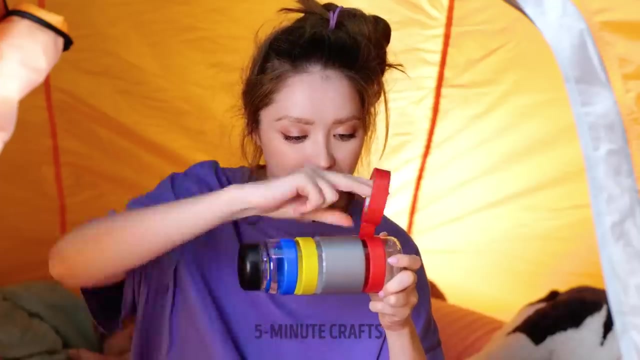 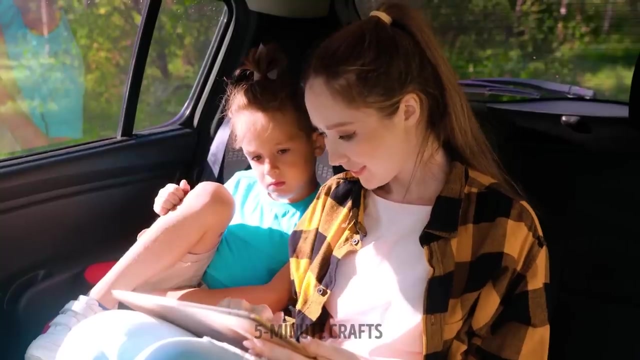 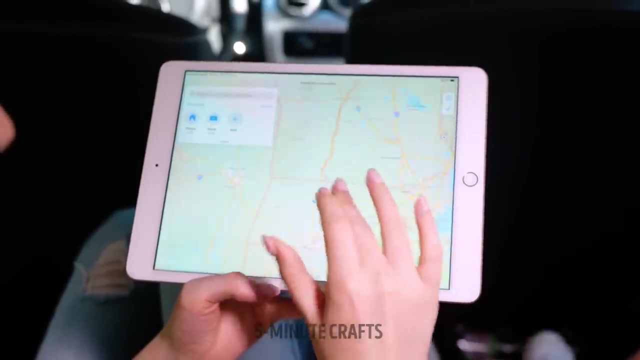 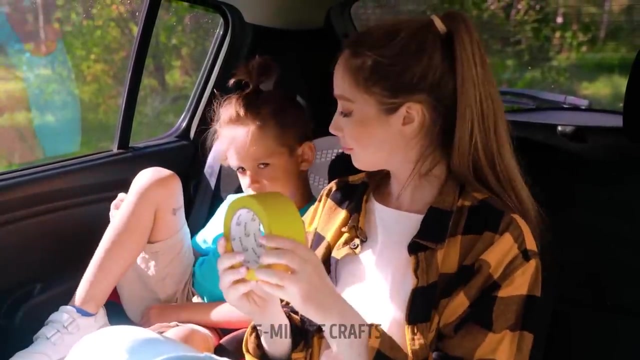 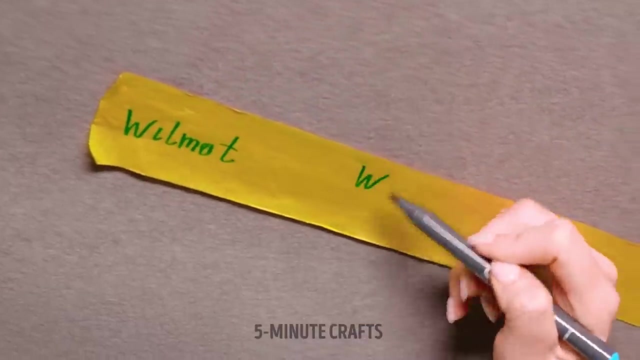 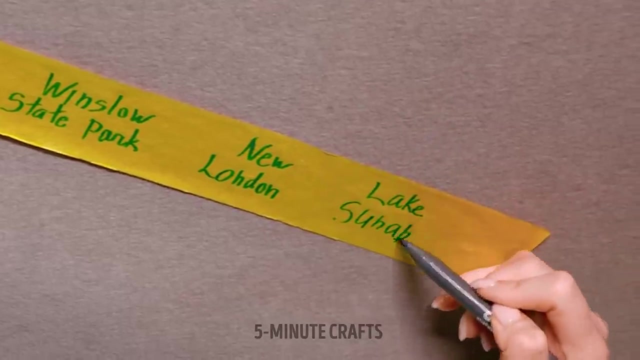 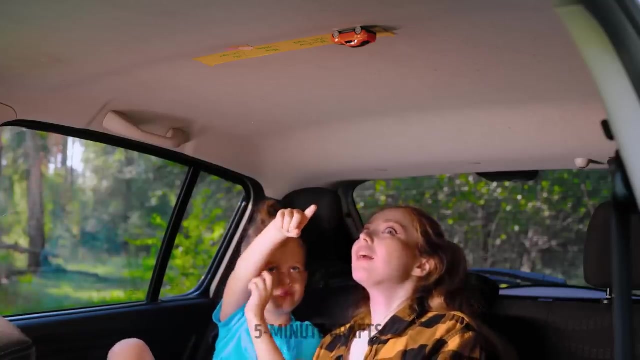 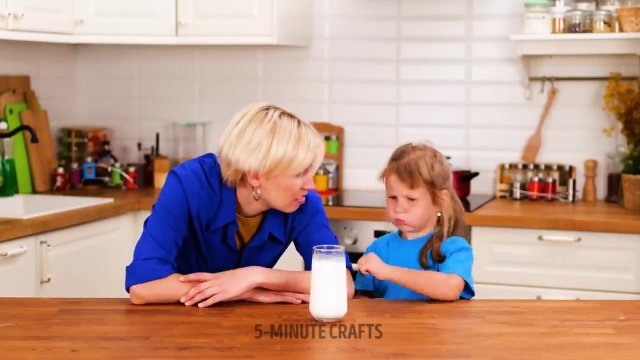 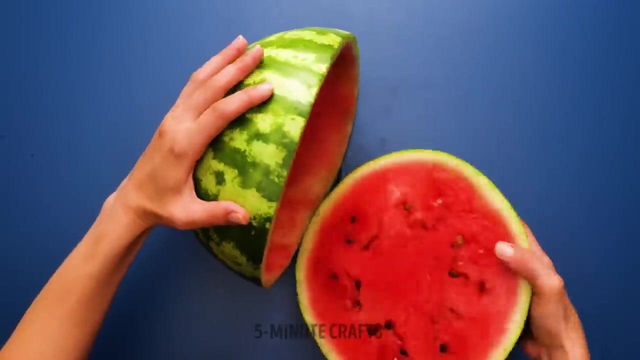 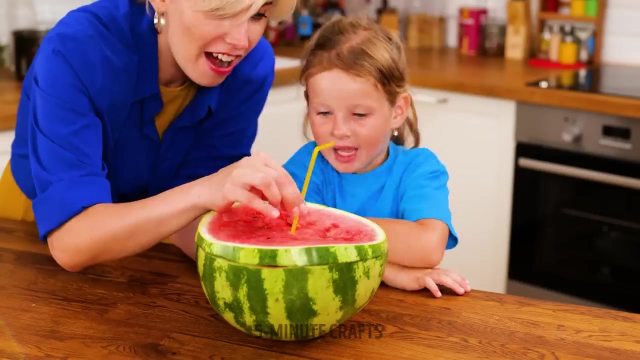 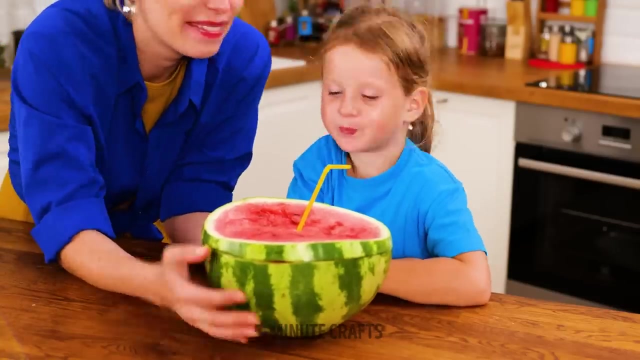 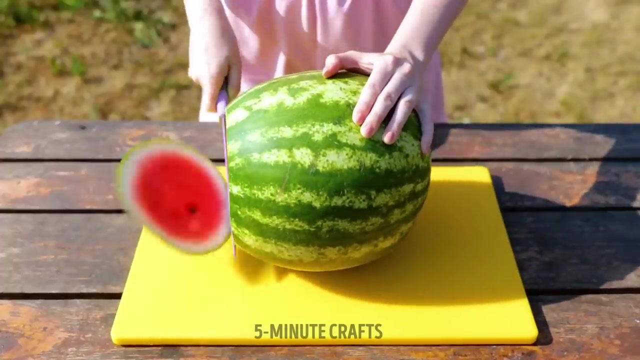 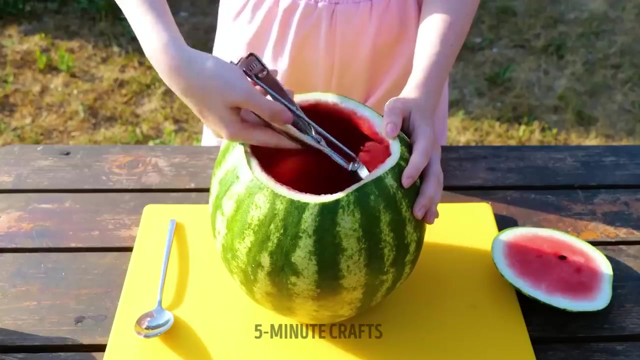 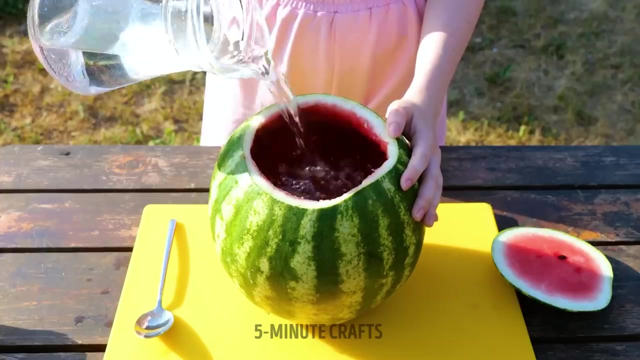 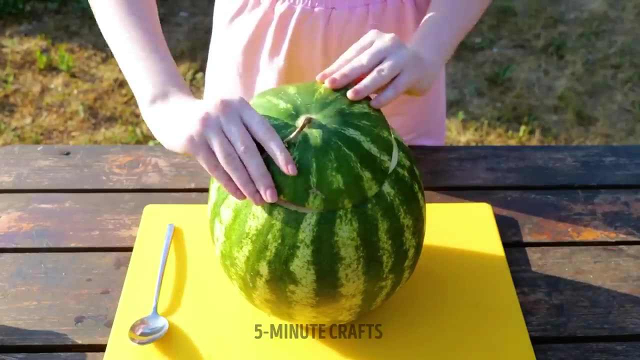 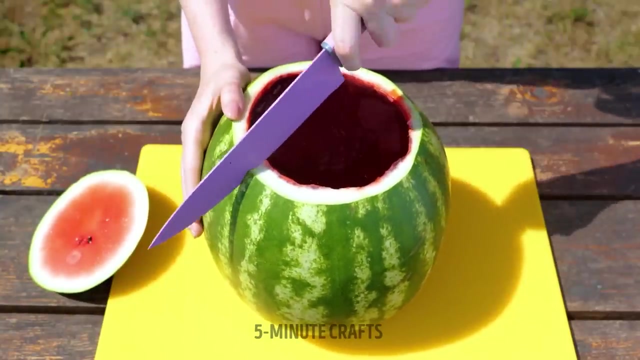 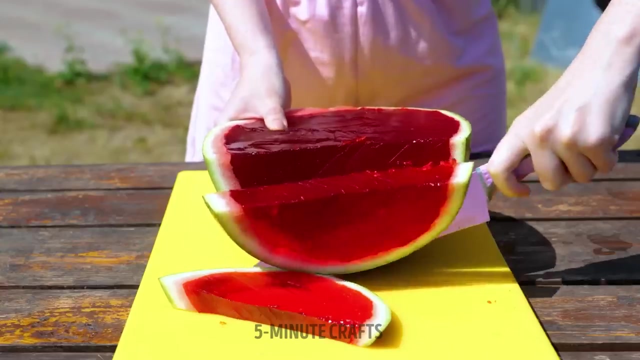 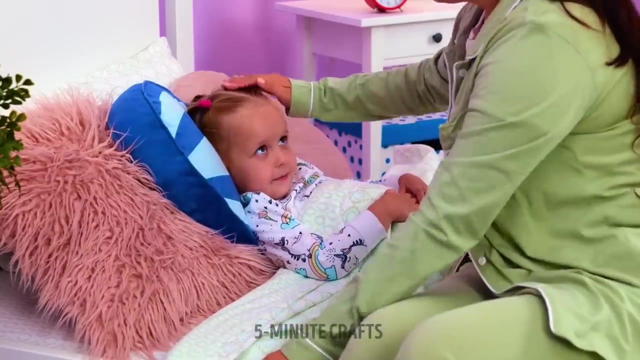 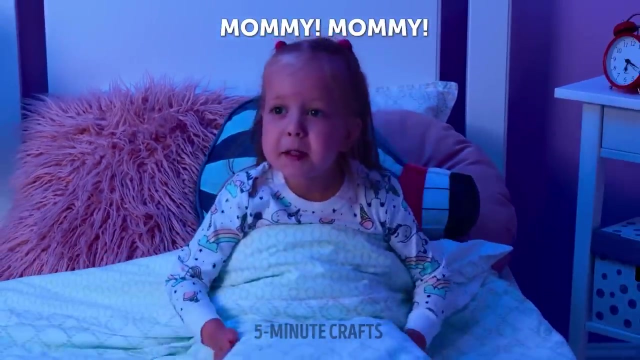 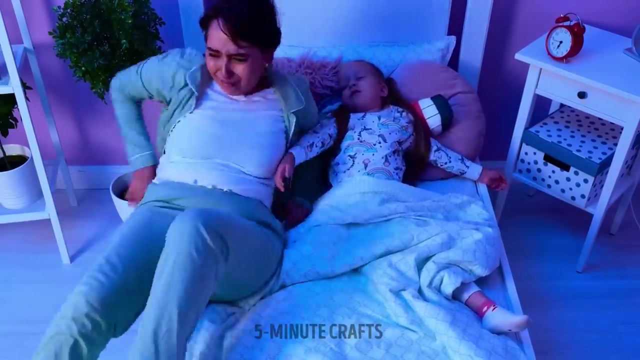 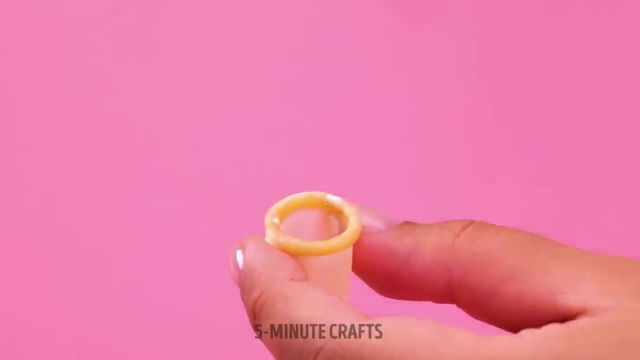 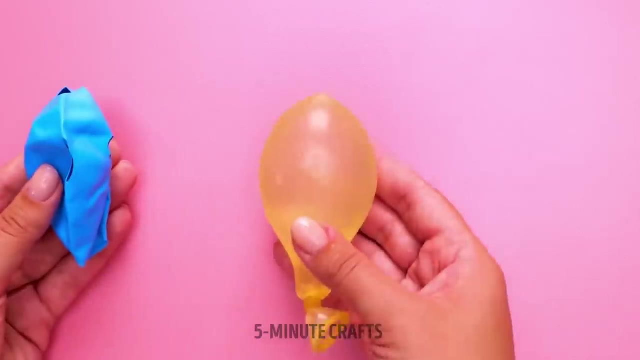 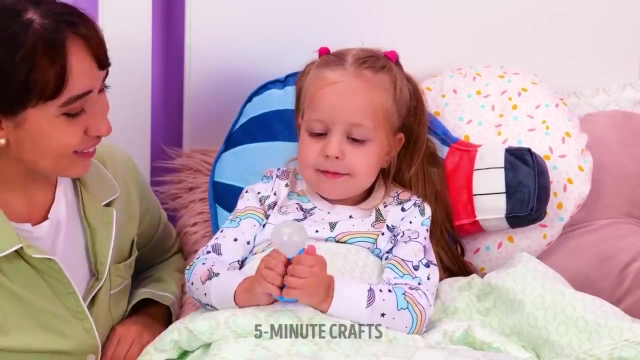 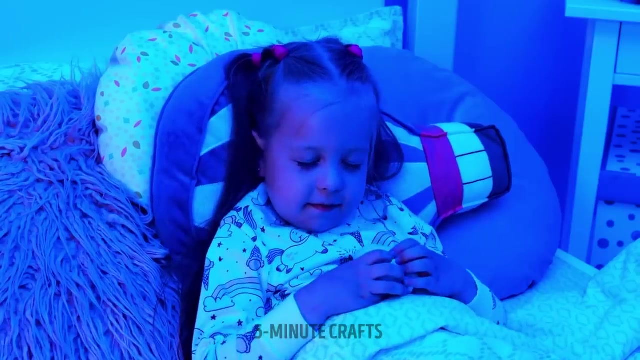 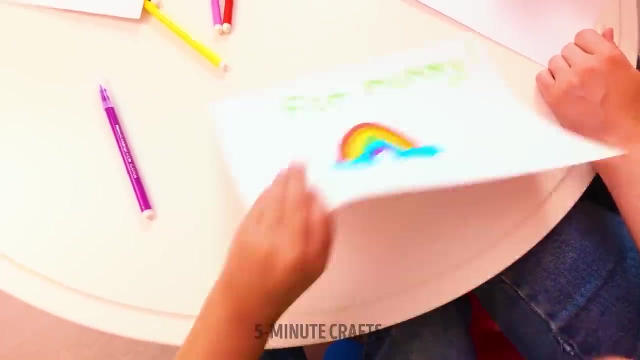 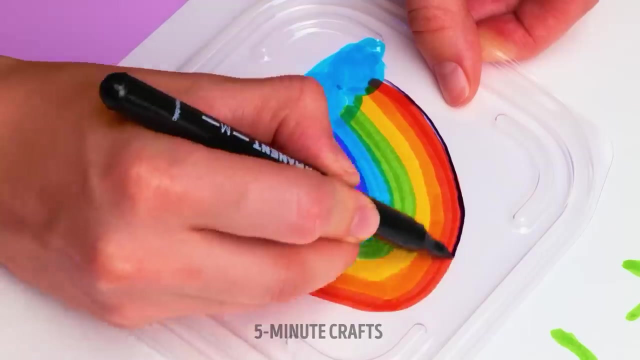 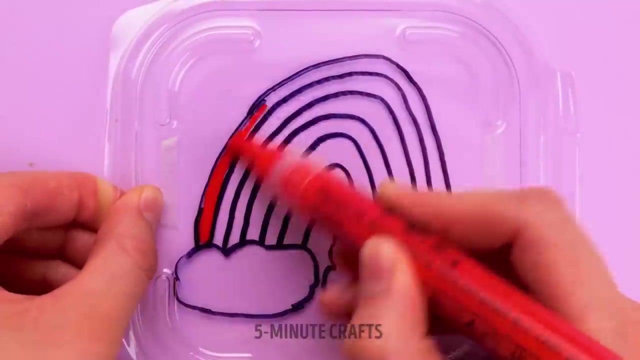 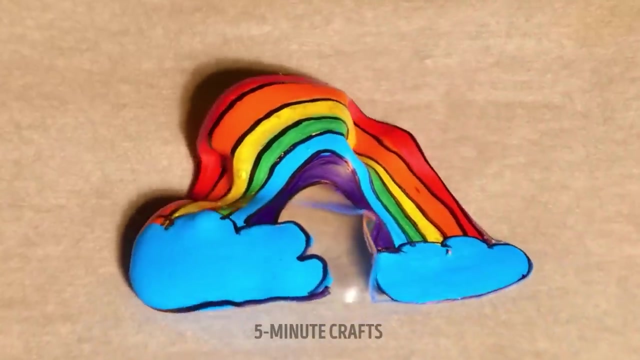 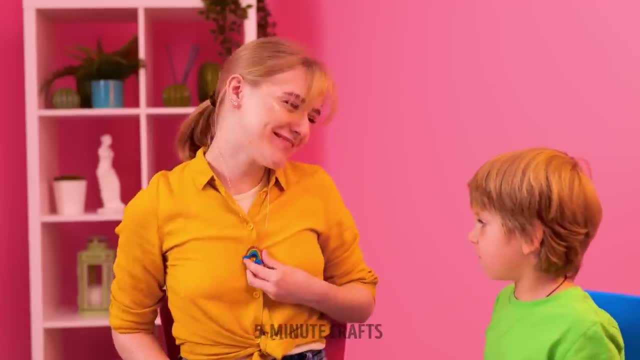 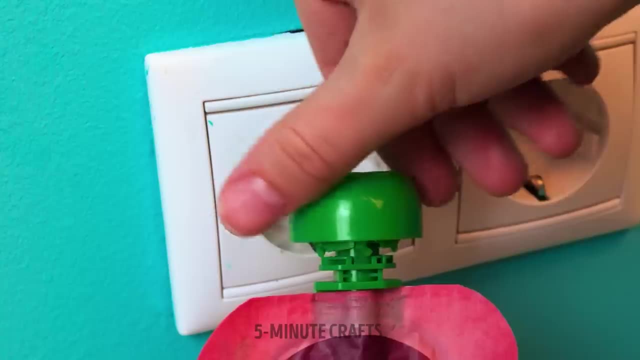 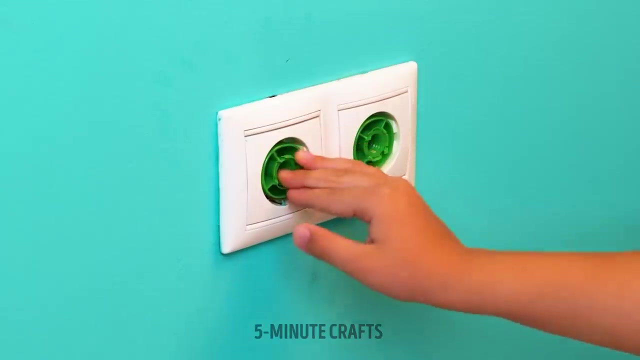 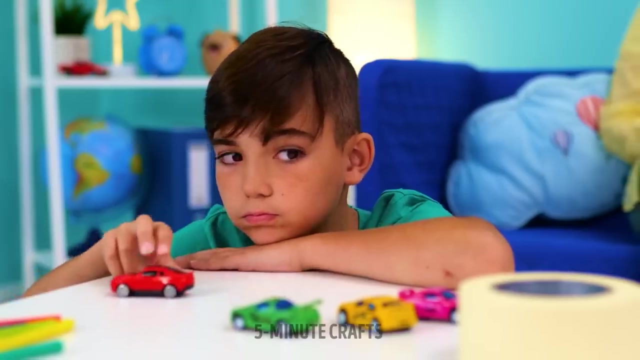 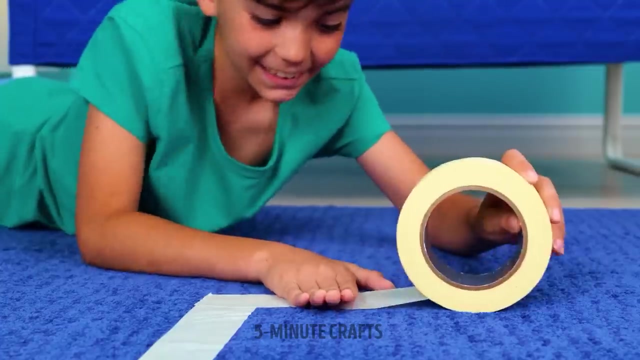 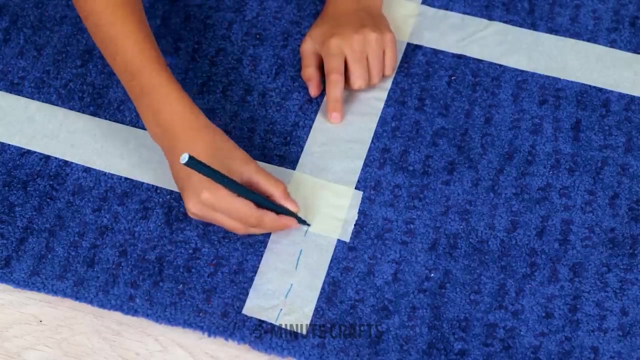 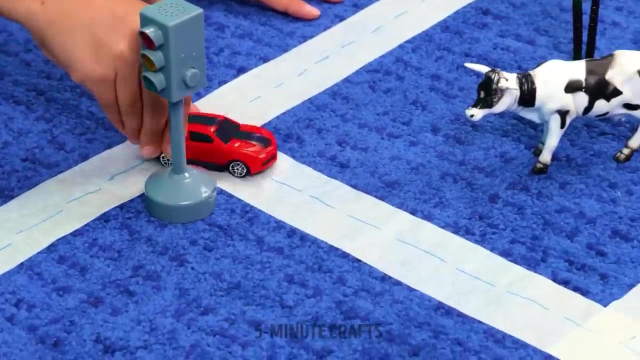 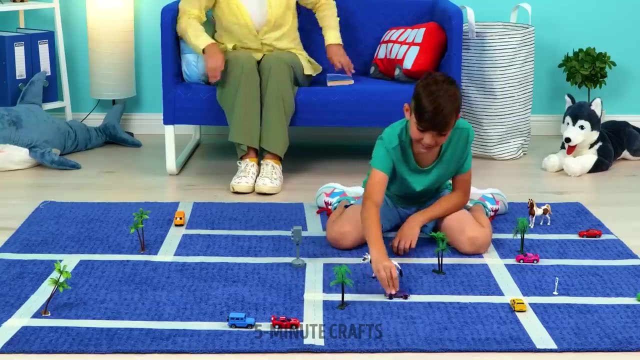 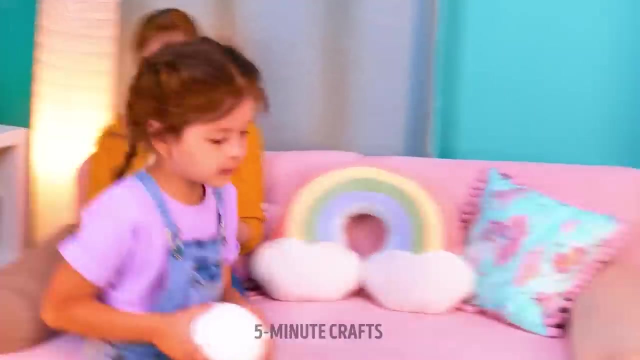 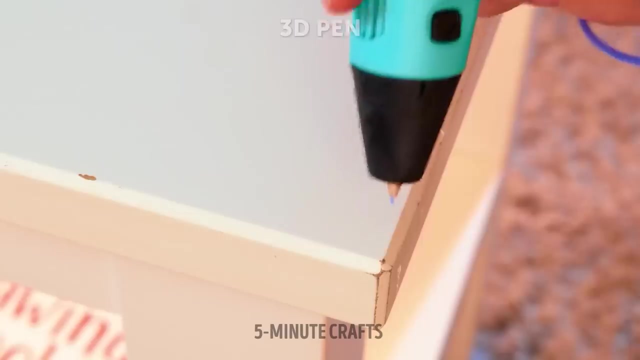 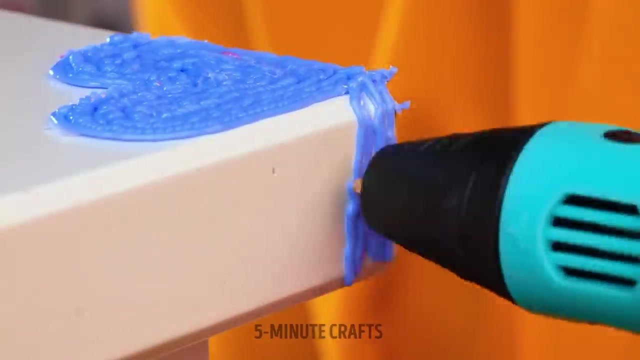 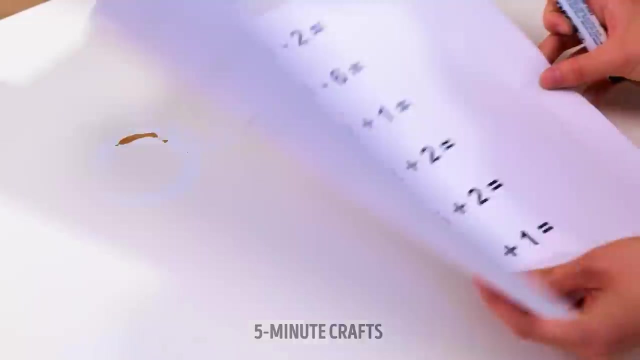 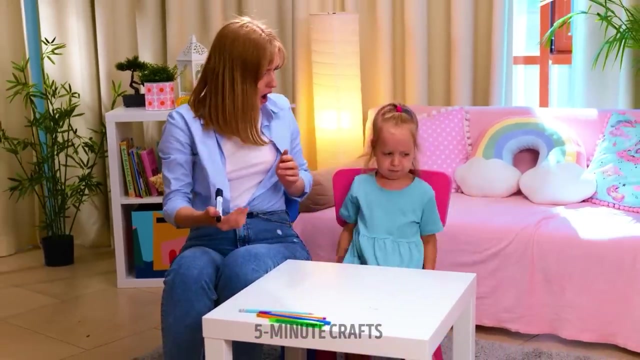 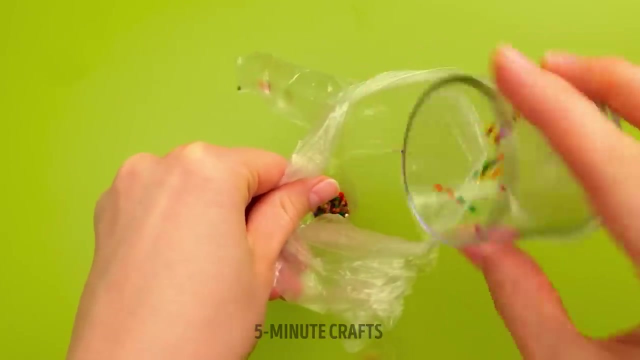 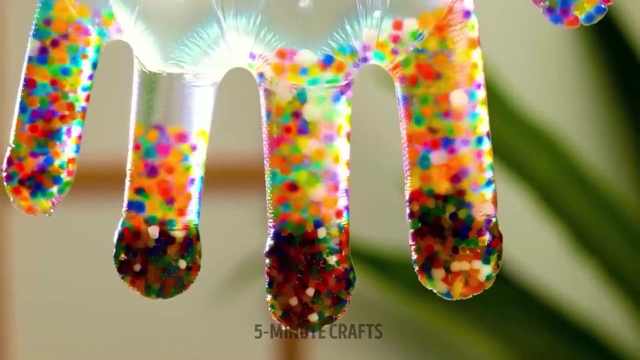 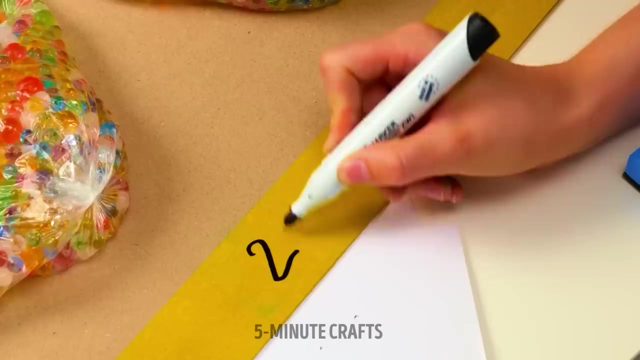 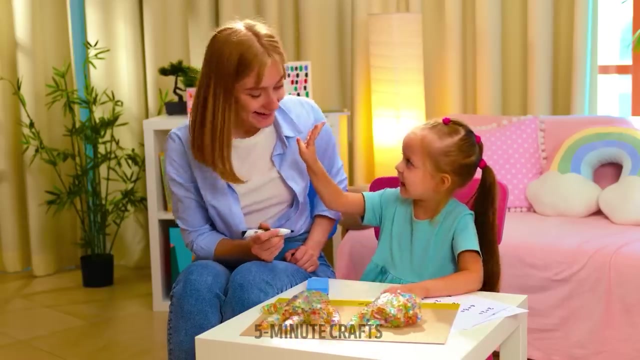 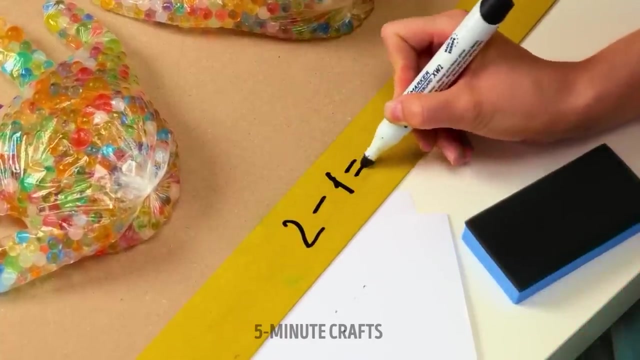 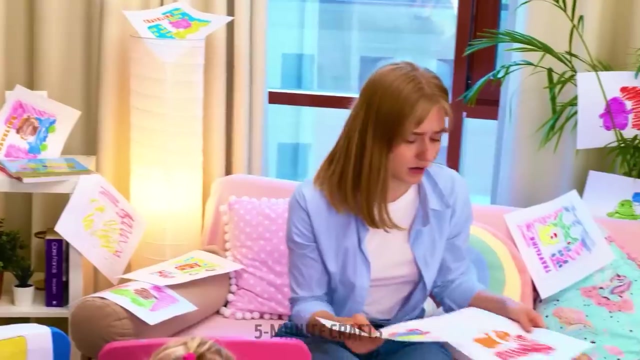 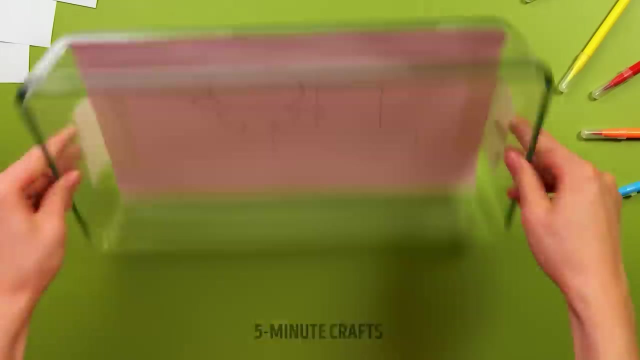 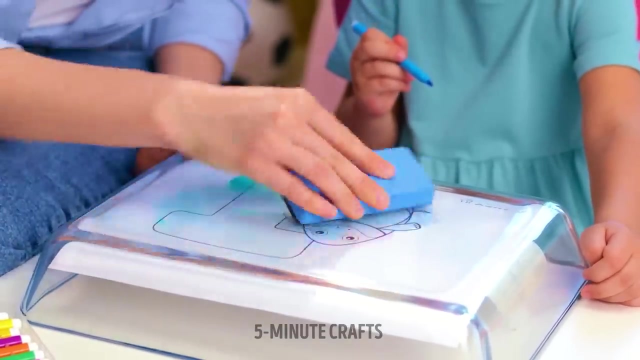 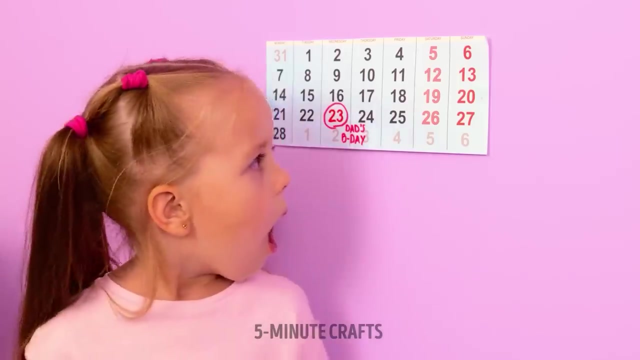 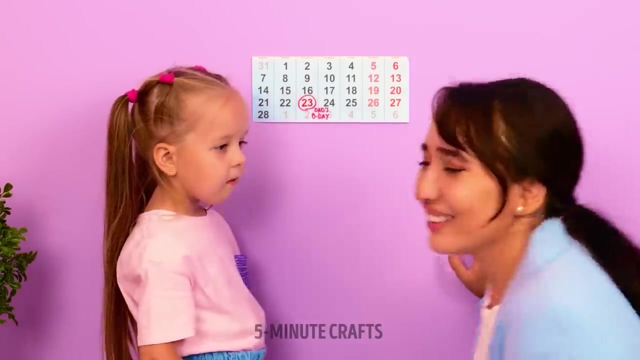 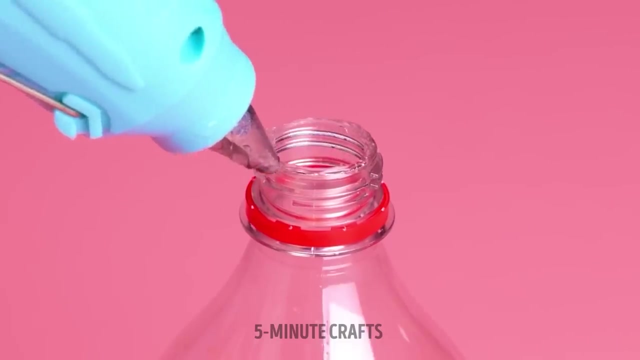 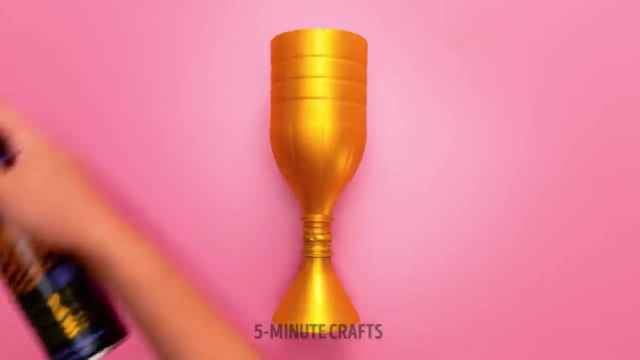 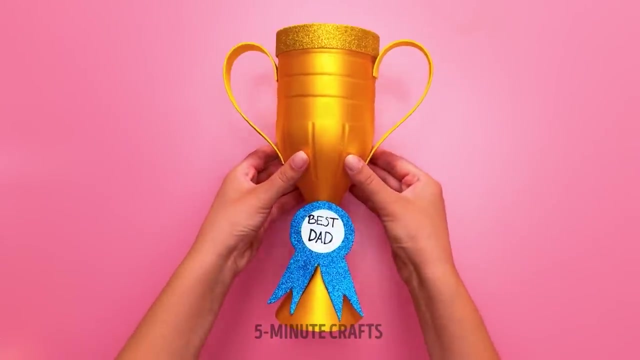 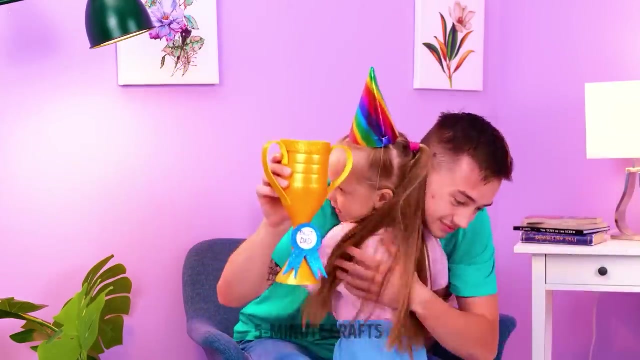 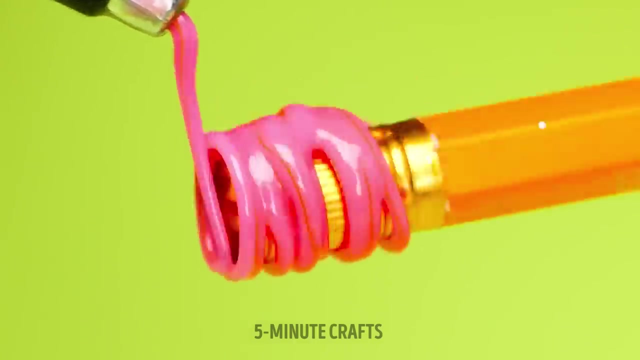 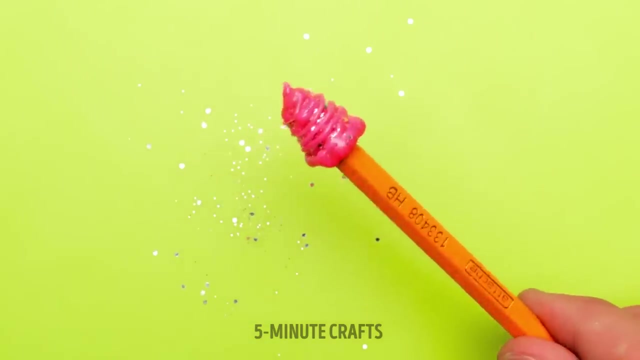 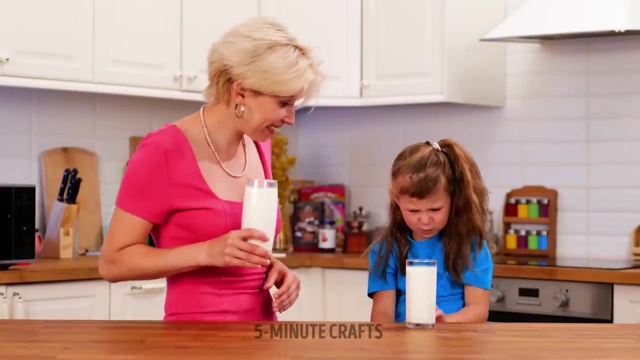 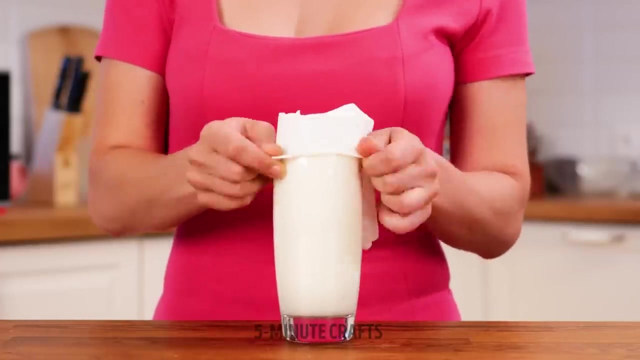 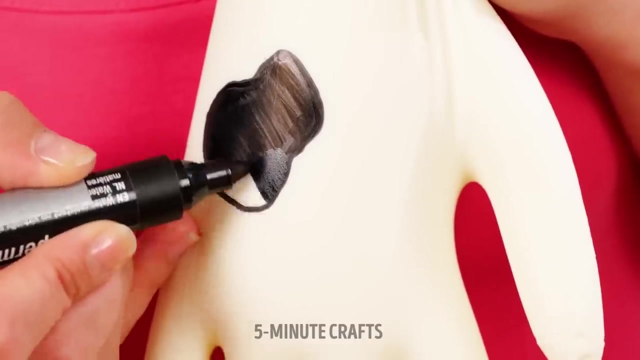 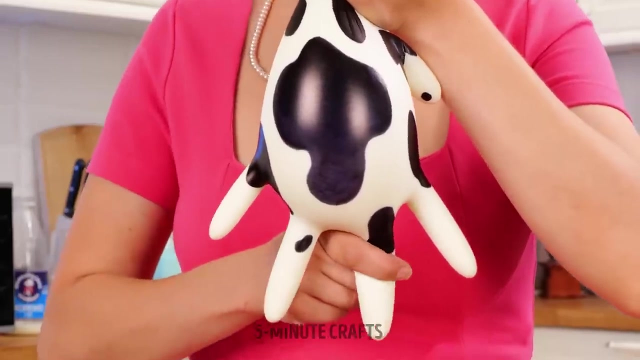 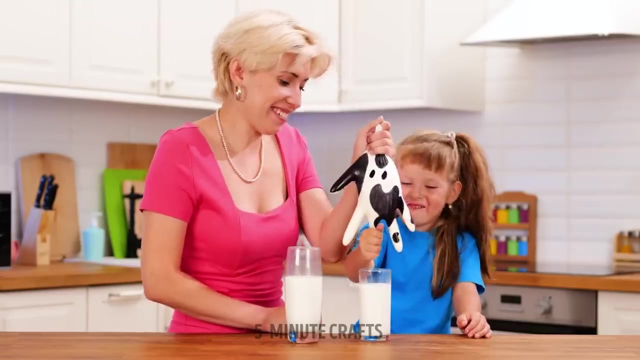 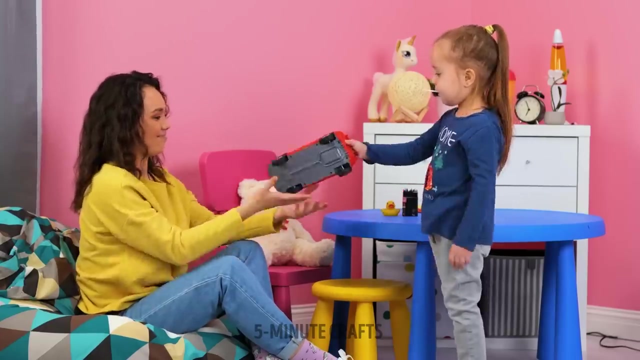 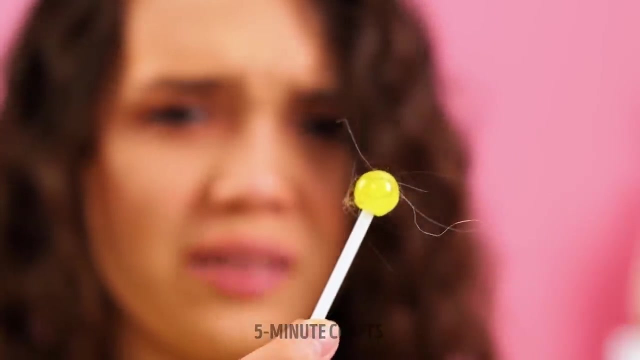 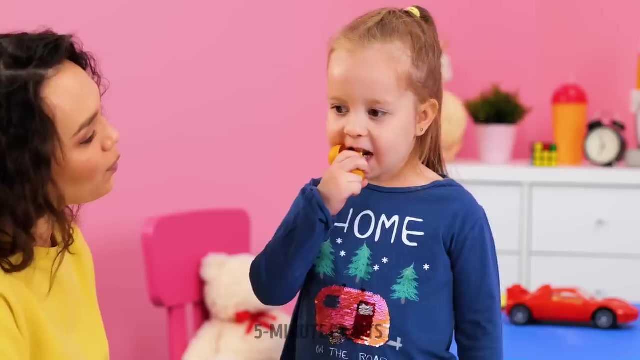 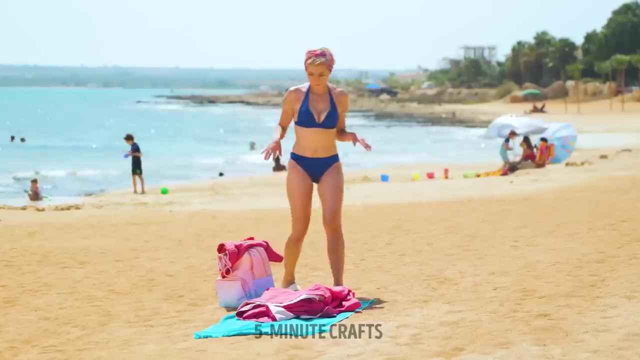 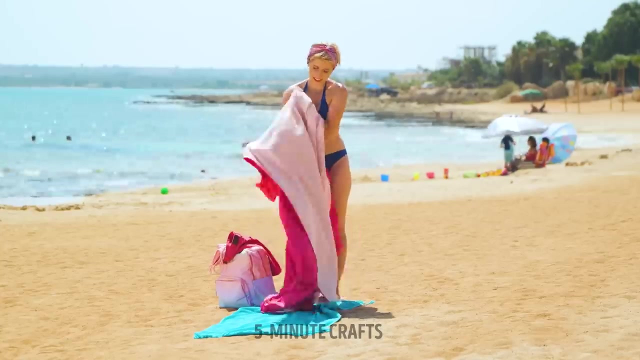 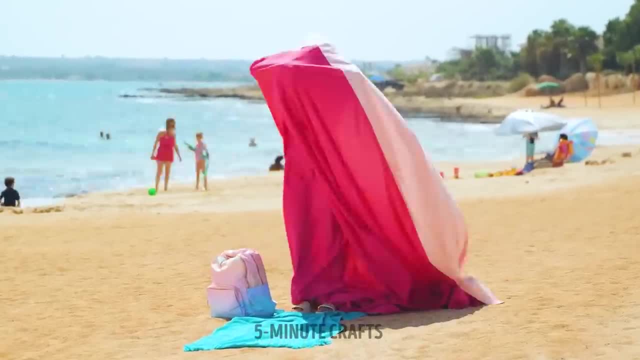 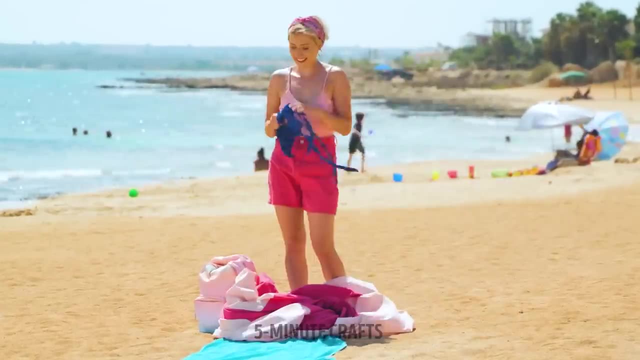 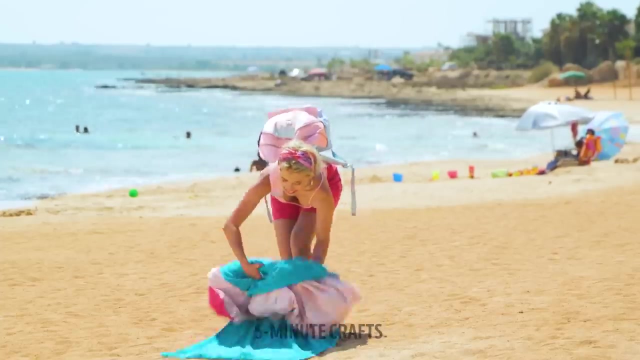 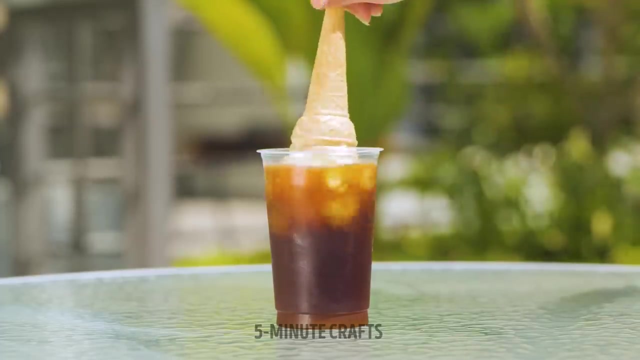 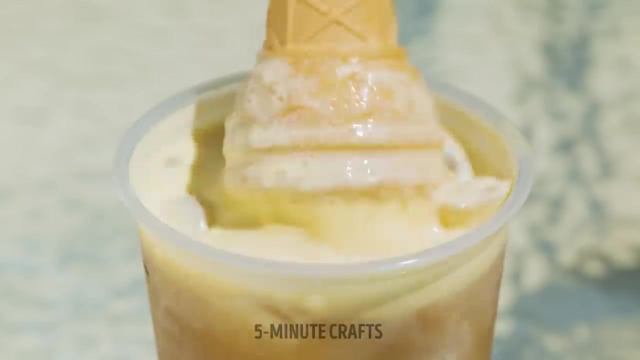 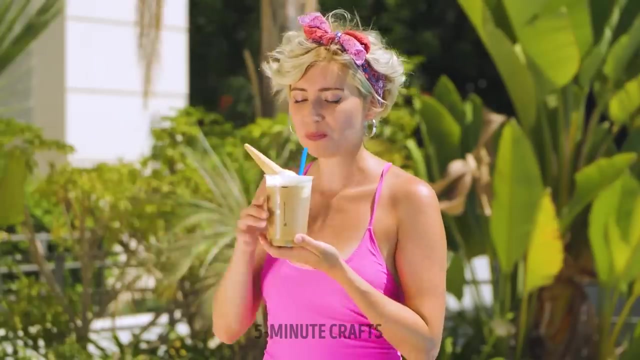 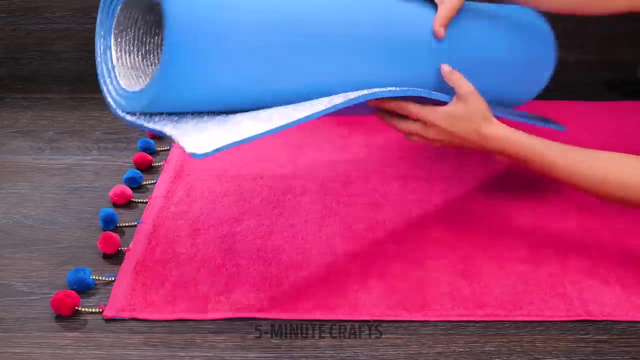 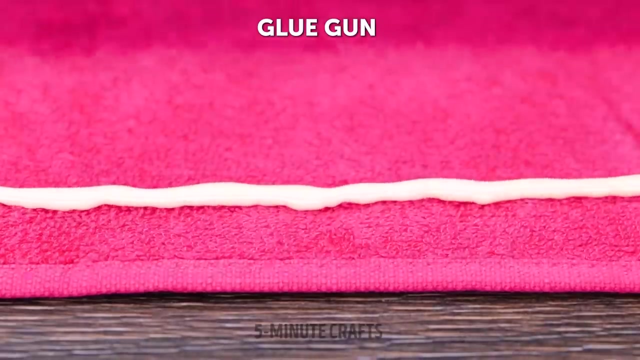 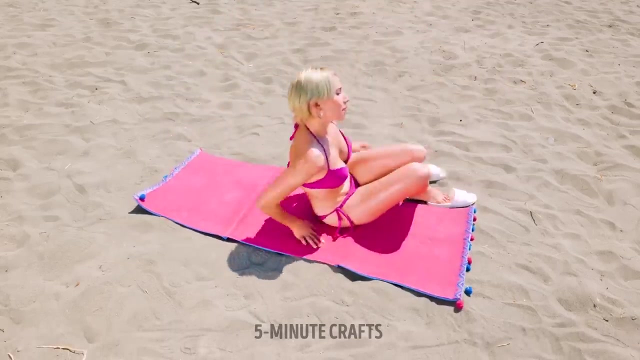 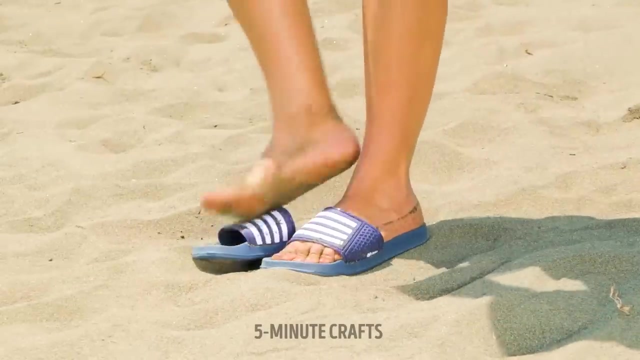 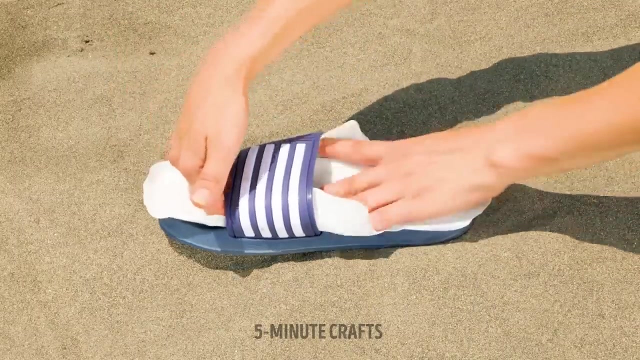 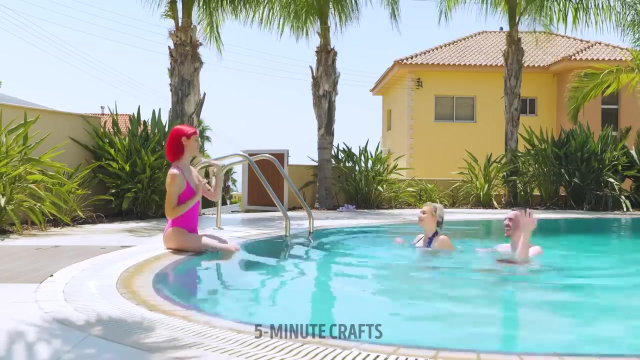 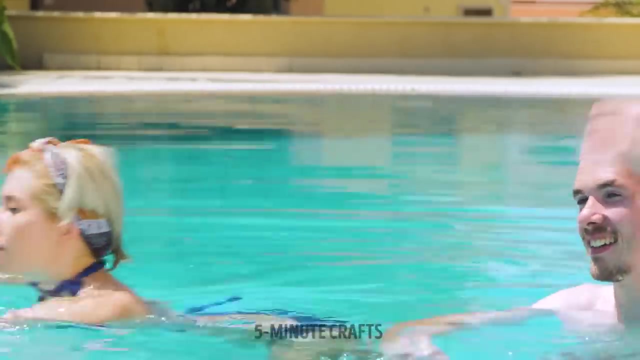 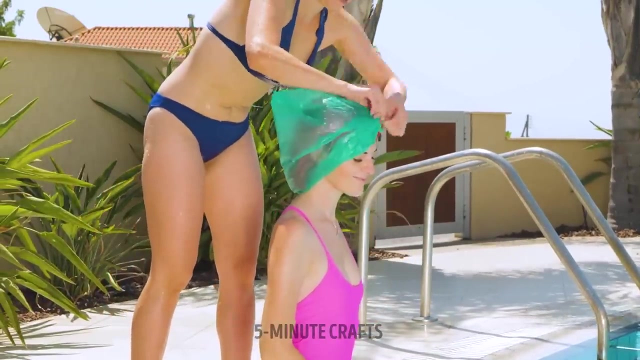 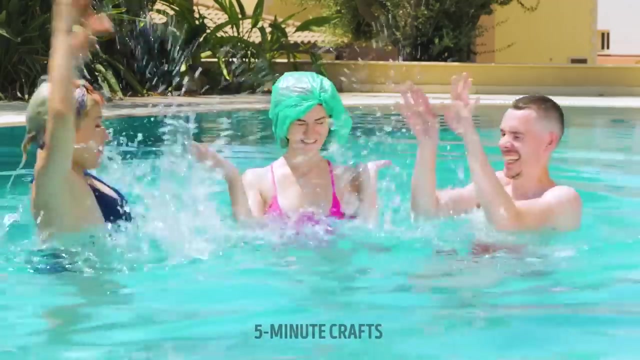 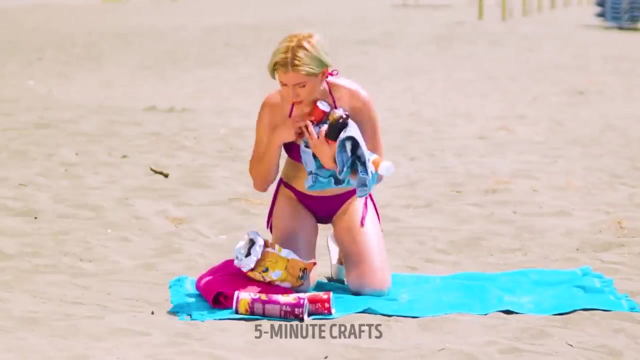 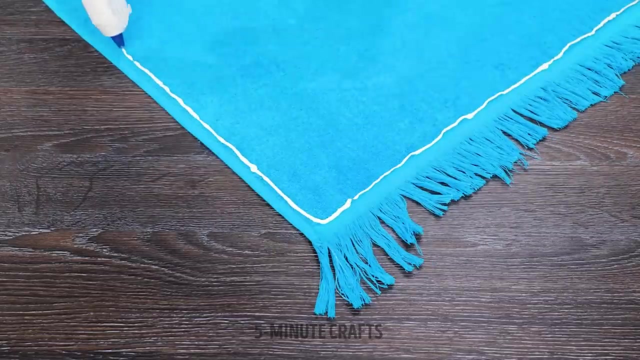 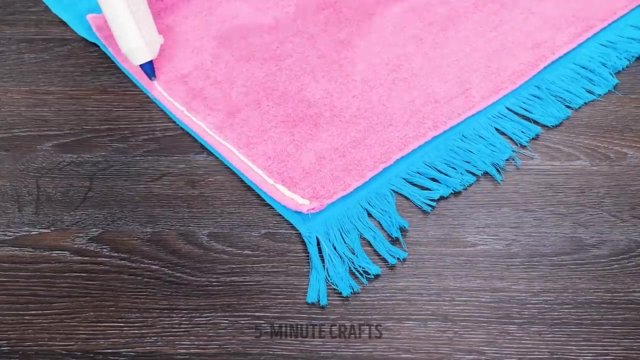 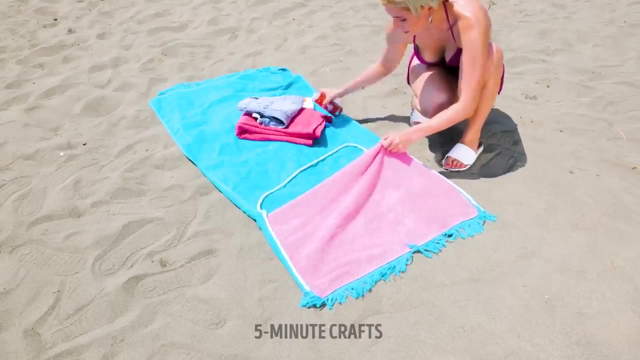 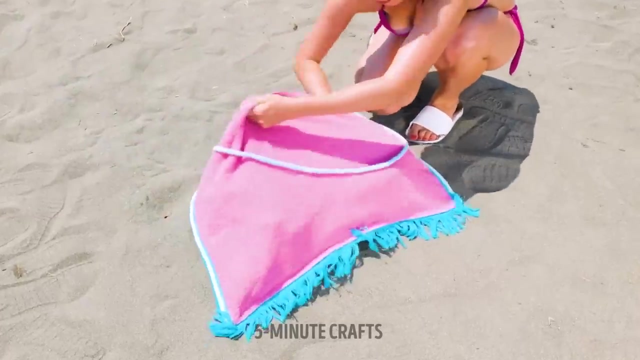 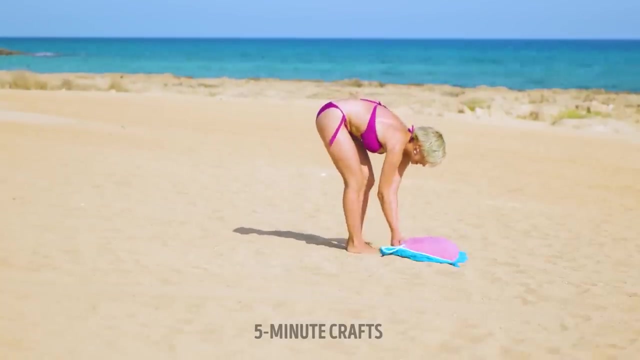 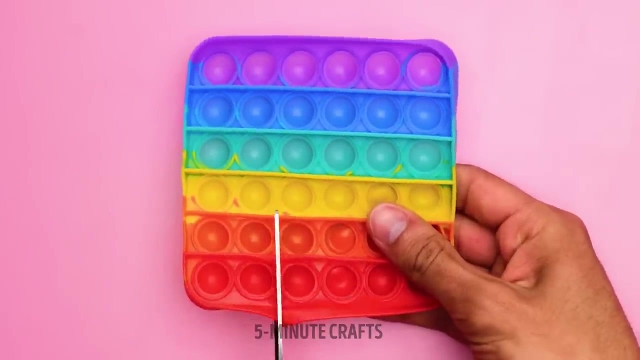 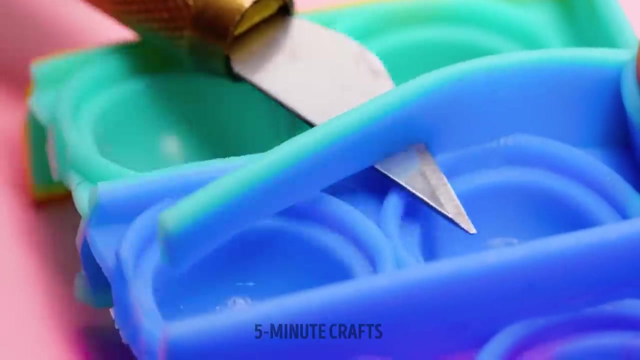 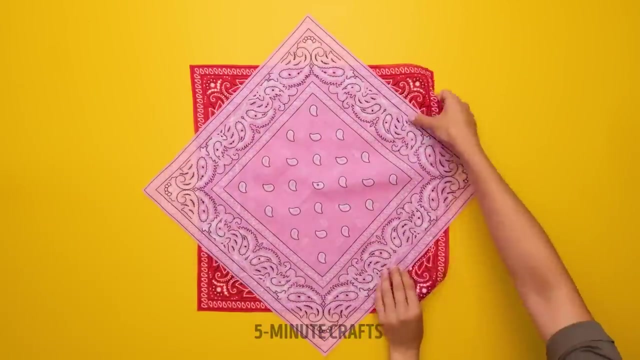 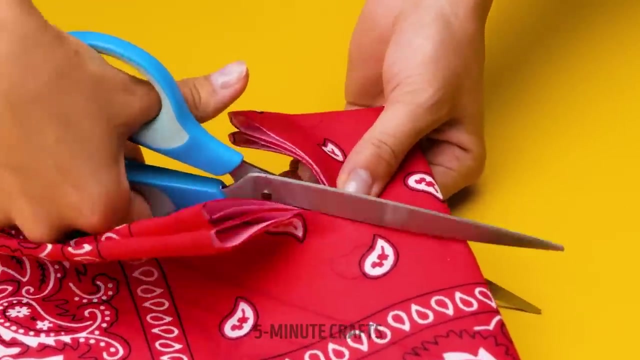 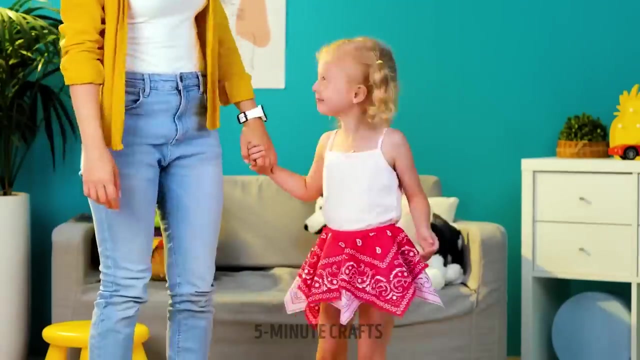 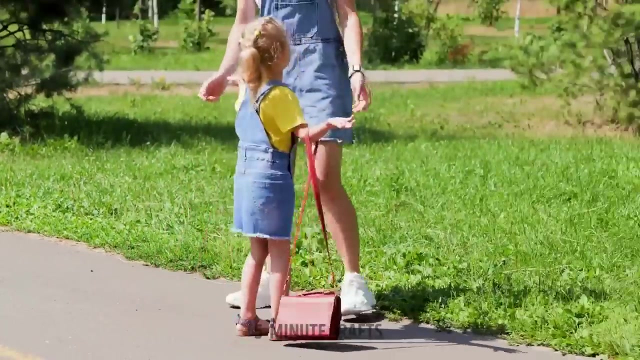 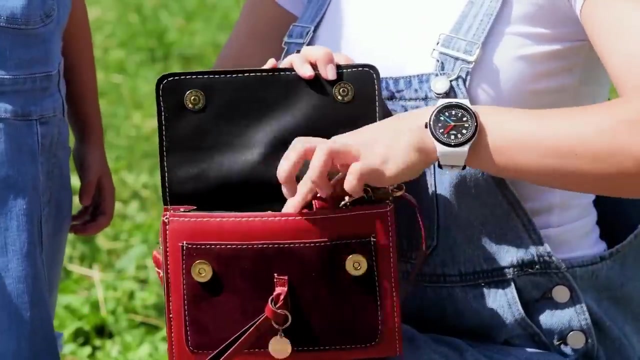 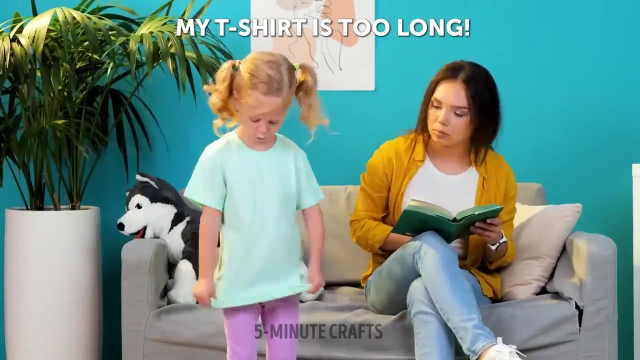 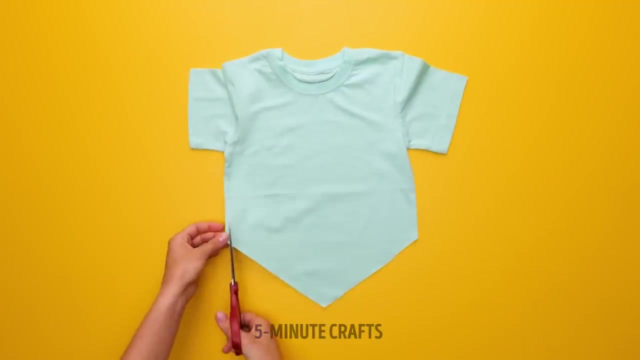 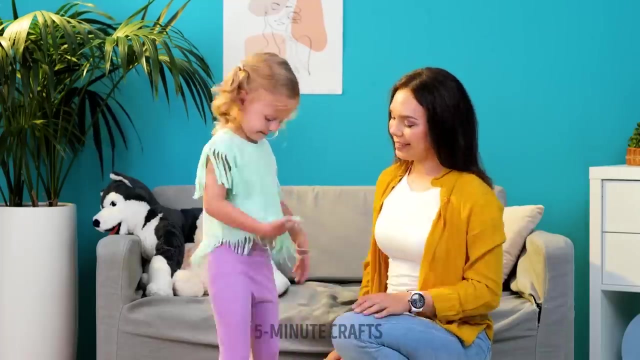 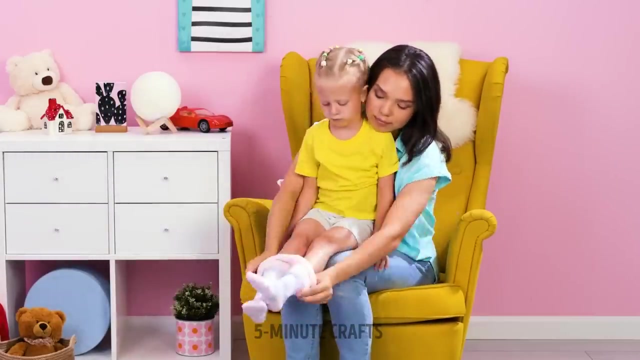 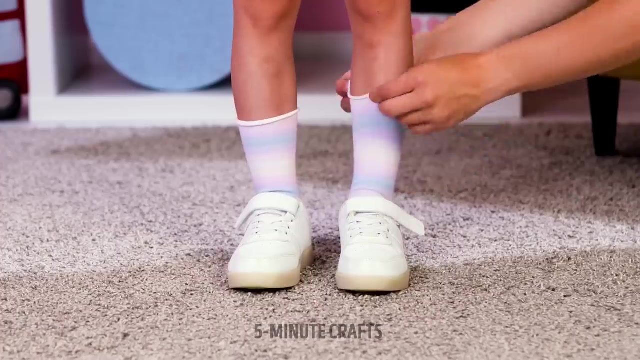 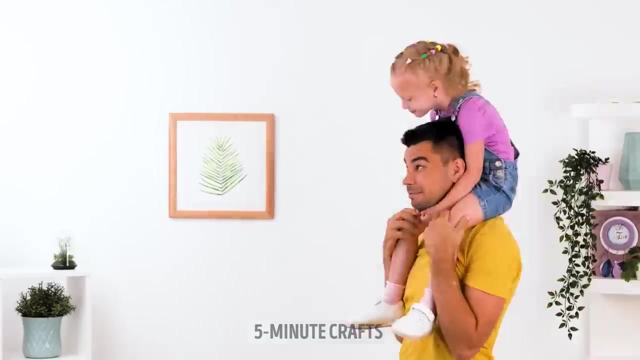 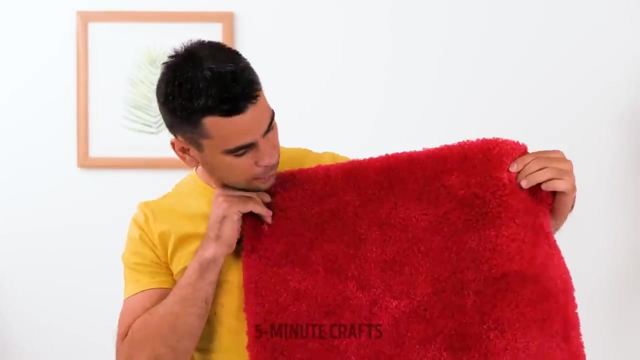 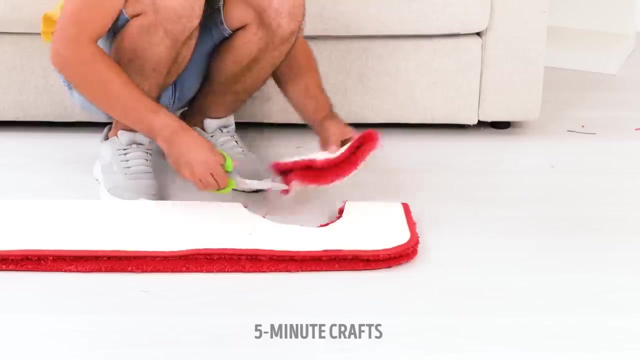 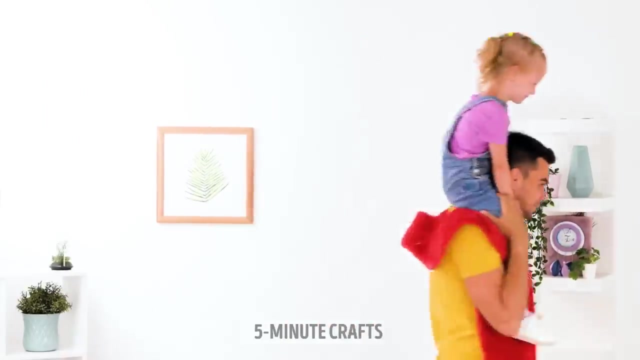 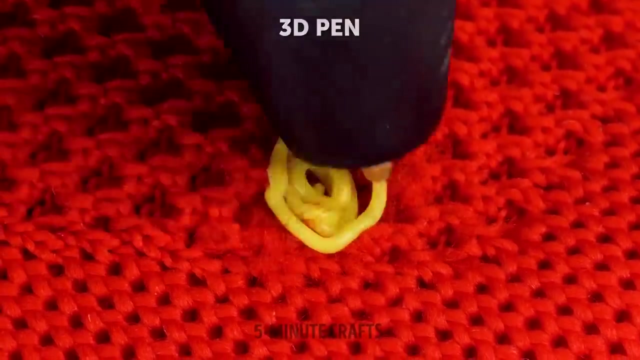 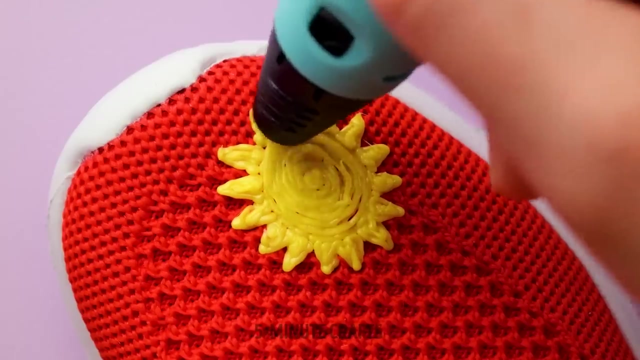 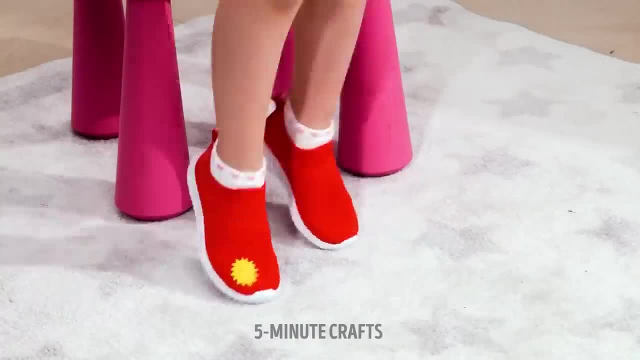 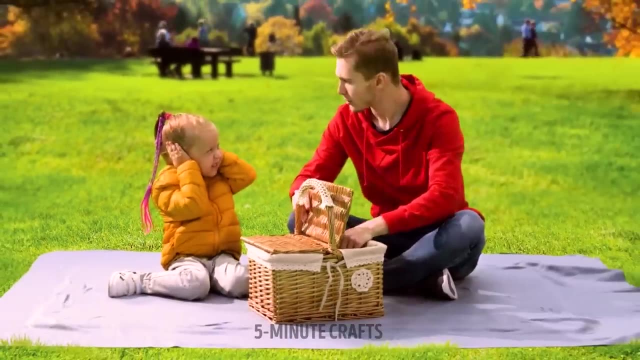 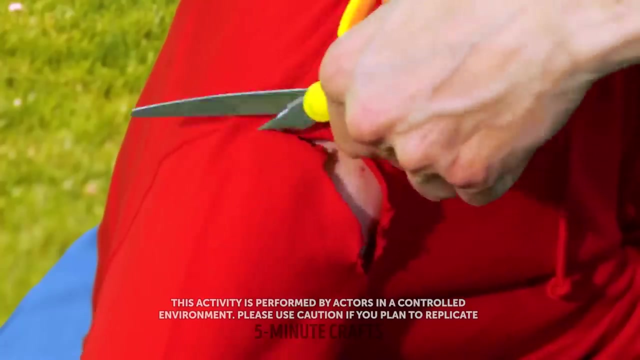 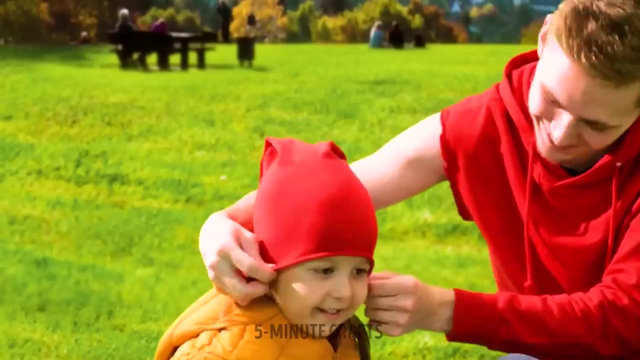 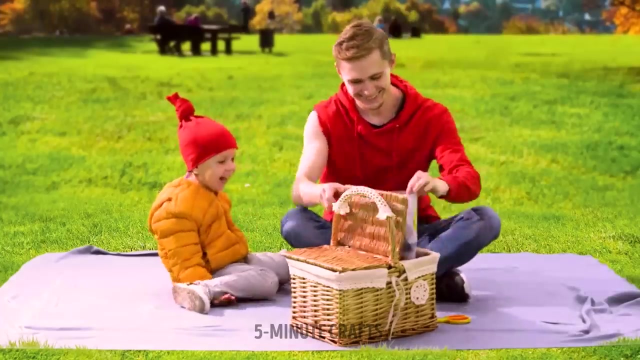 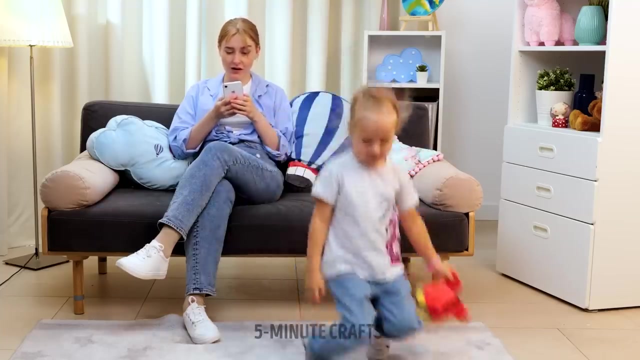 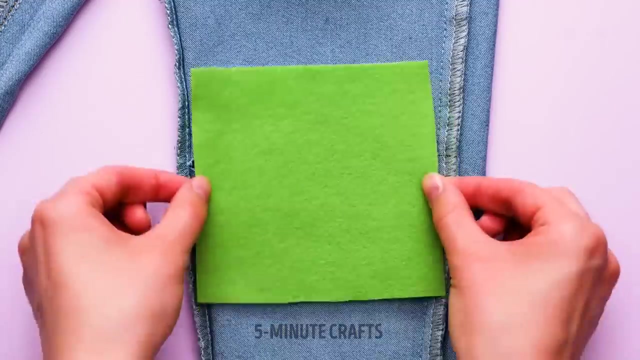 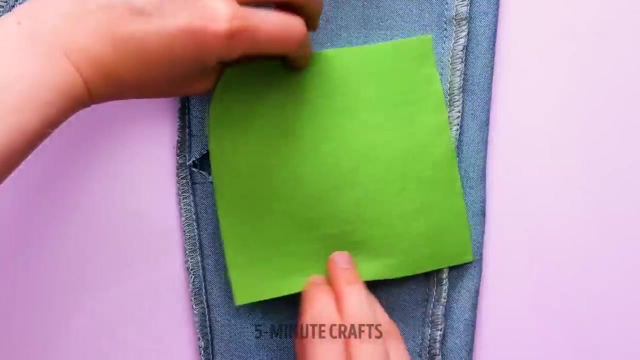 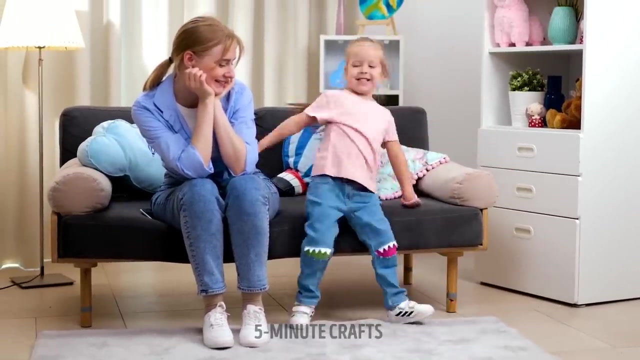 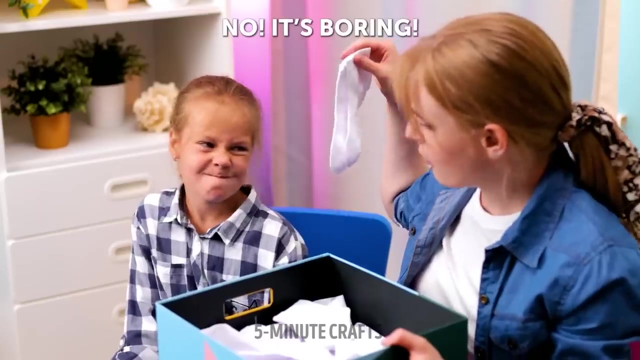 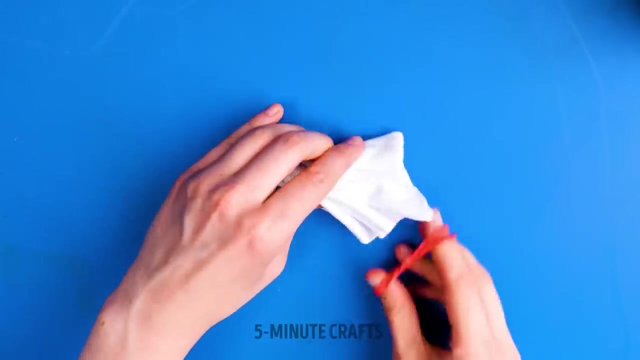 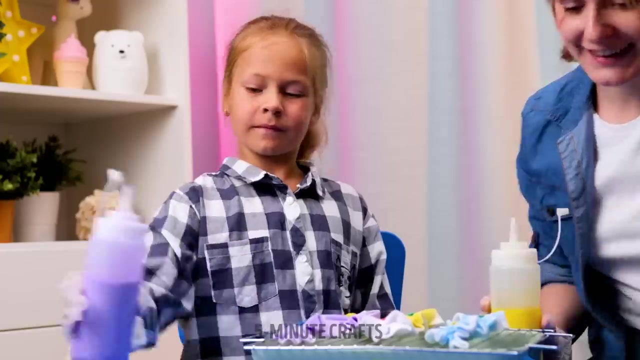 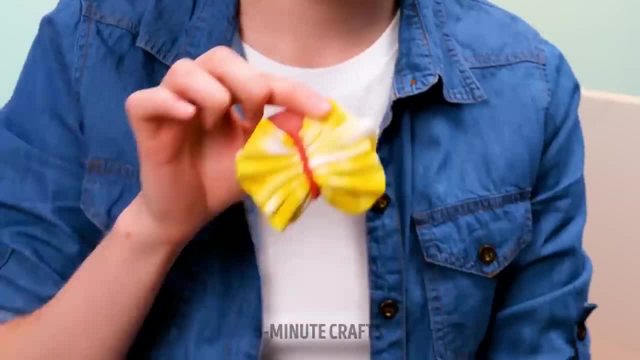 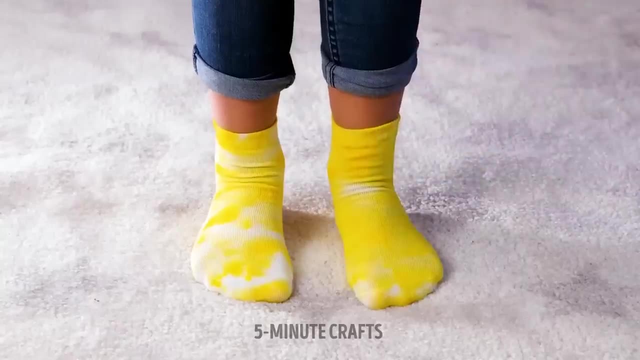 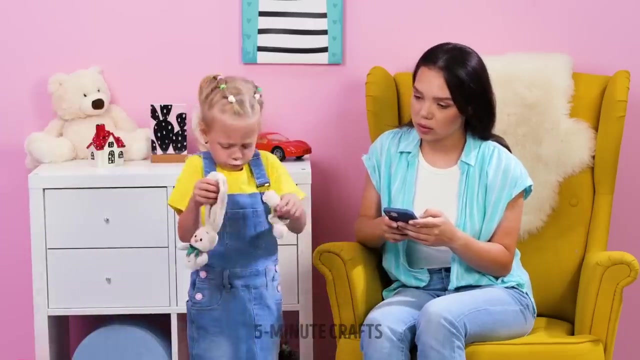 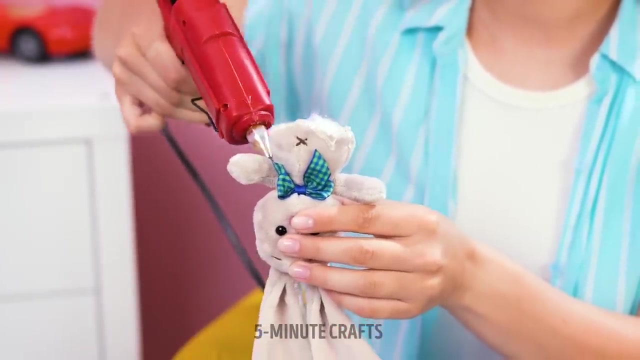 Why would we stop playing those stupid songs? Just close your eyes and you'll be fine. Such a short time in your life, All this hardship and convenience Makes it hard to make sense. Are we missing out? Are we missing out- And I know it's just a matter of time. 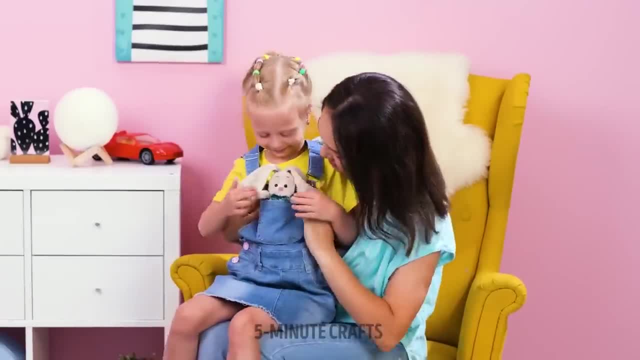 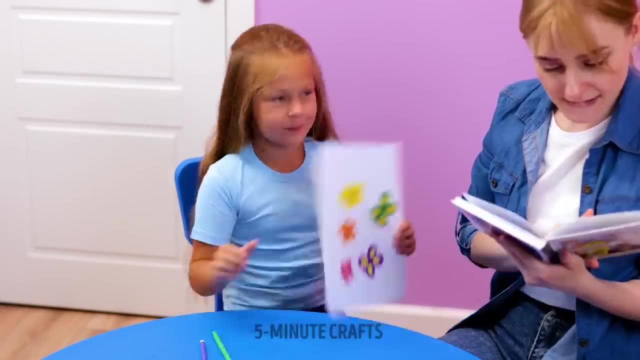 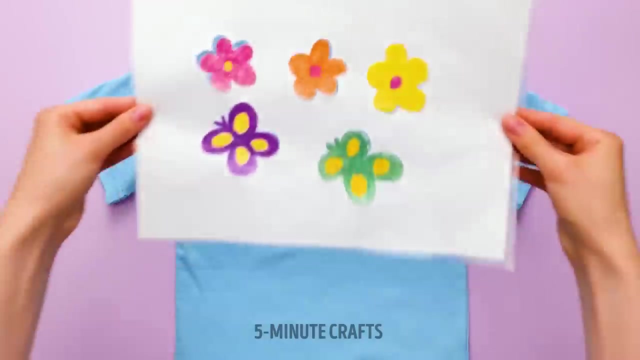 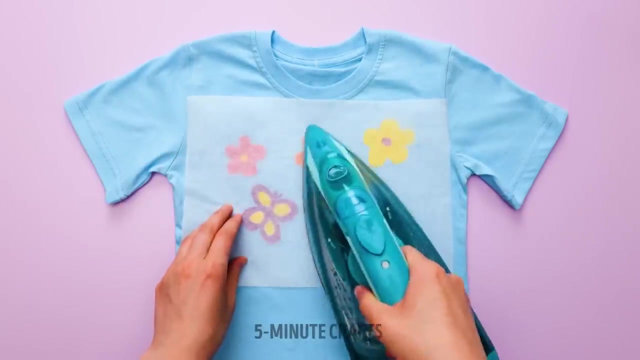 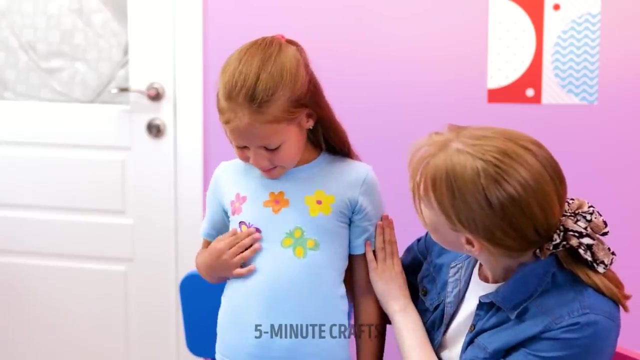 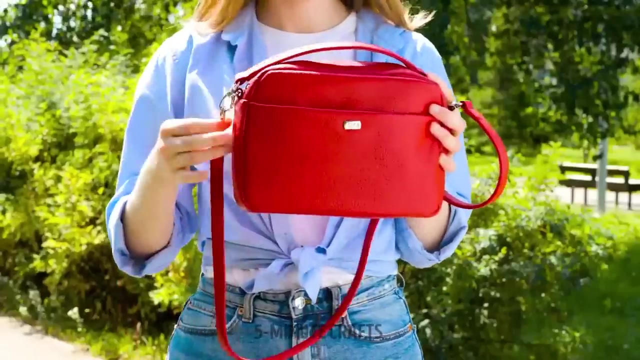 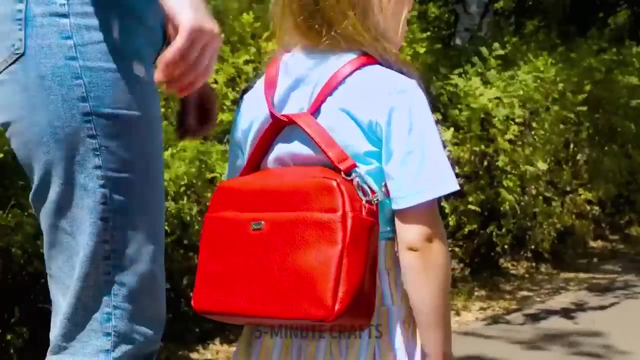 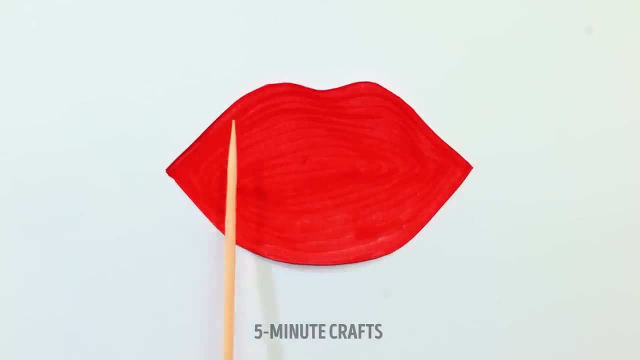 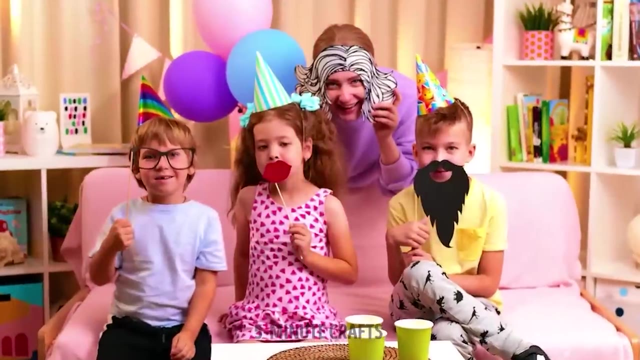 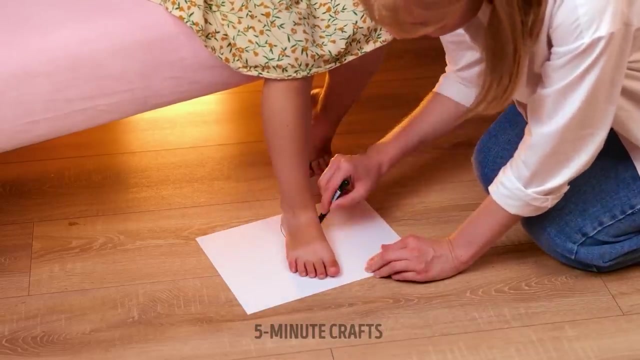 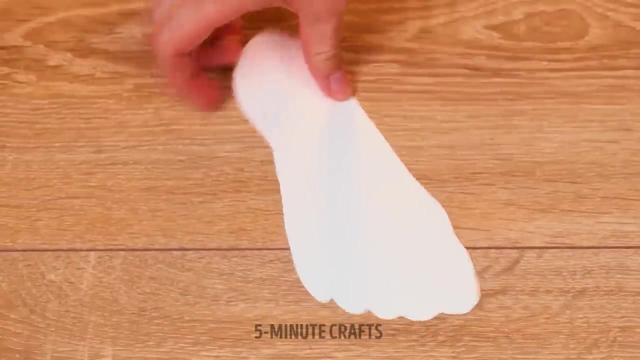 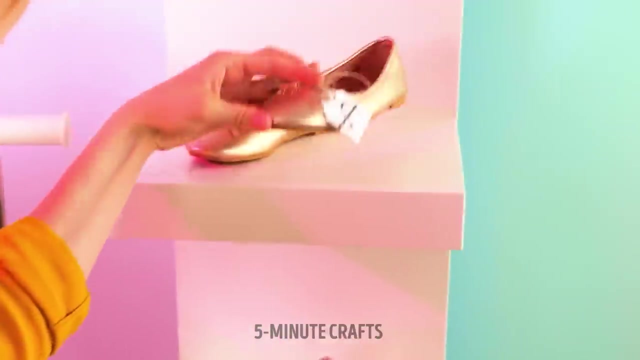 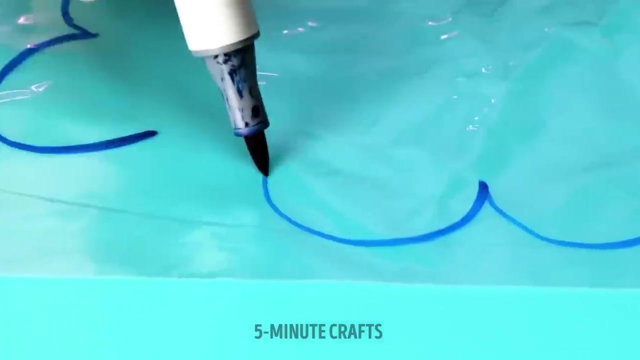 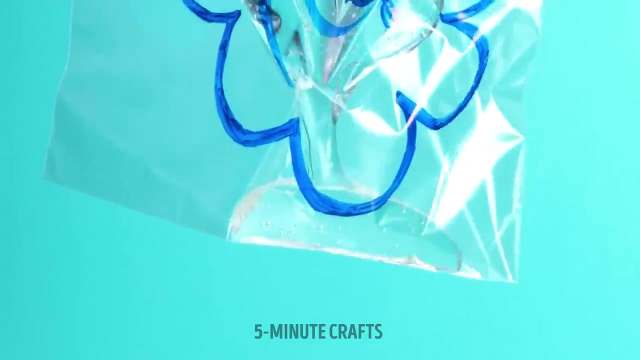 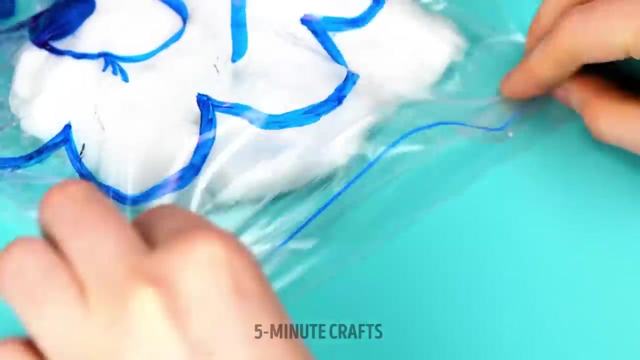 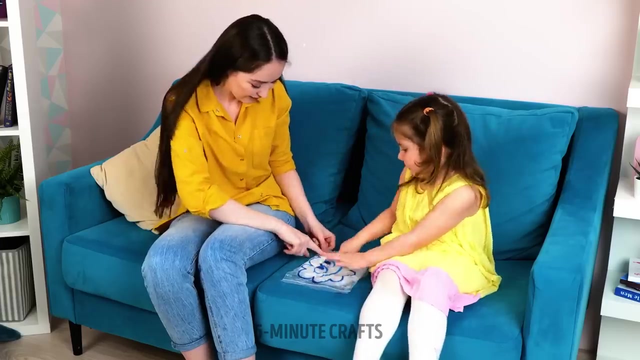 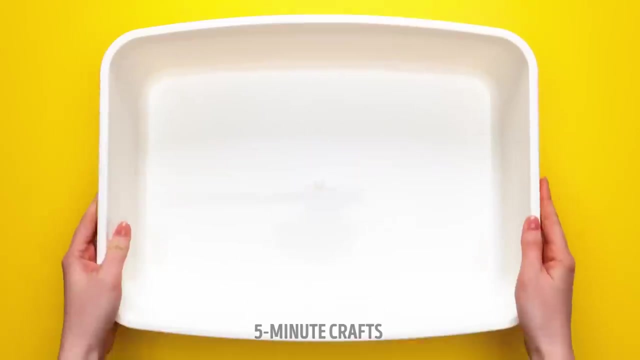 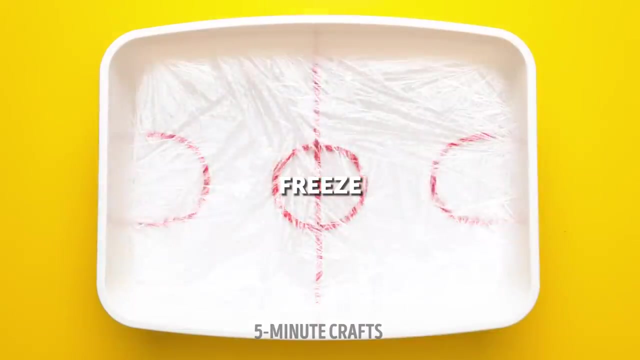 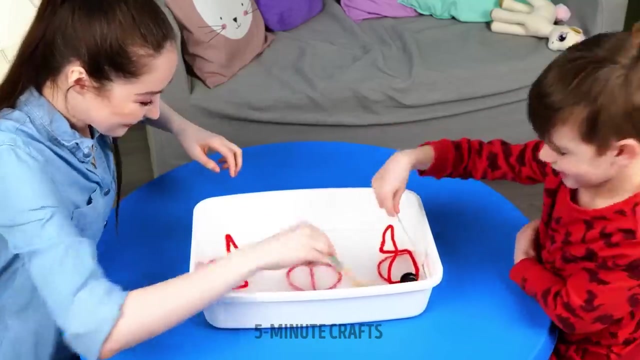 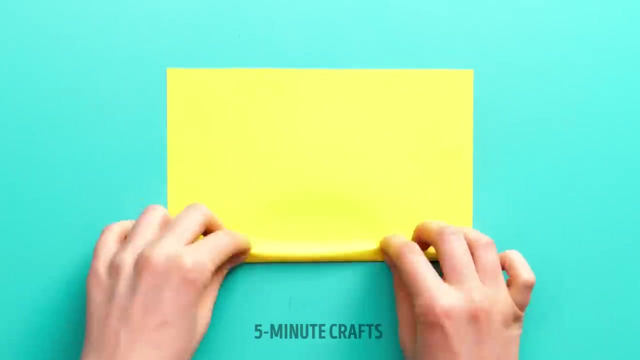 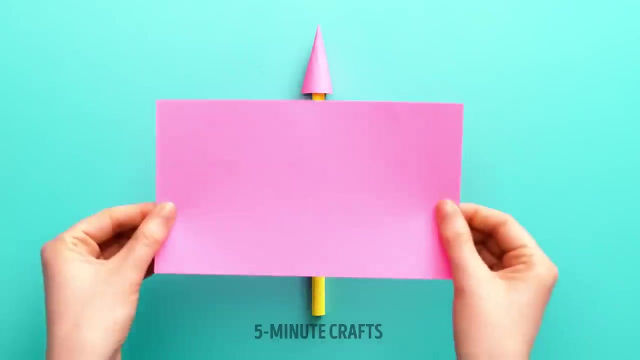 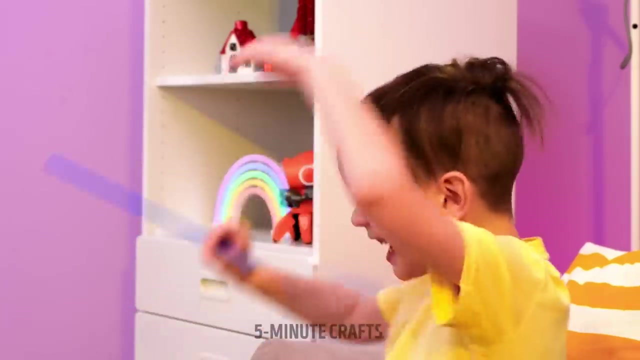 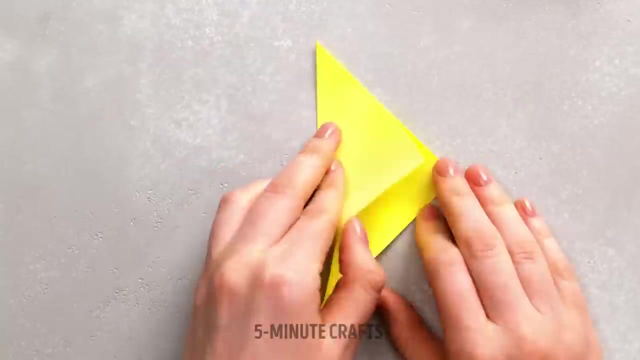 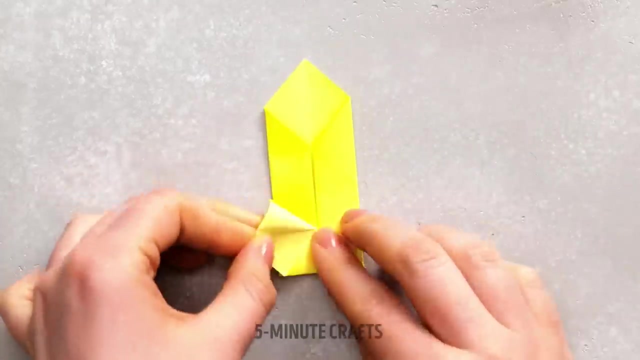 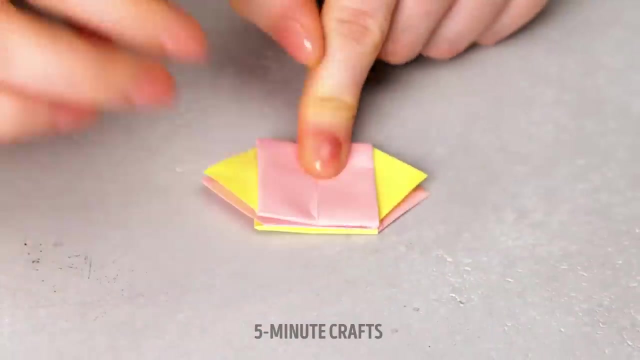 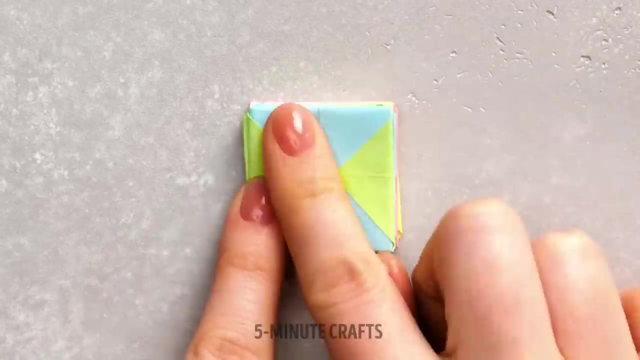 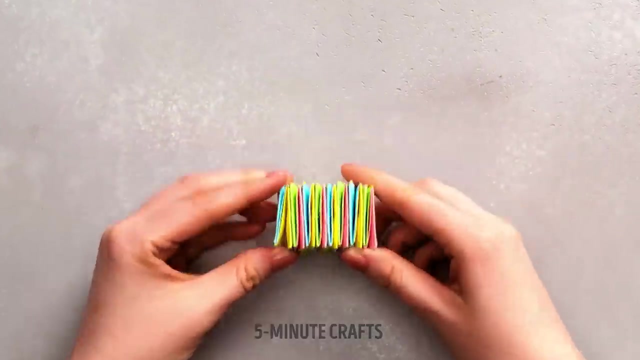 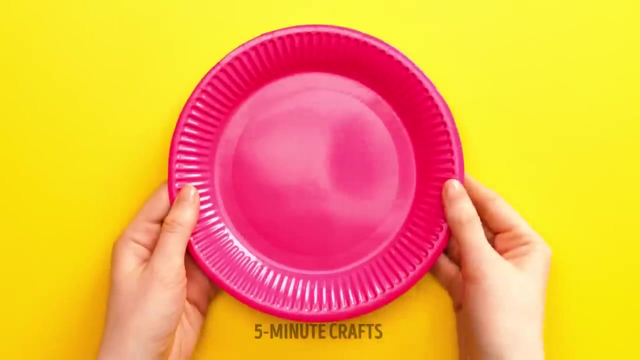 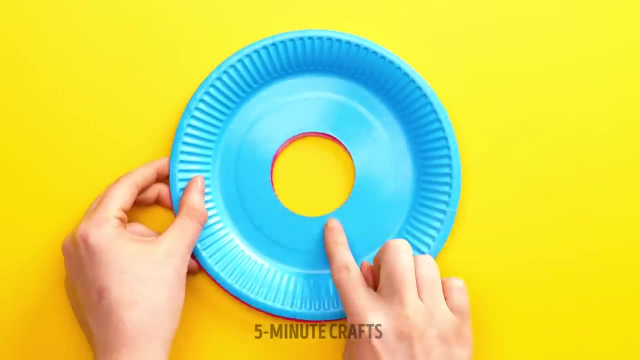 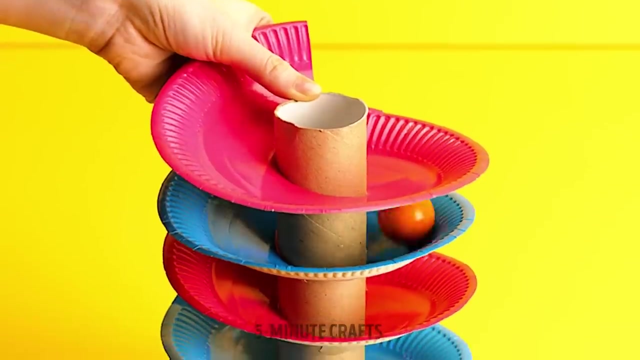 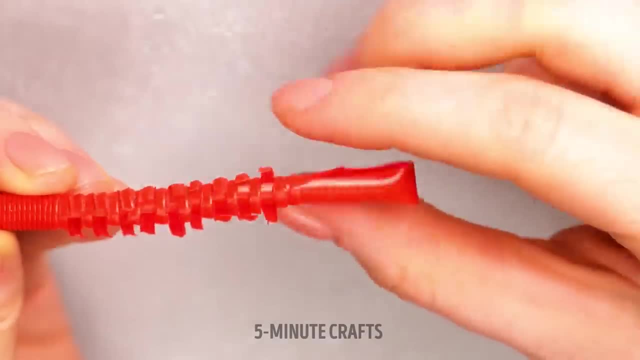 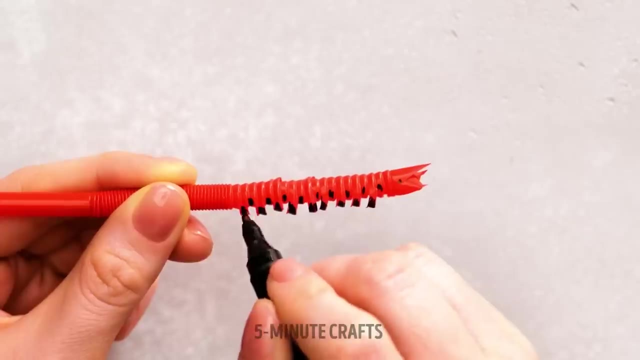 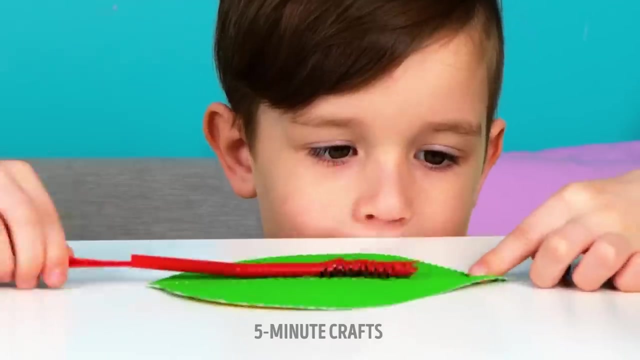 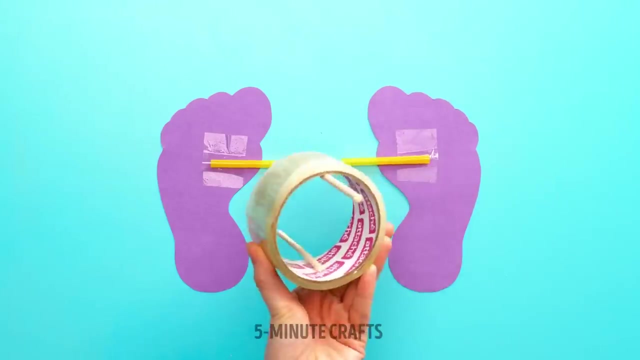 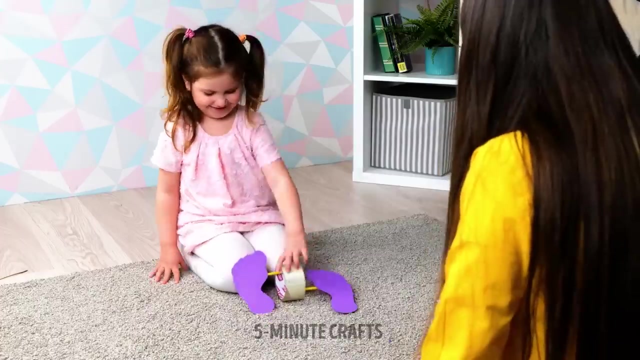 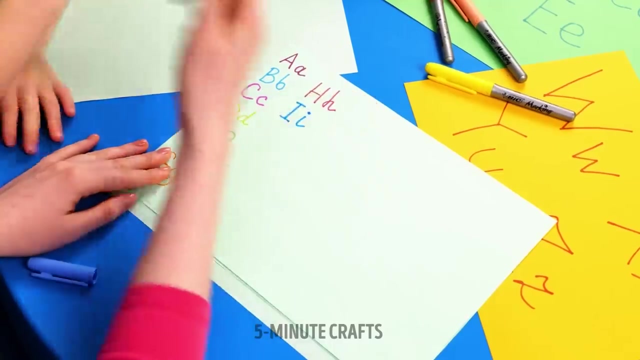 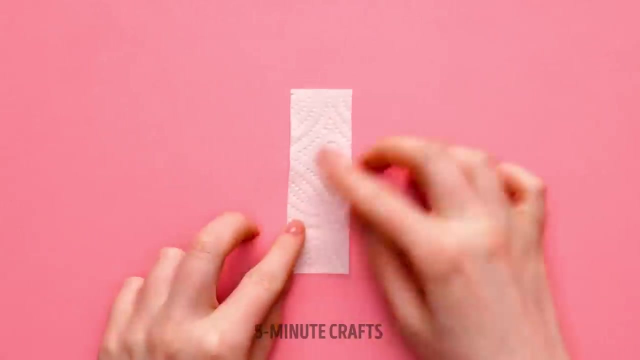 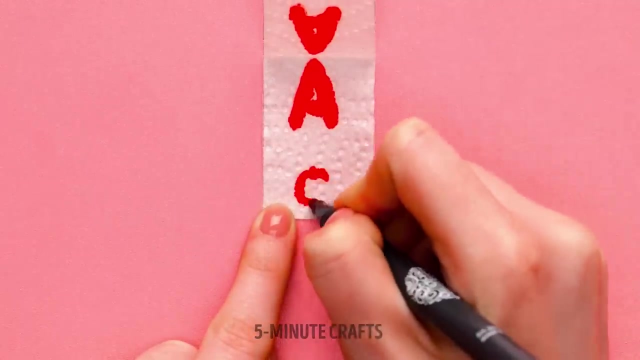 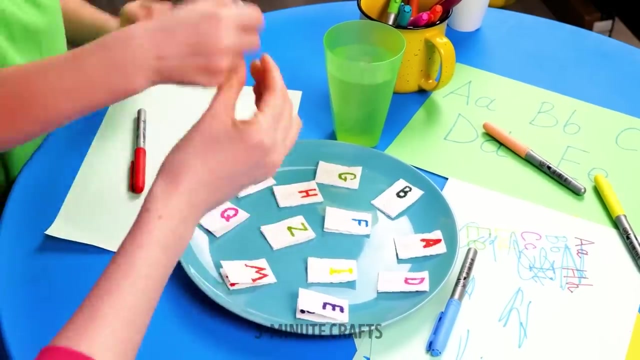 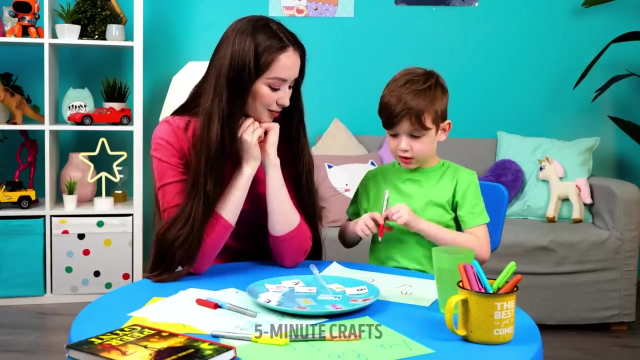 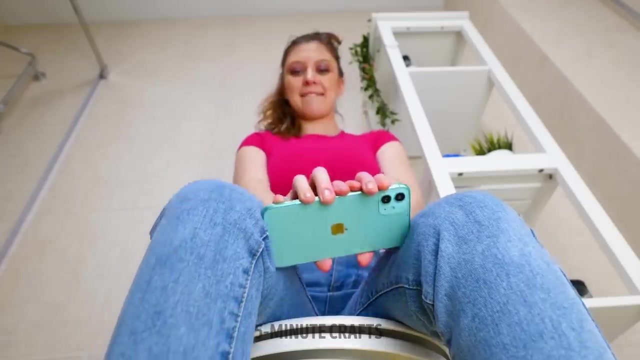 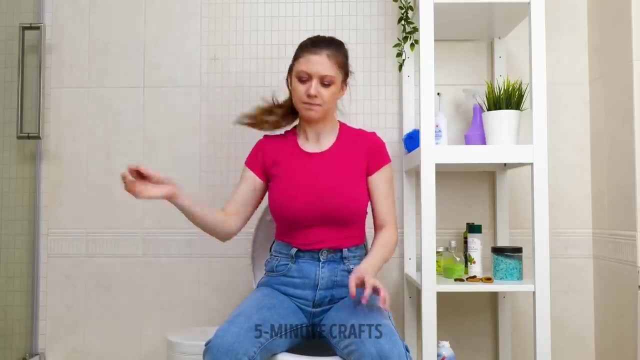 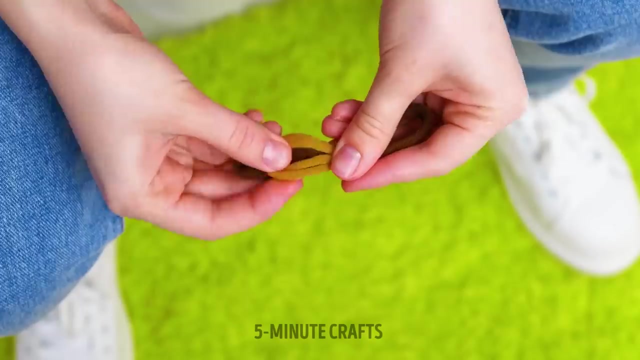 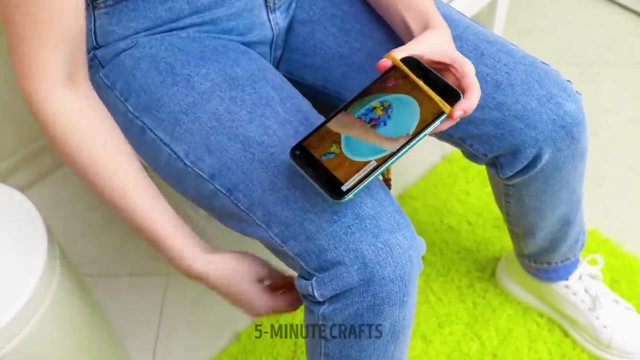 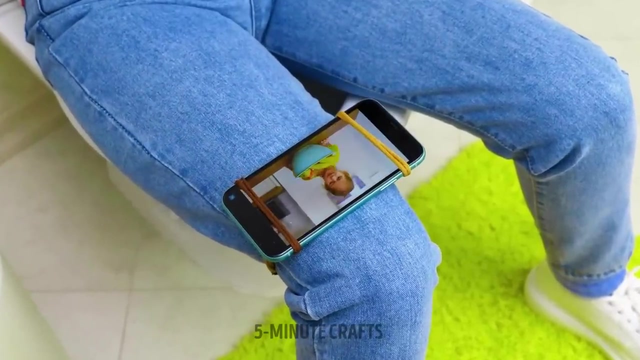 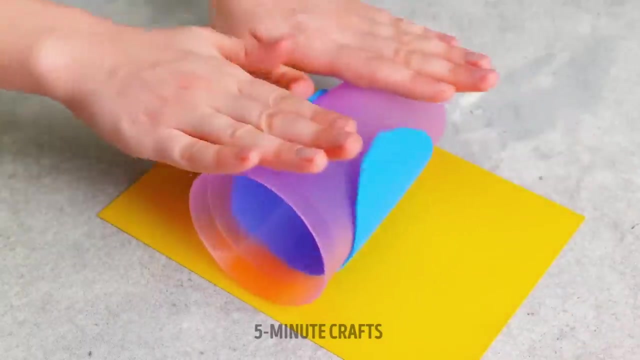 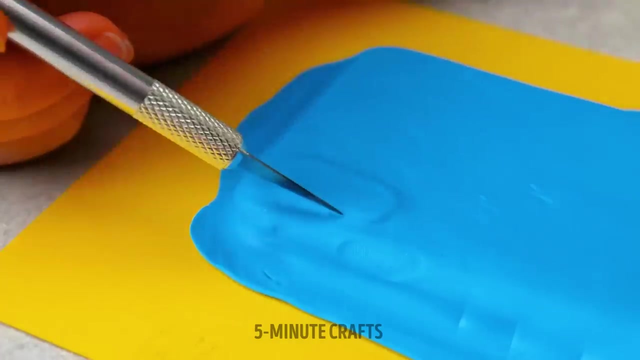 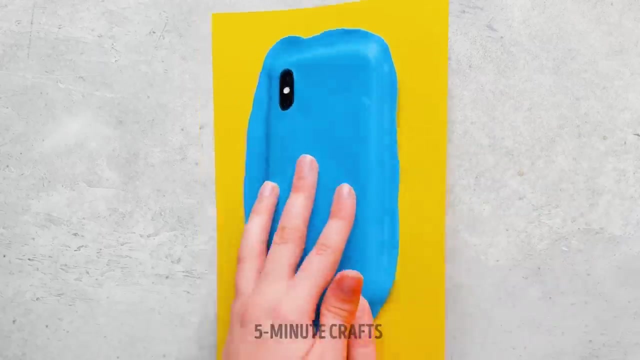 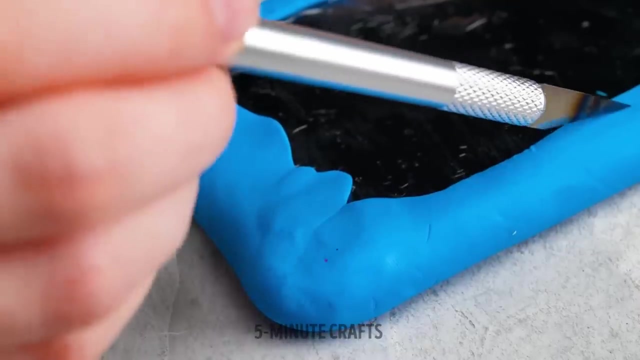 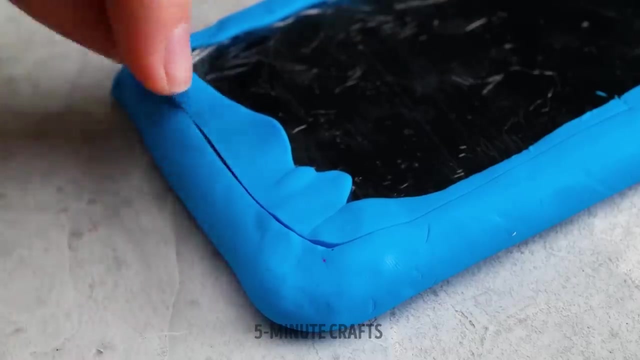 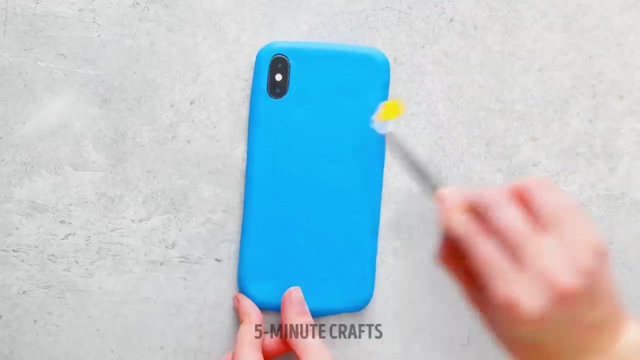 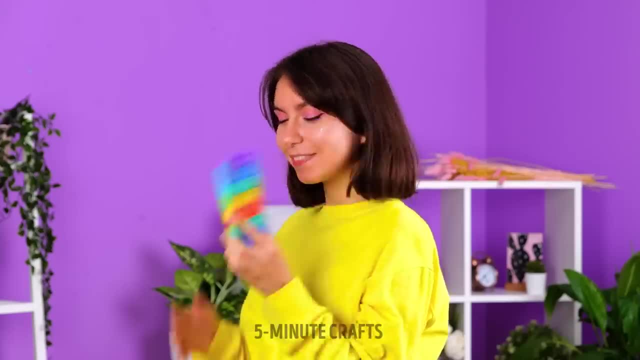 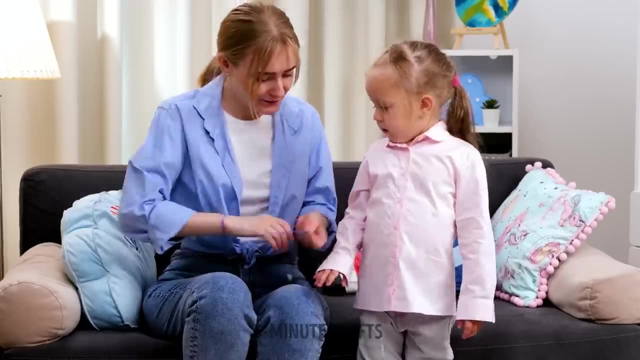 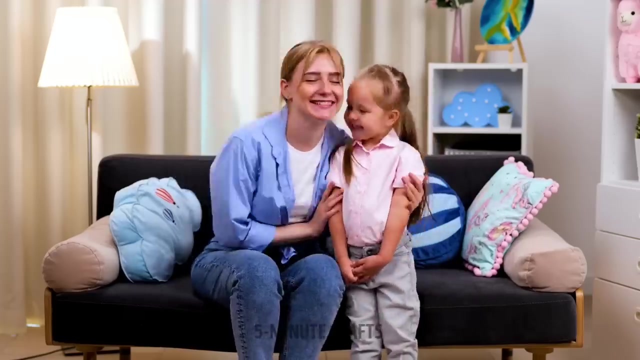 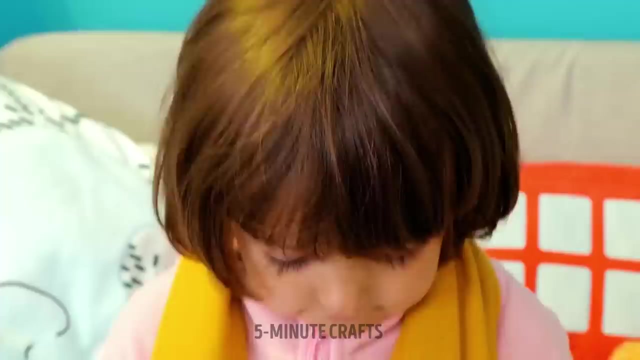 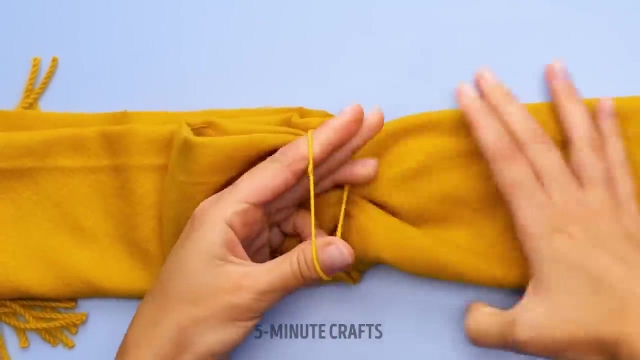 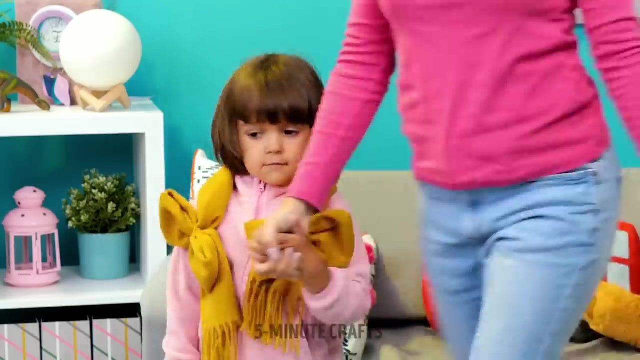 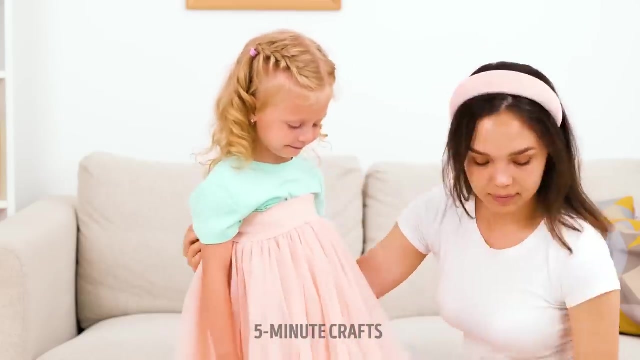 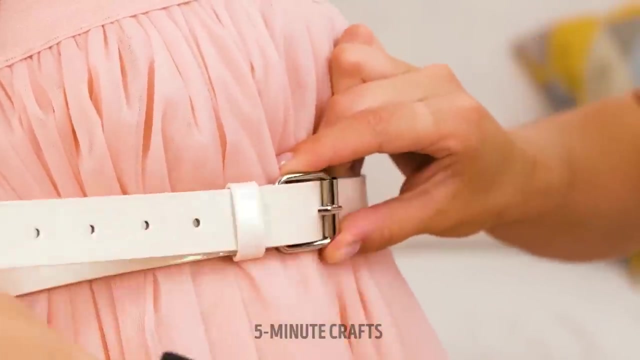 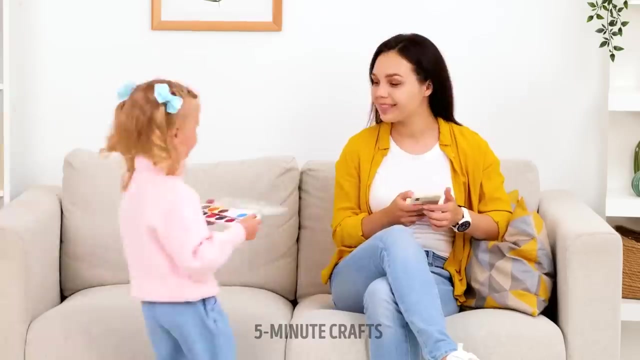 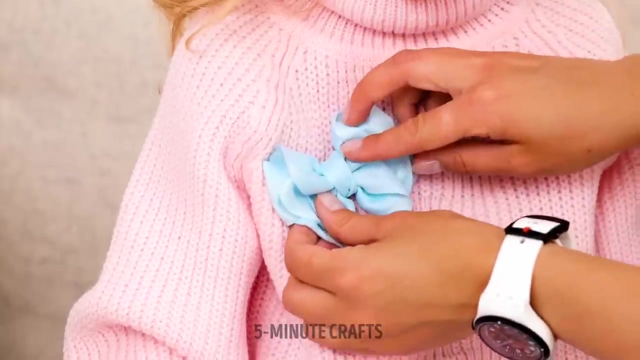 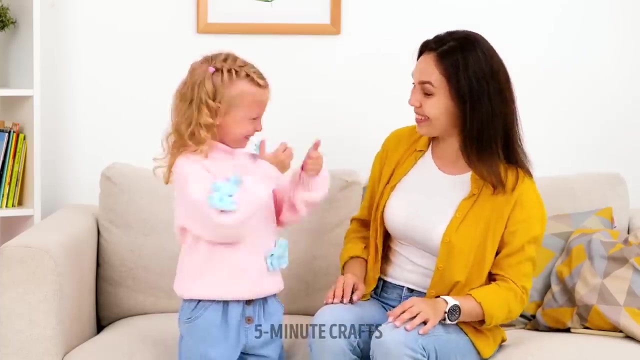 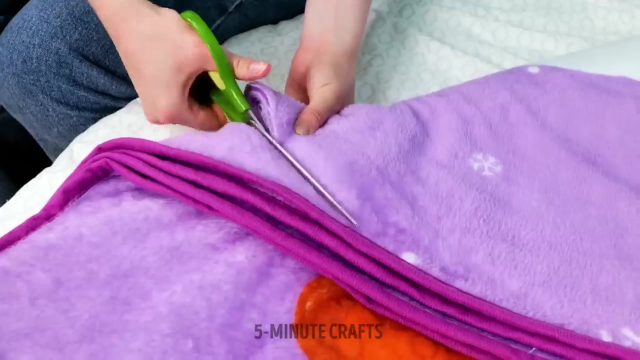 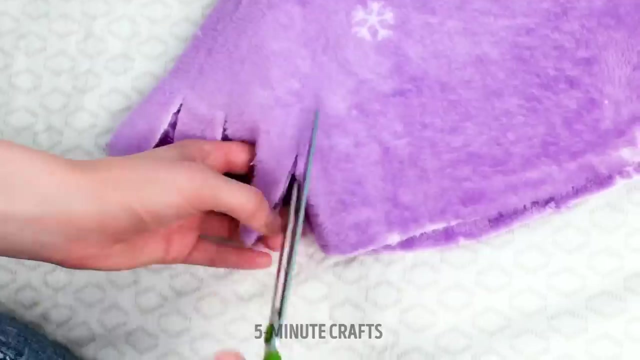 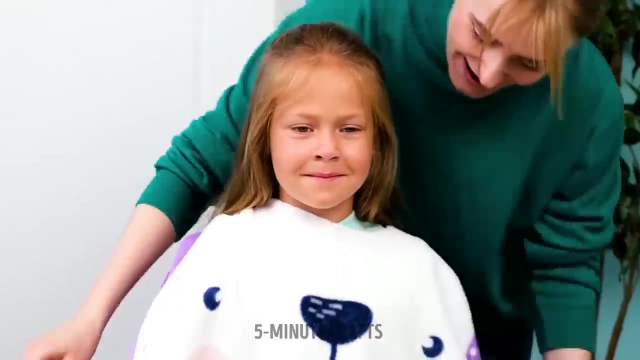 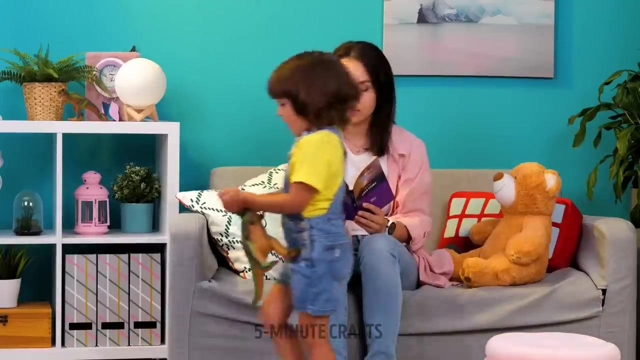 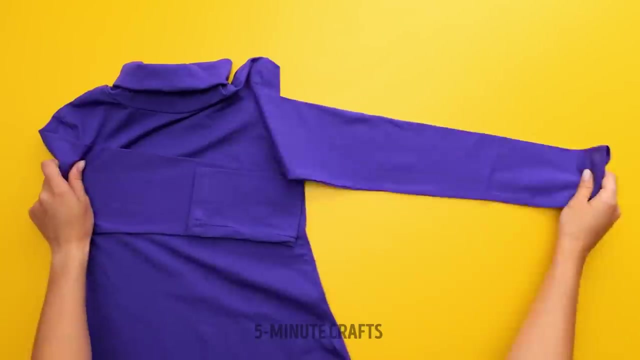 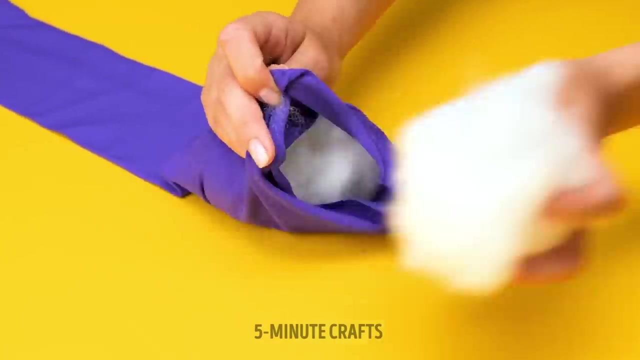 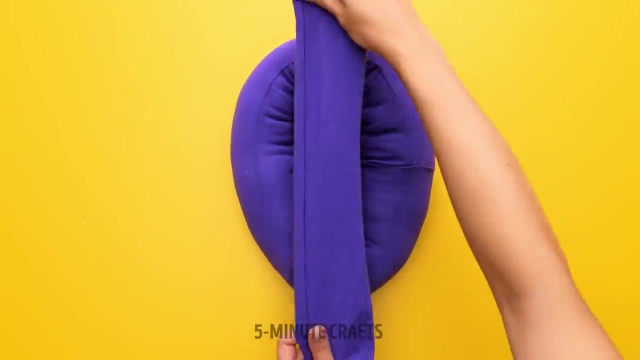 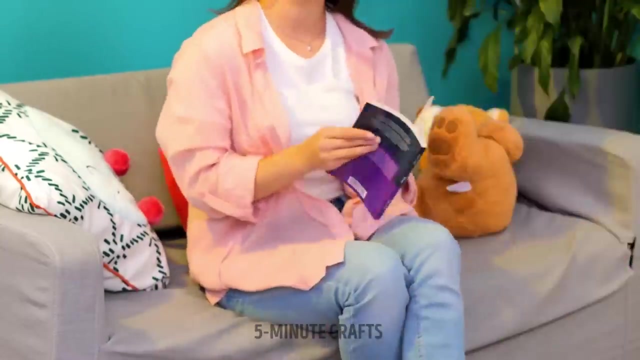 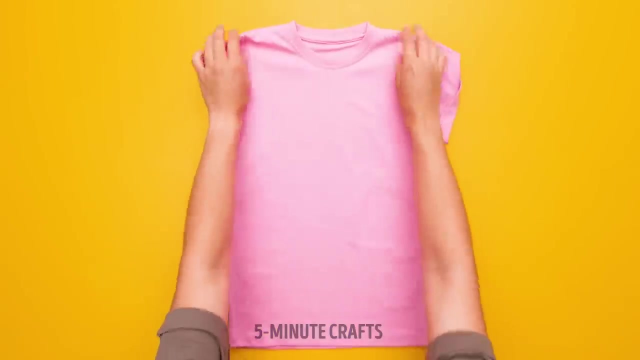 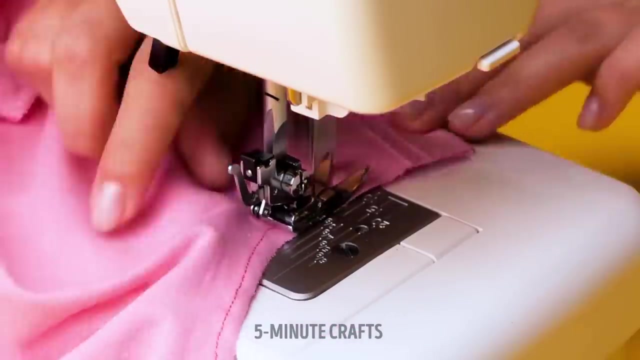 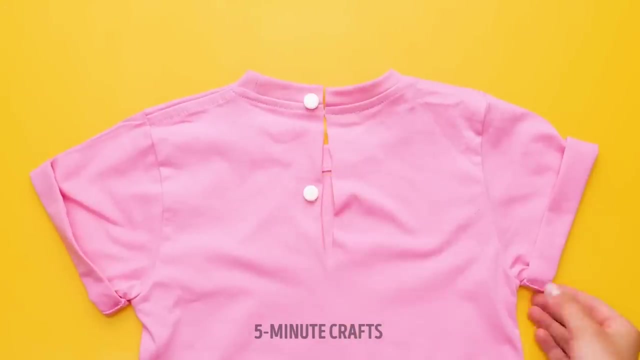 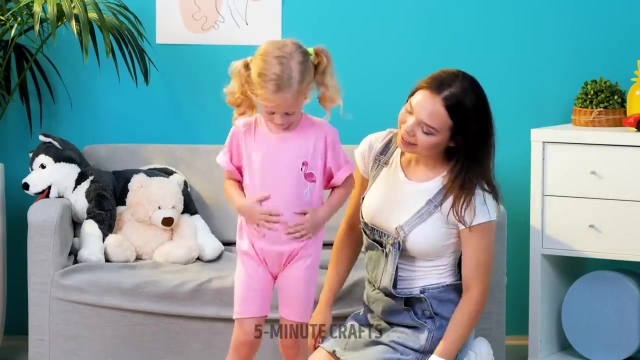 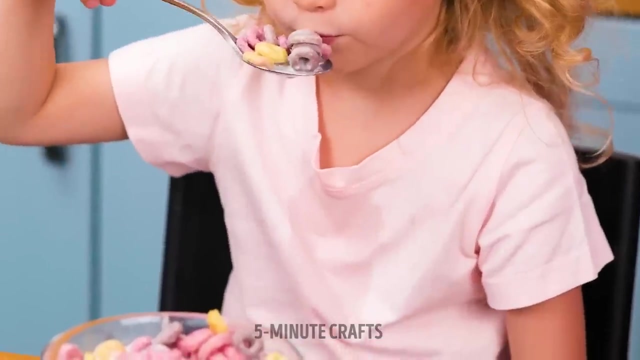 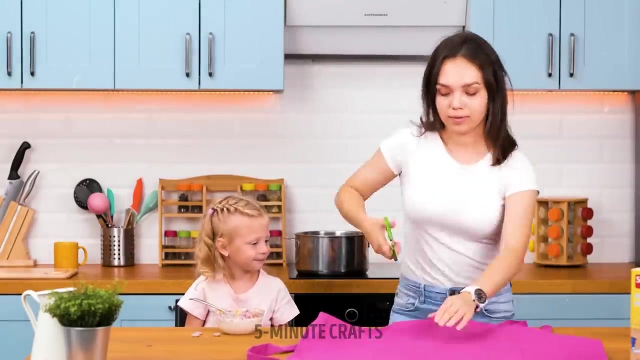 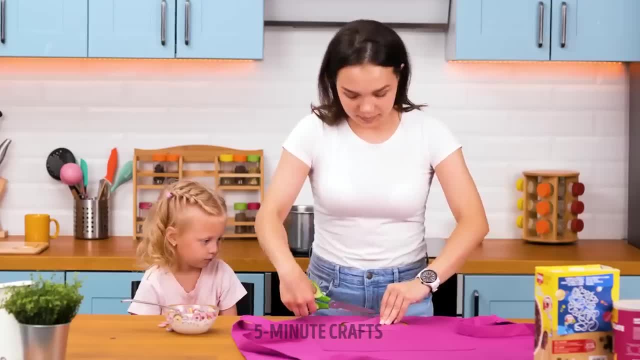 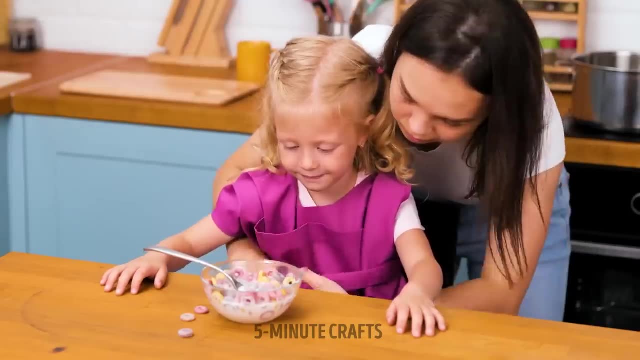 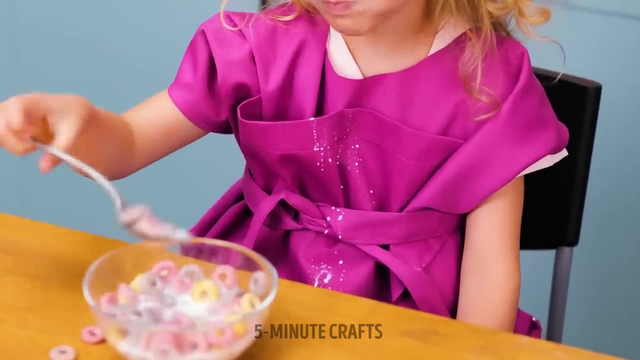 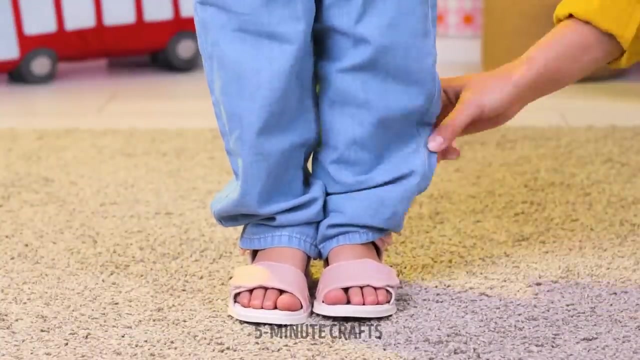 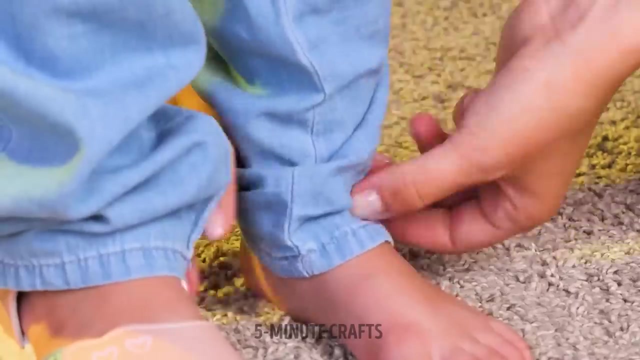 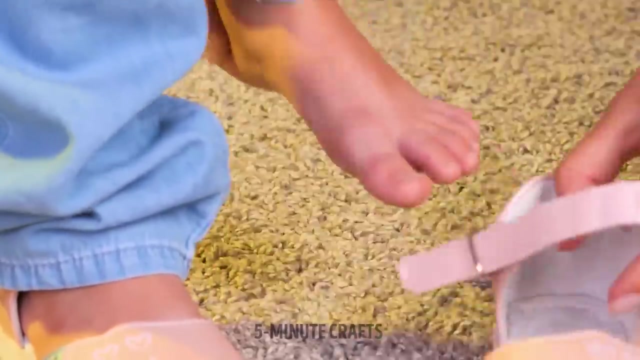 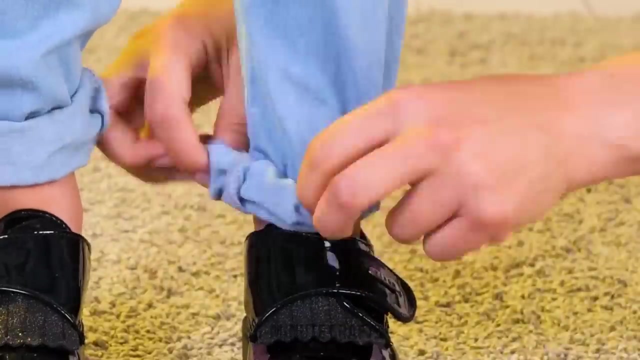 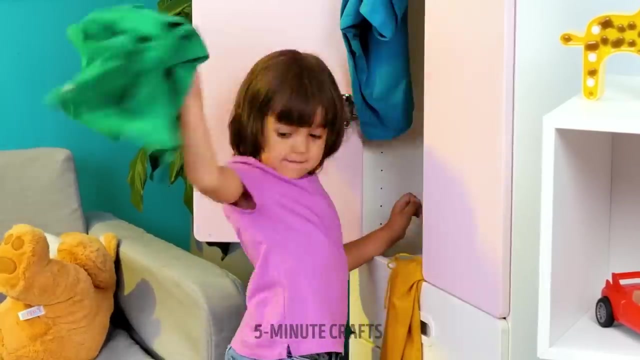 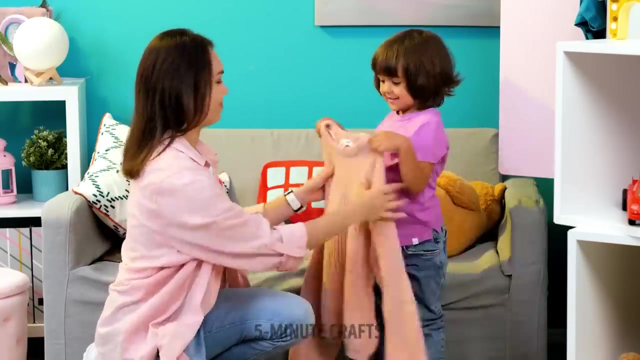 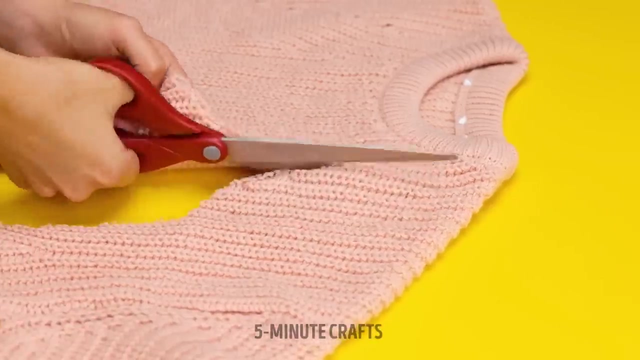 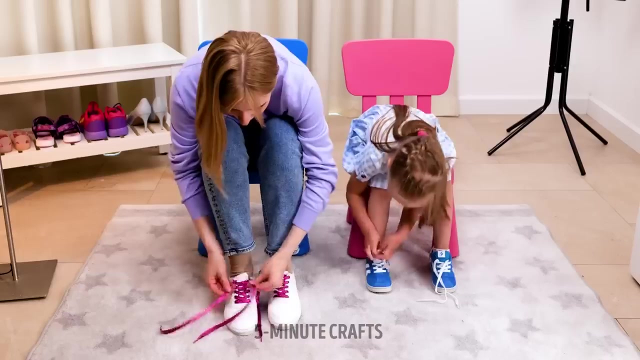 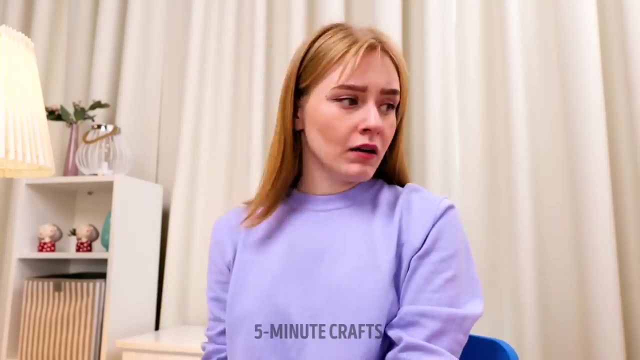 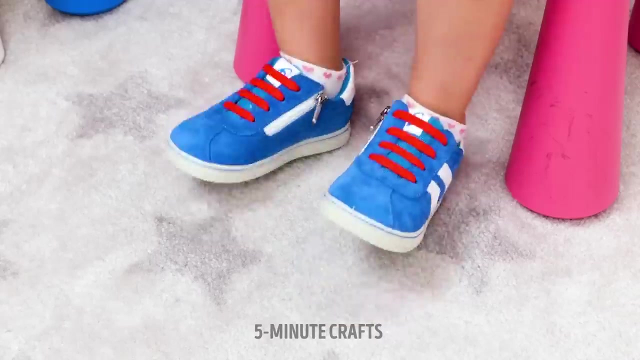 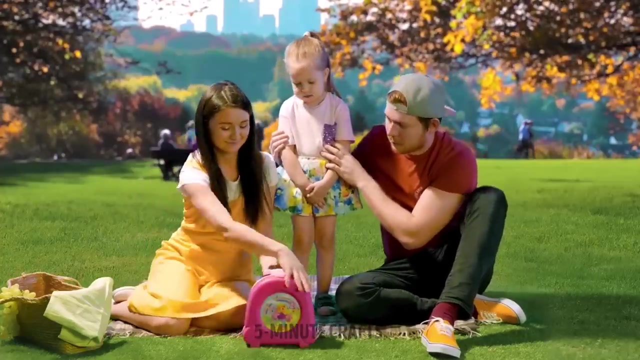 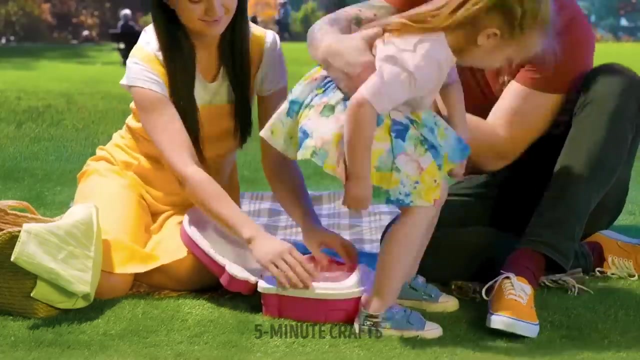 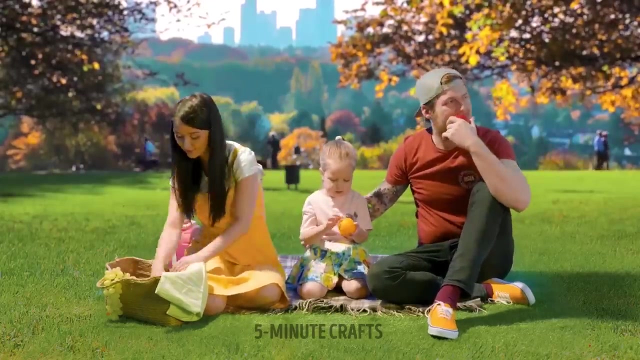 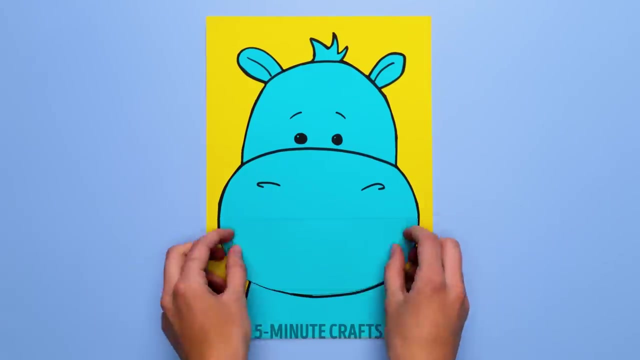 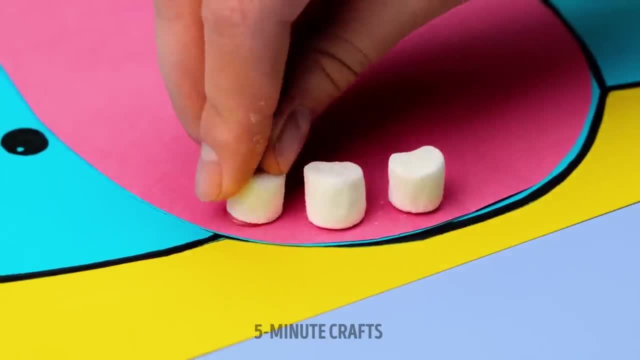 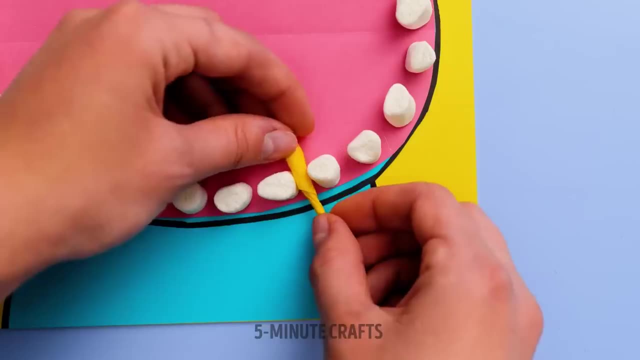 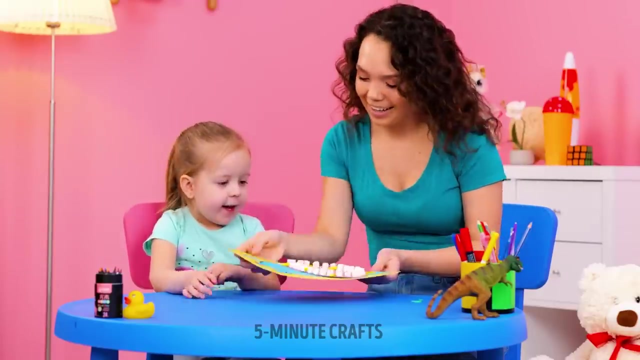 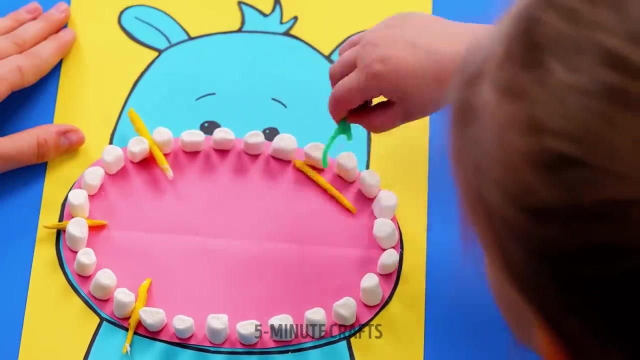 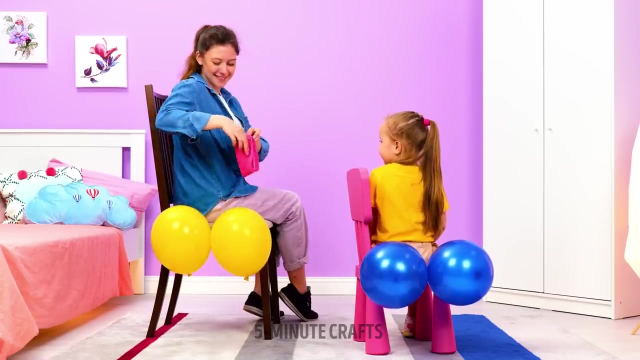 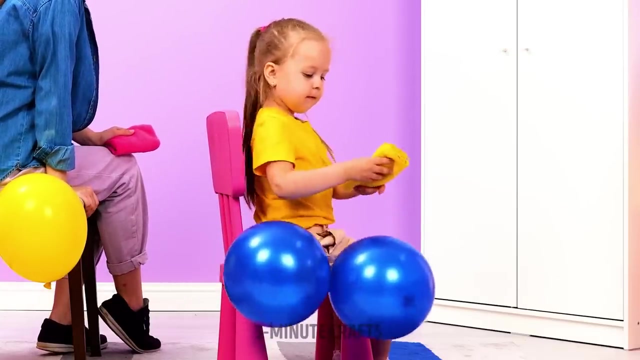 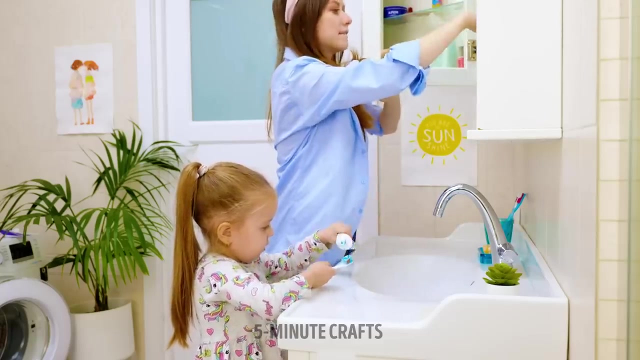 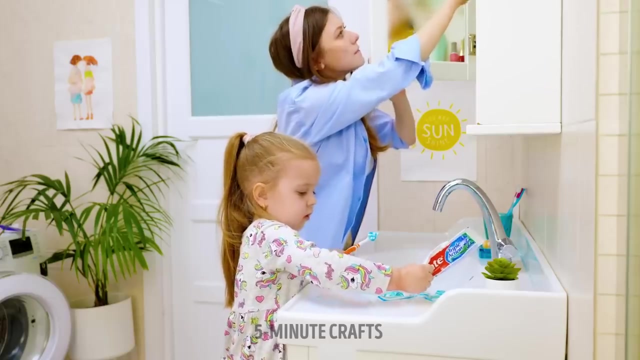 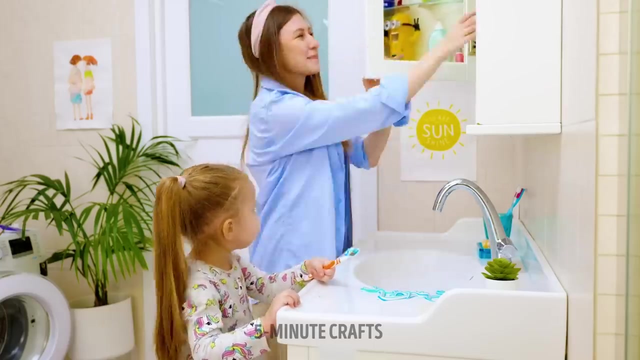 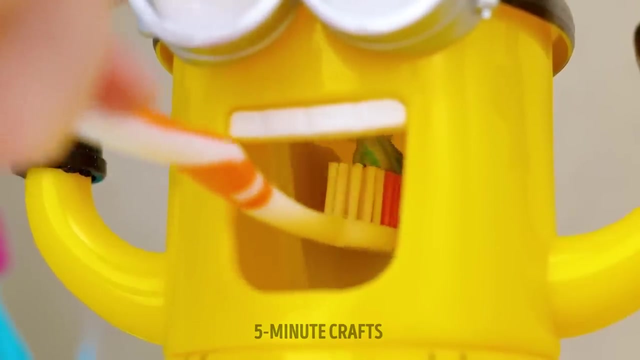 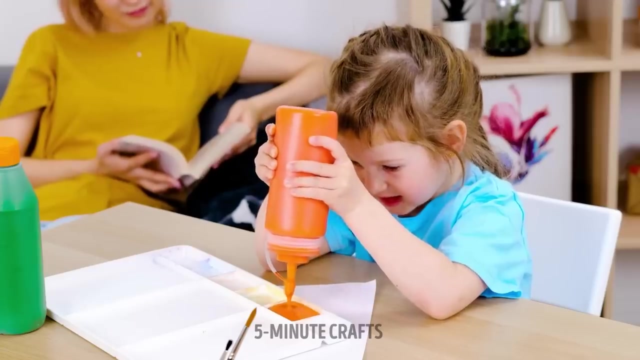 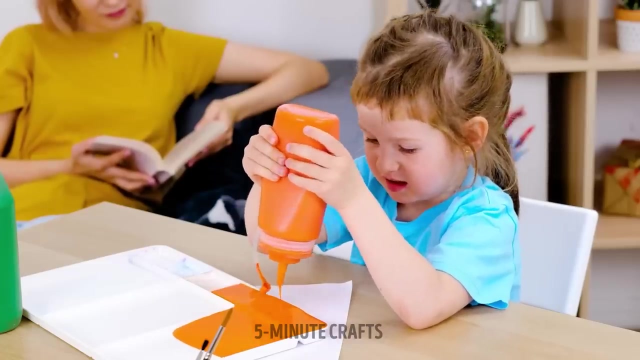 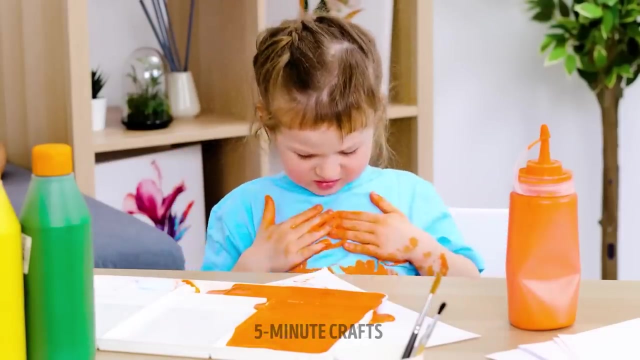 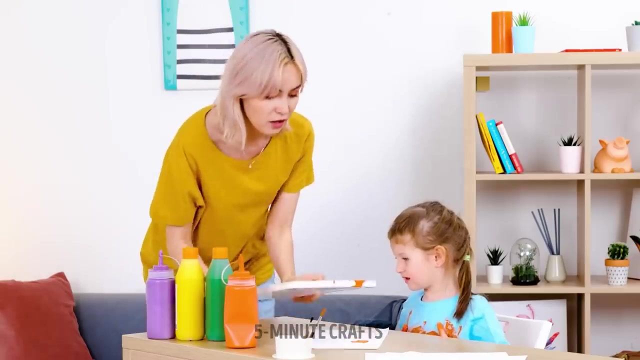 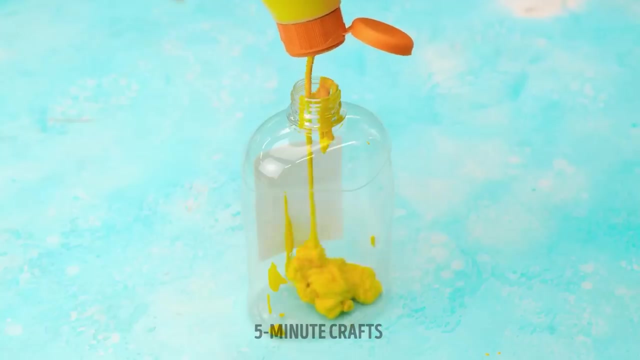 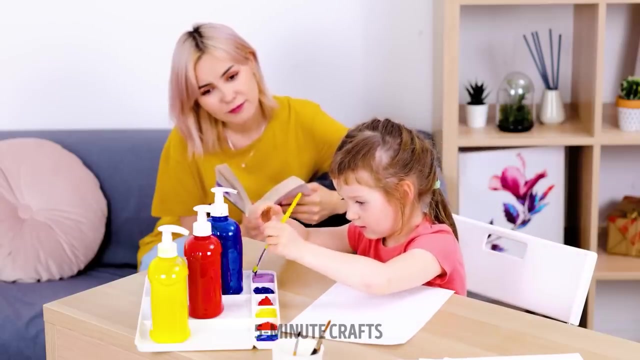 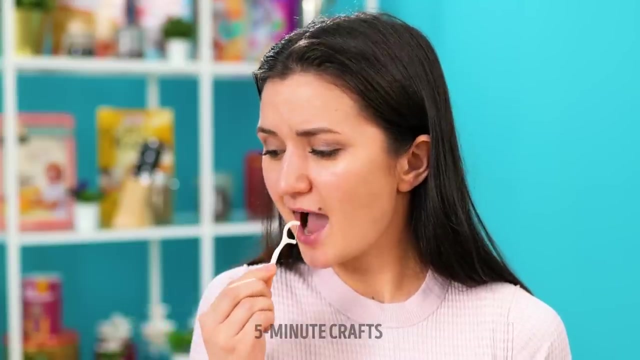 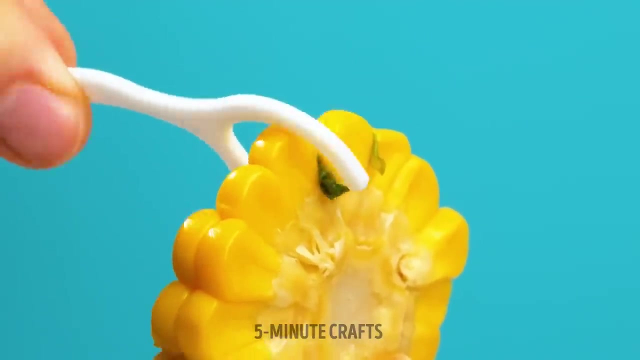 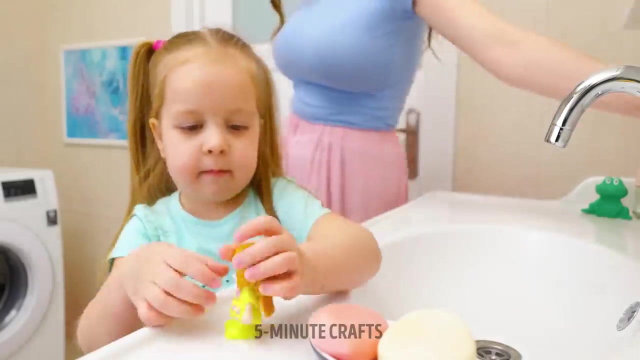 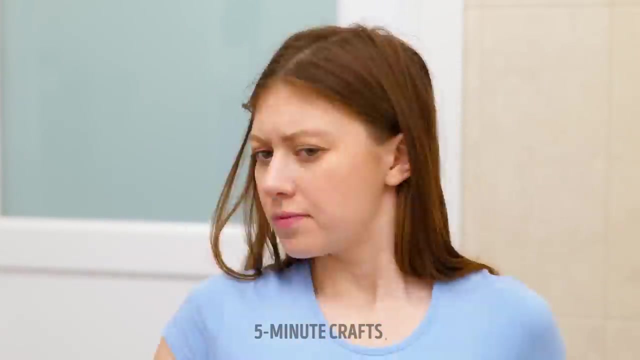 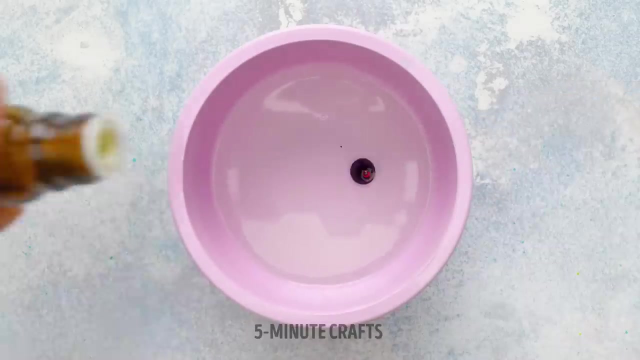 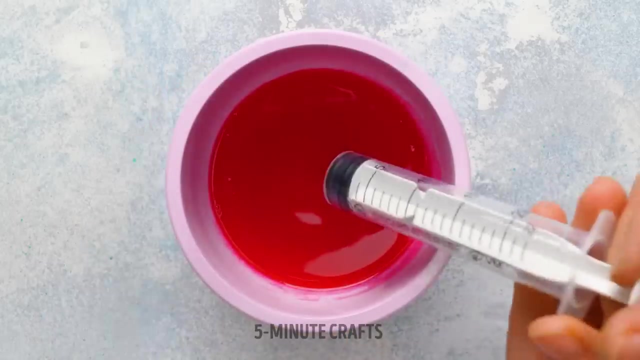 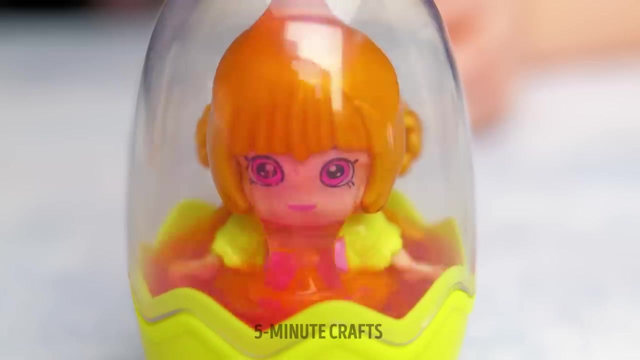 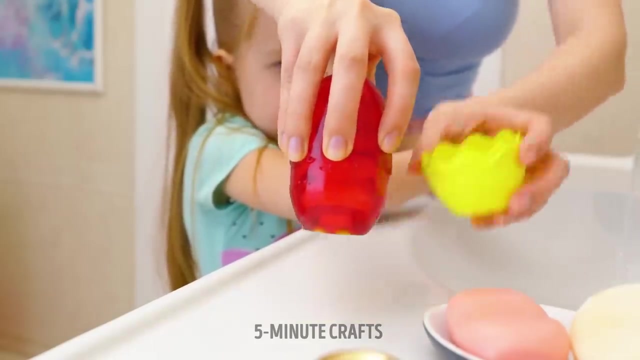 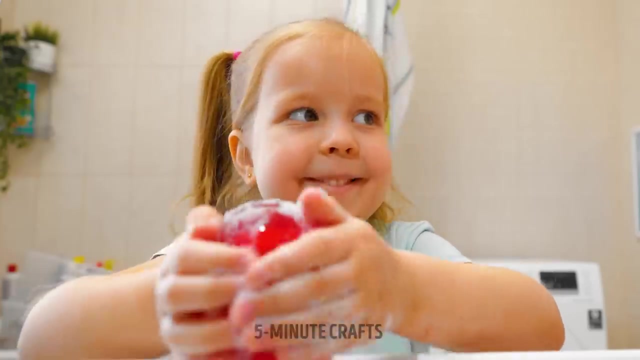 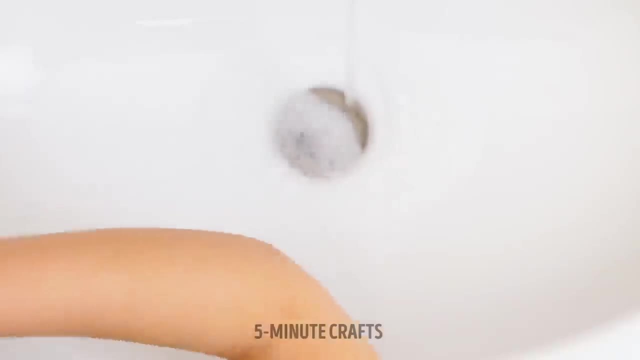 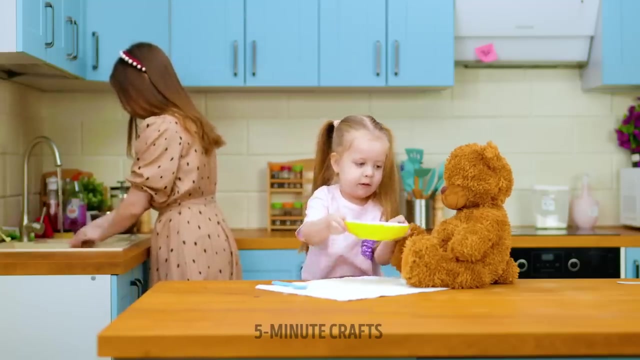 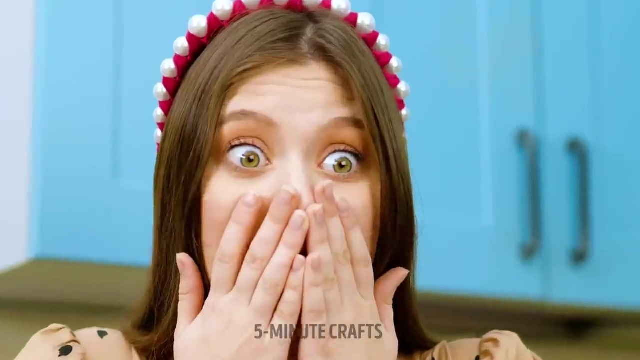 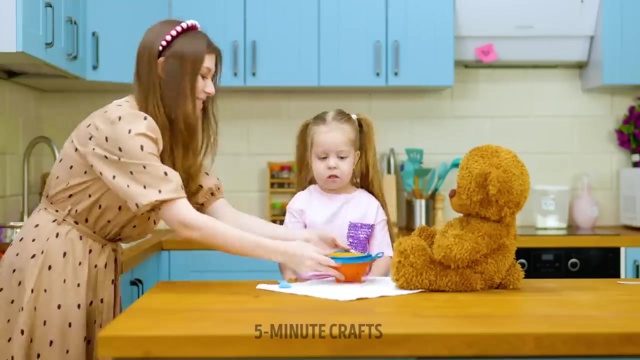 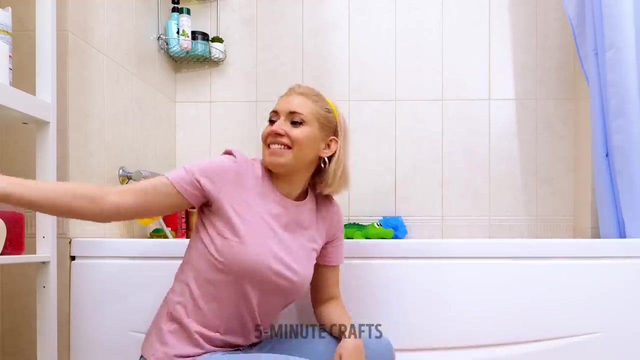 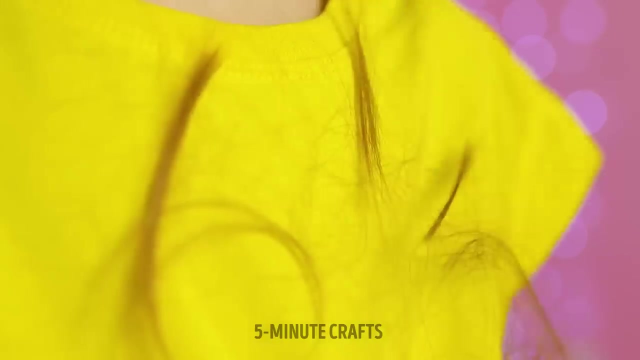 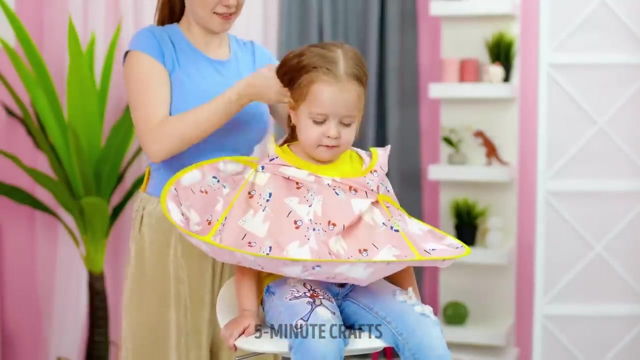 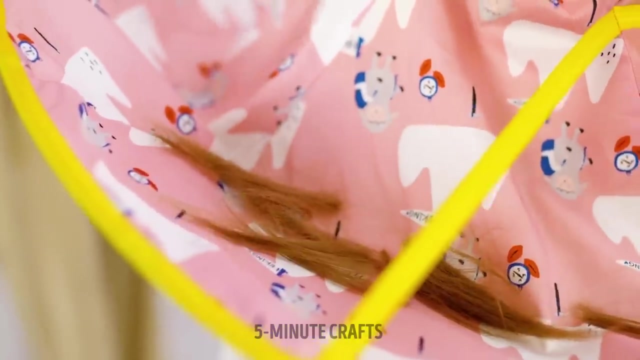 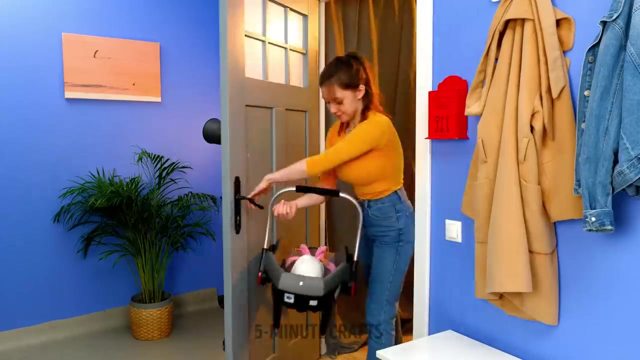 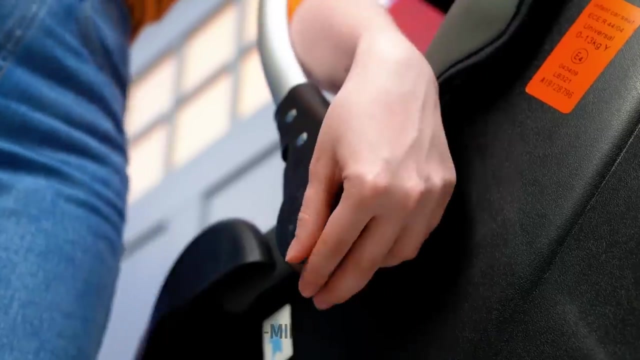 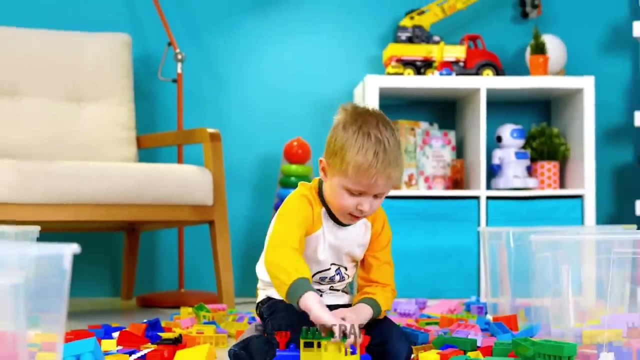 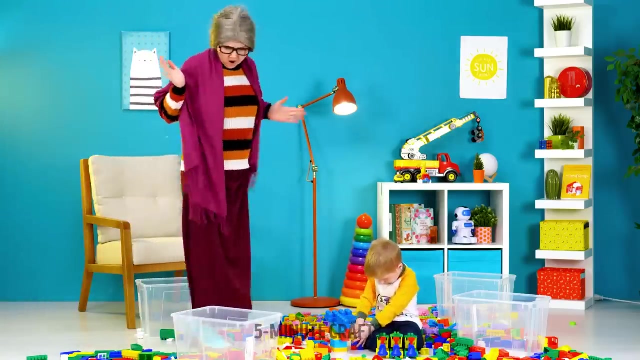 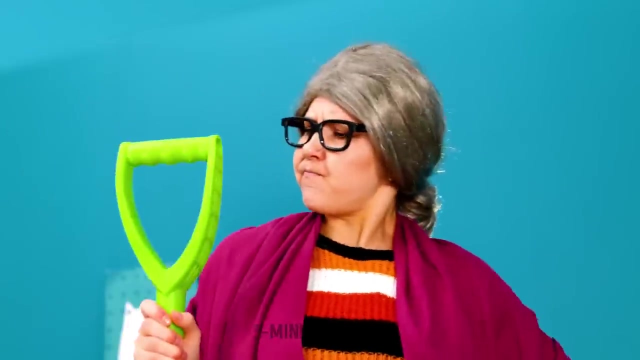 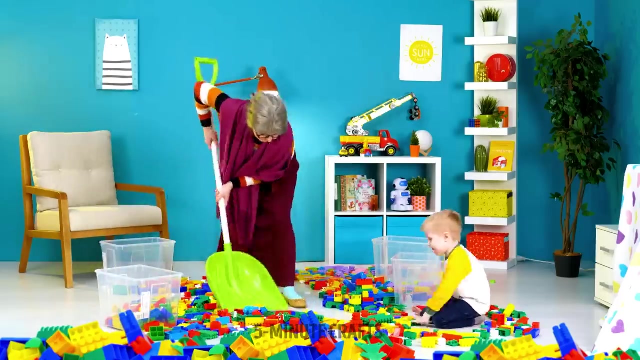 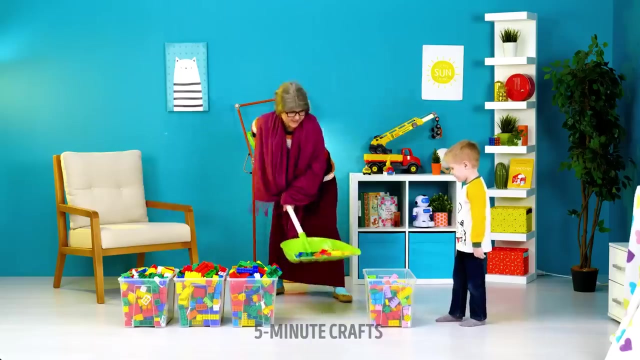 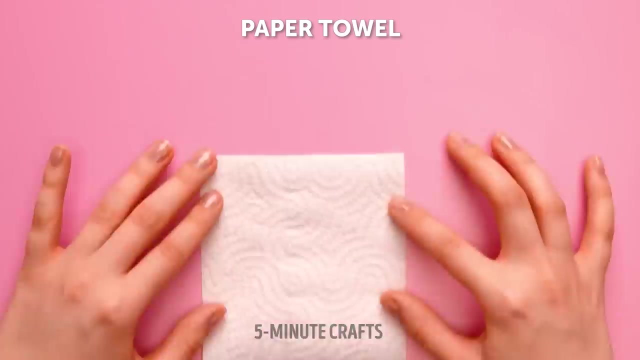 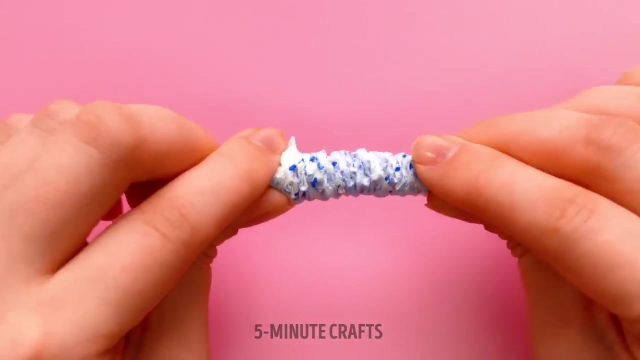 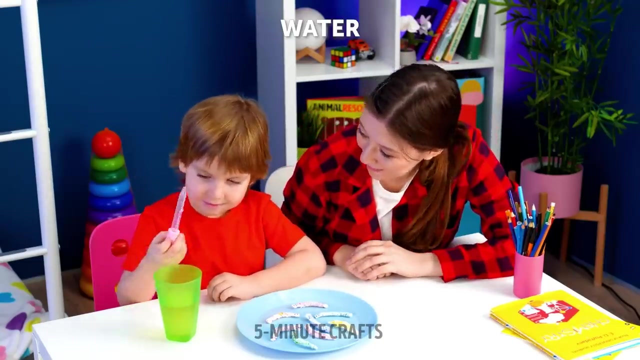 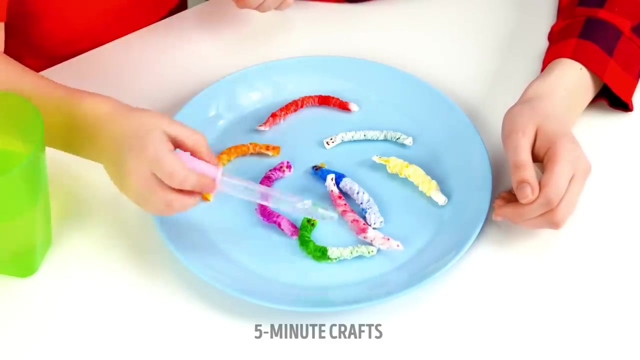 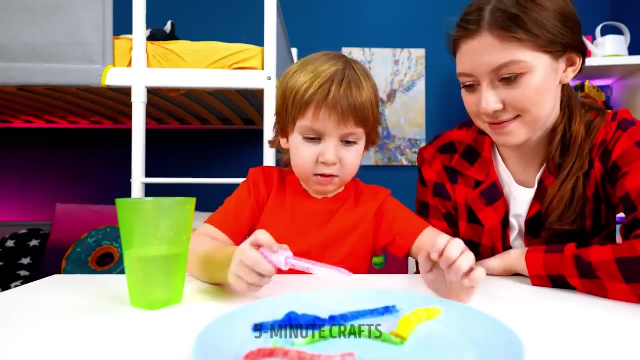 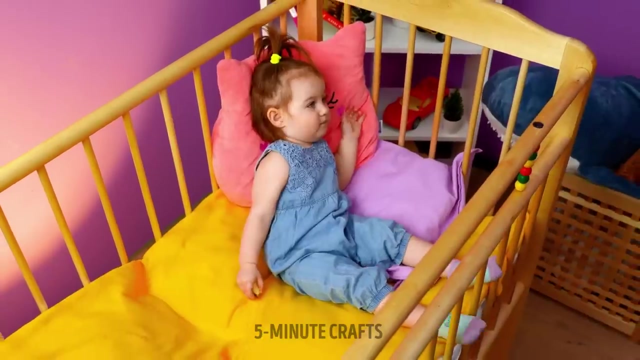 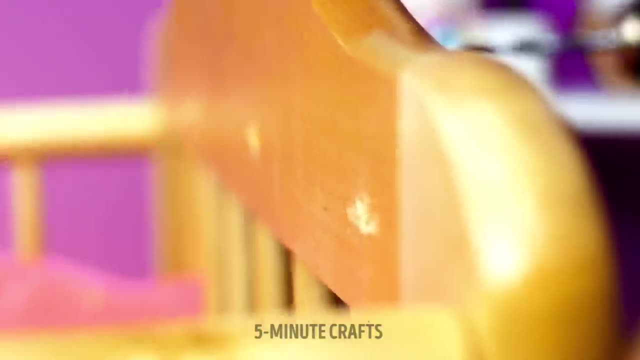 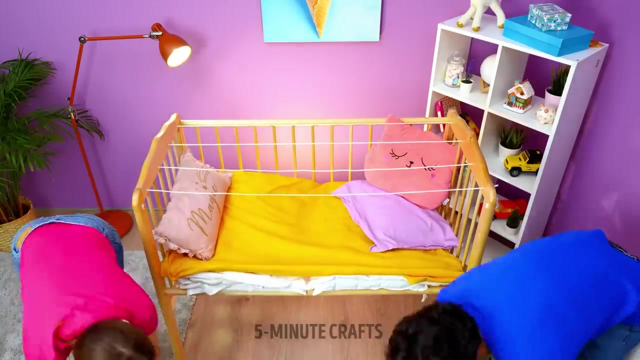 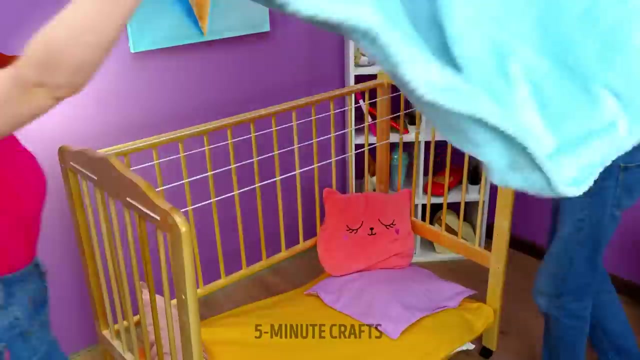 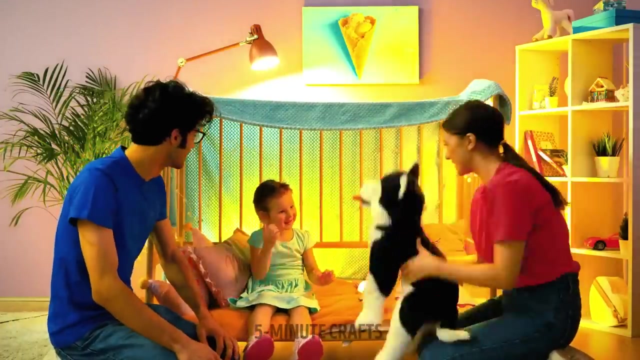 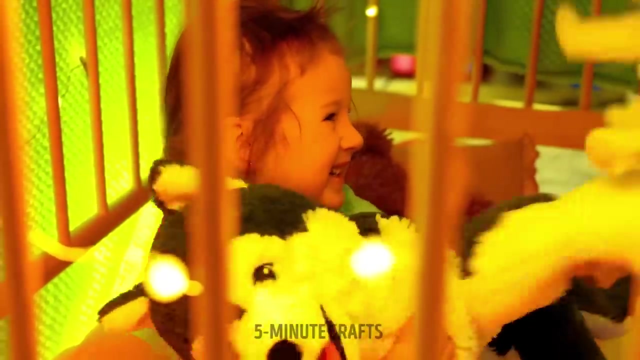 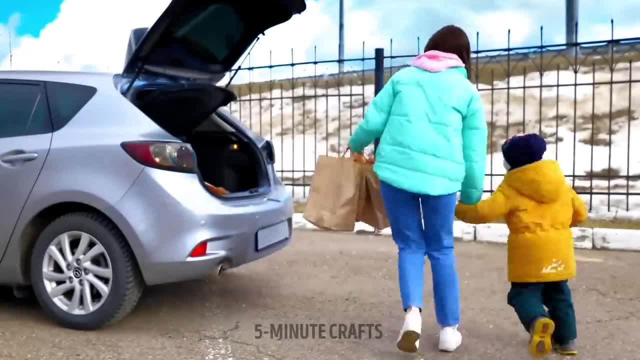 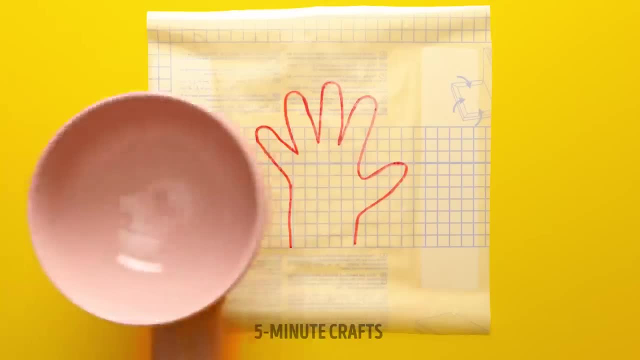 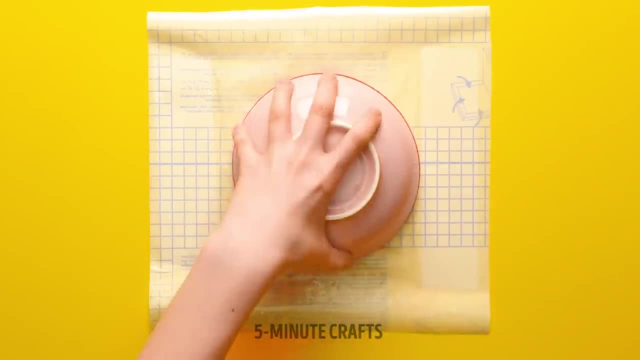 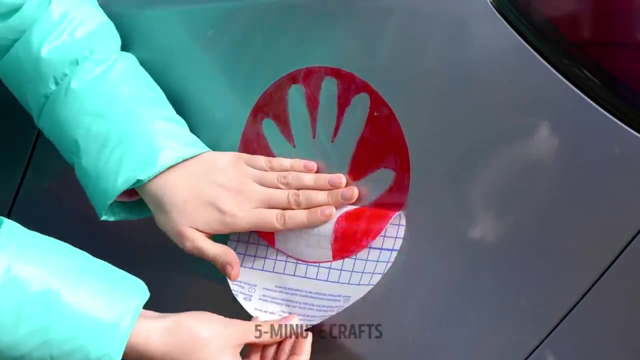 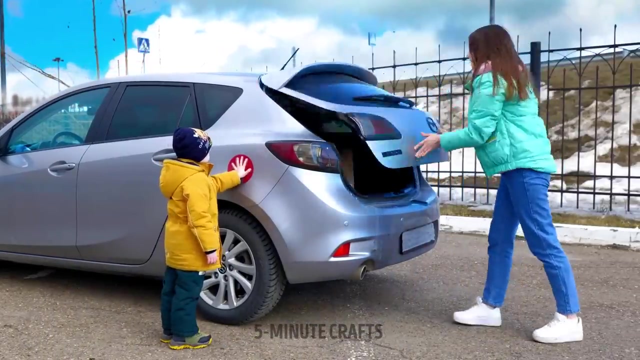 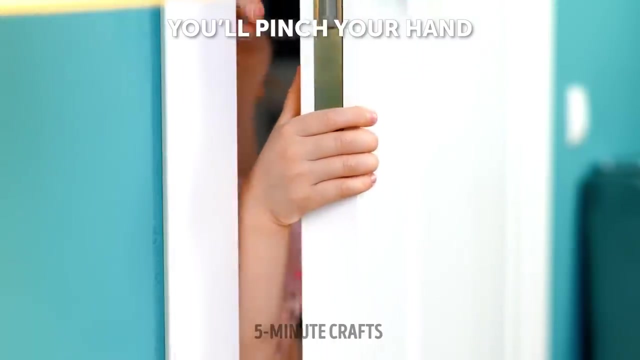 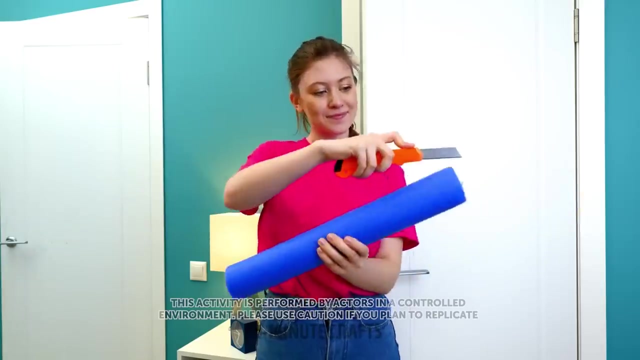 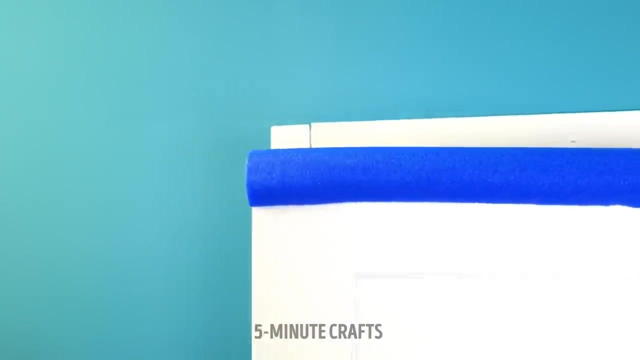 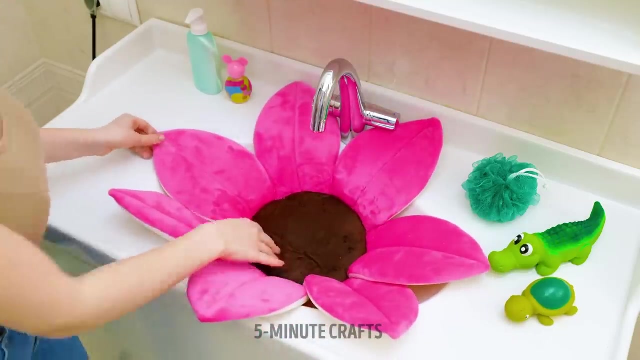 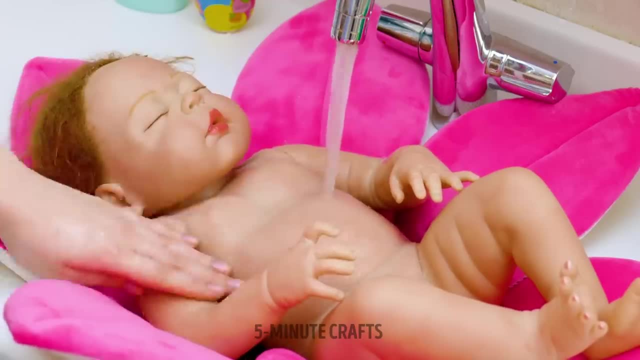 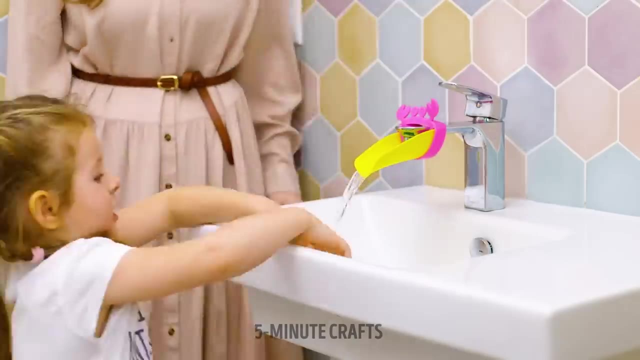 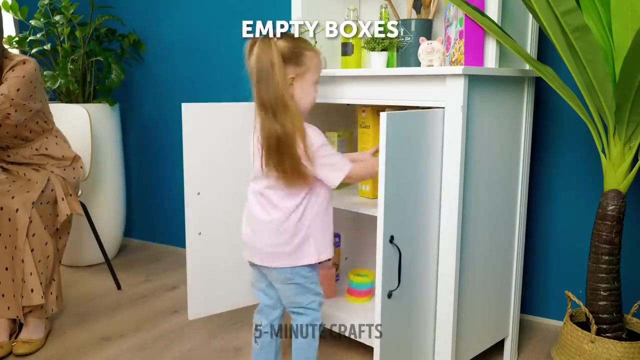 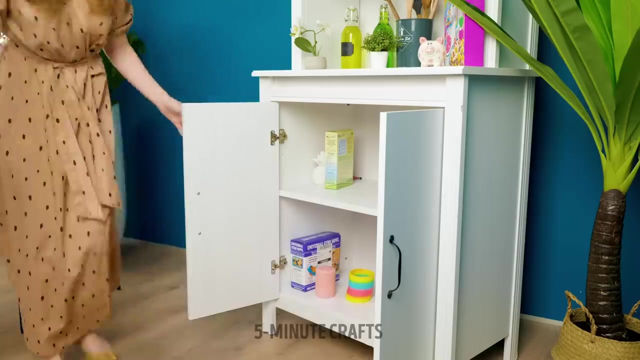 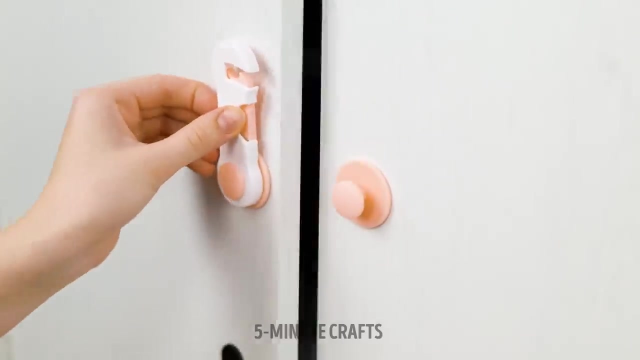 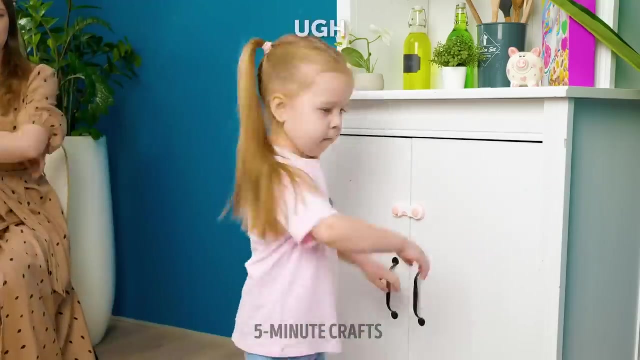 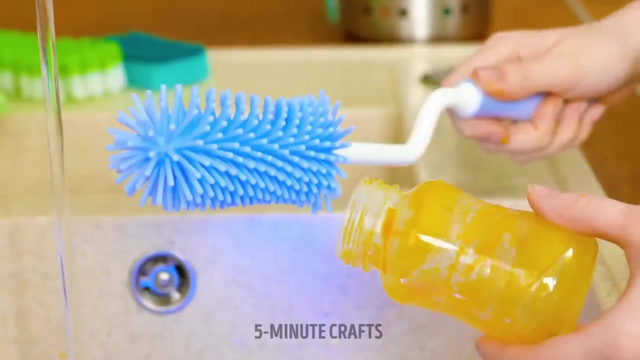 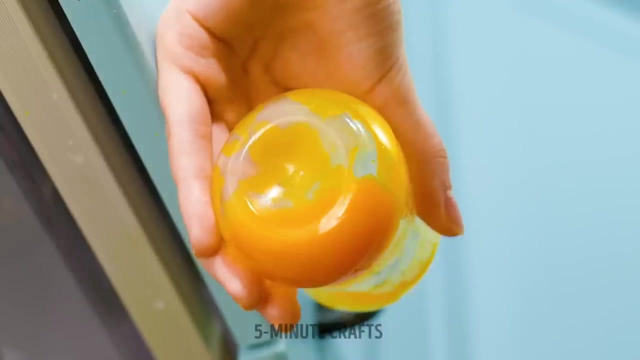 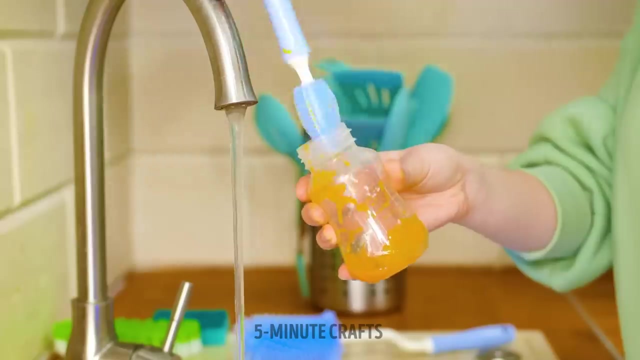 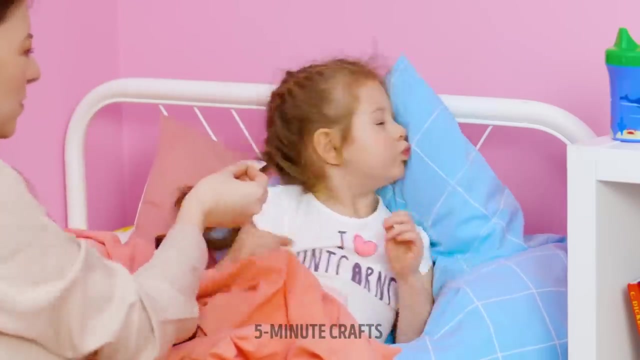 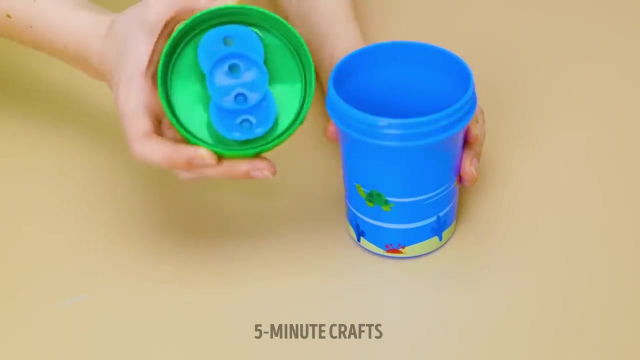 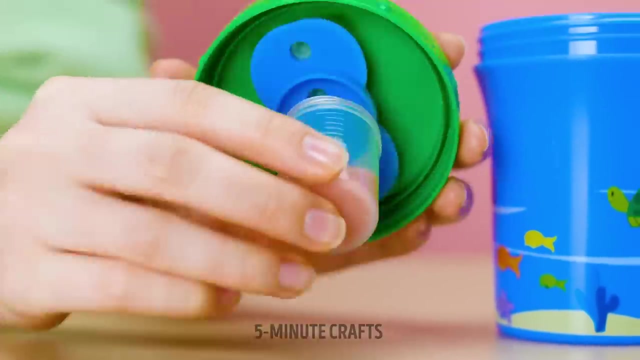 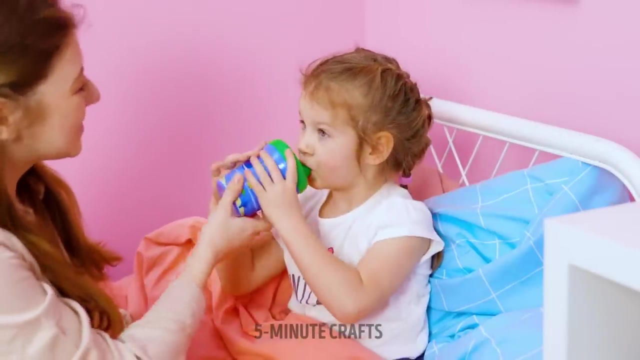 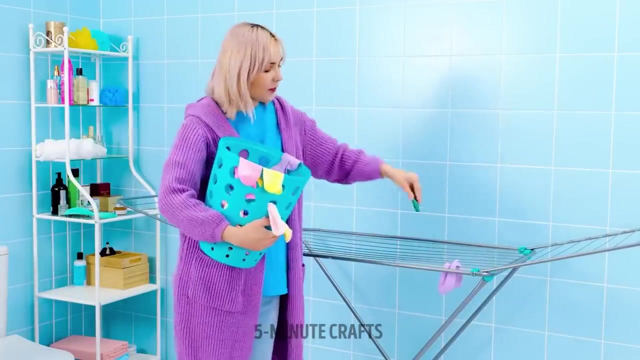 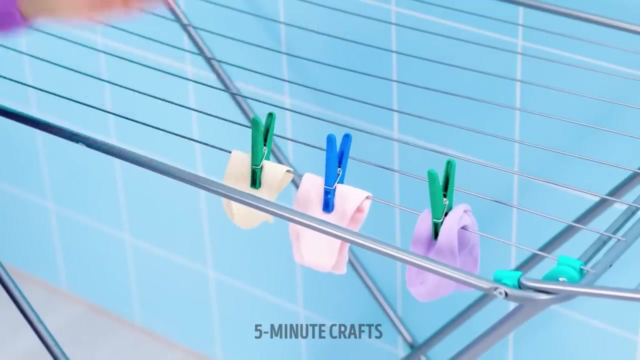 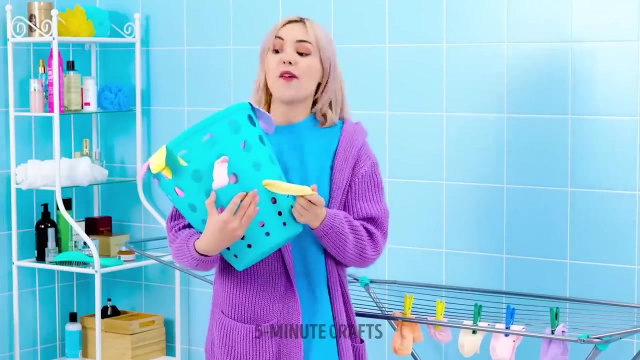 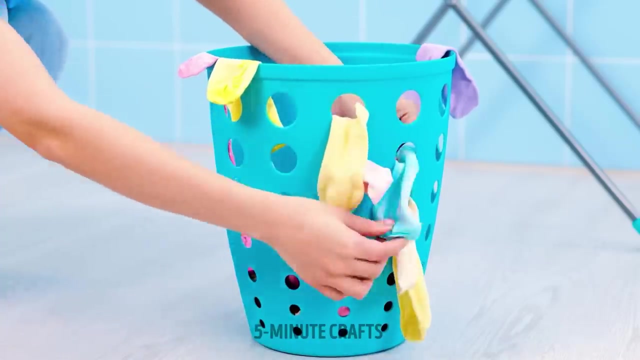 If you were looking for one hell of a ride, Just come and get it, baby, I'm all yours. If you were looking for one hell of a ride. If you were looking for one hell of a ride. If you were looking for one hell of a ride.